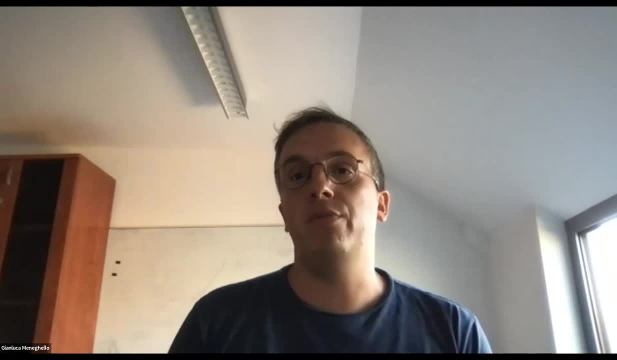 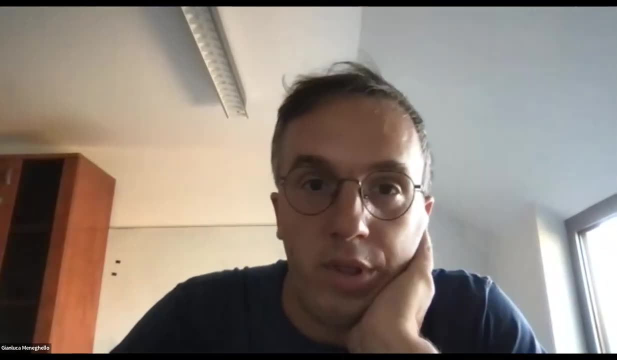 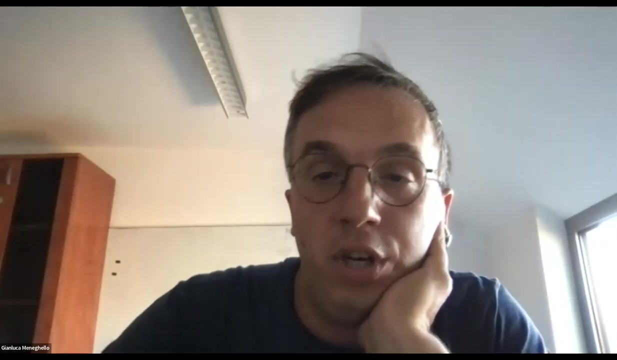 leaders from 18 federal agencies, departments and different offices, and with the goal to enhance collaborations on research within the Arctic region. This again is the Physico-Economic Community of Practice and our main aim is to coordinate research for physical geography. 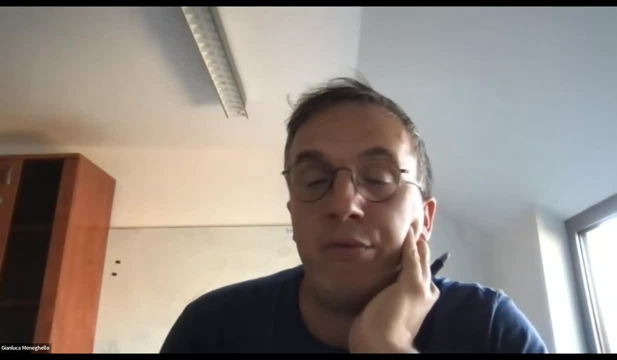 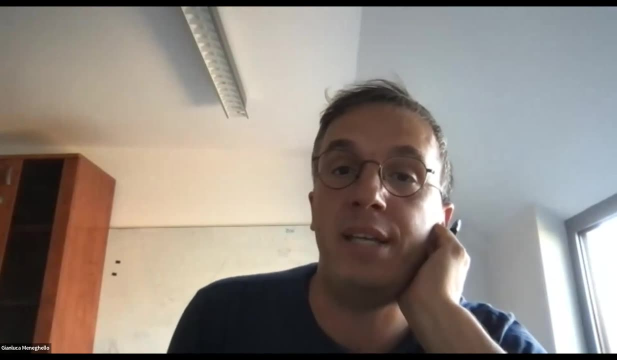 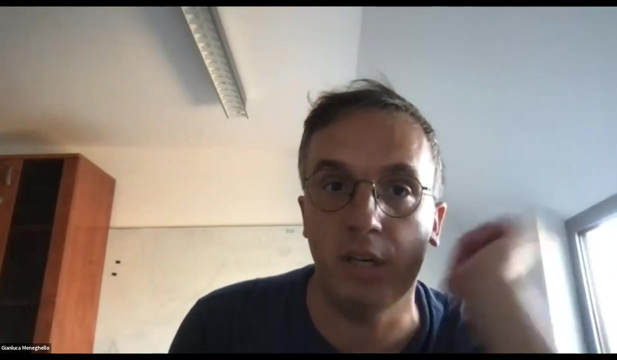 in the Arctic Ocean. The plan for today is to discuss how our community of practice can contribute to the success of the Biennial Implementation Plan. This is a plan that has been recently released. You can find it online on the IRPC website. There is a link on the. 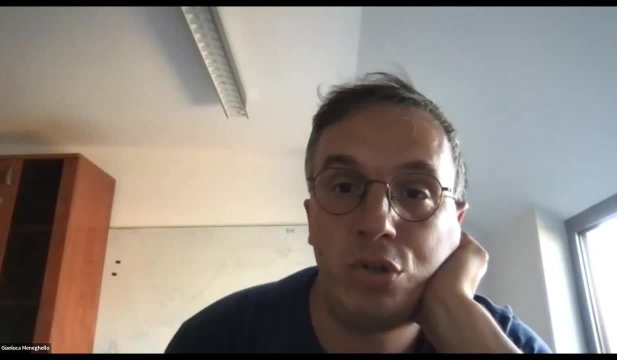 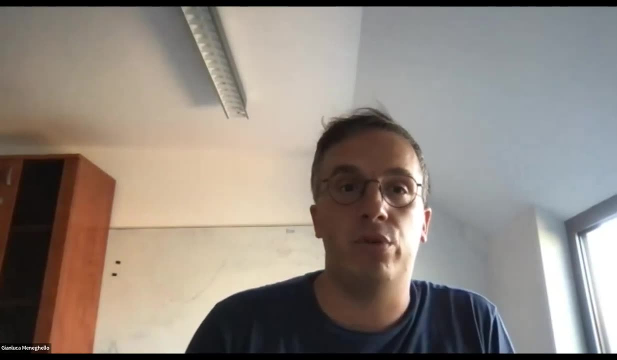 webpage And, in particular, today. what we will do is to hear from the program managers, and we would like to hear their opinions about what are the most important research directions for our field, for Arctic Physical Geography. Our first speaker will be Serena Stella. 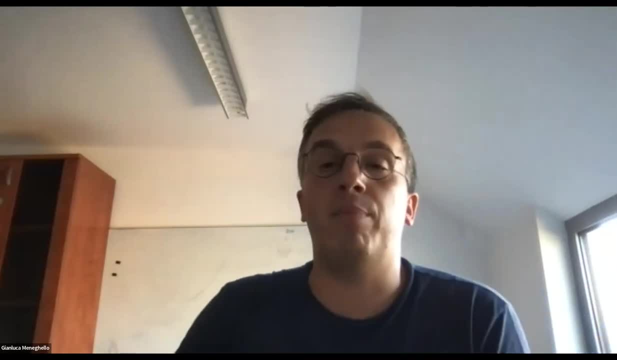 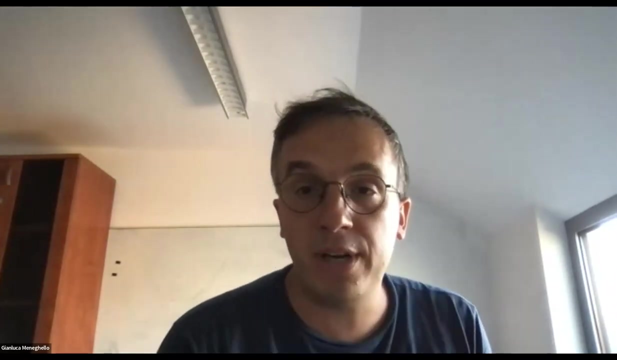 the IRPC Program Manager and we will hear about a brief overview of what the Biennial Implementation Plan is and what are the deliverables that our community can provide and contribute to. Then we will hear from three program managers In particular. we will hear 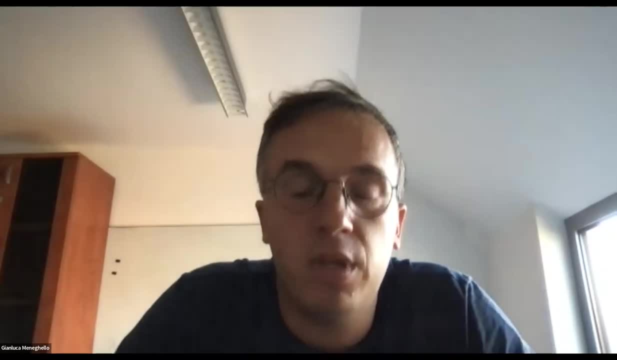 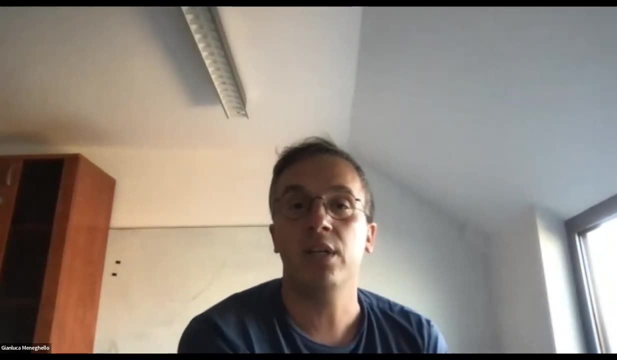 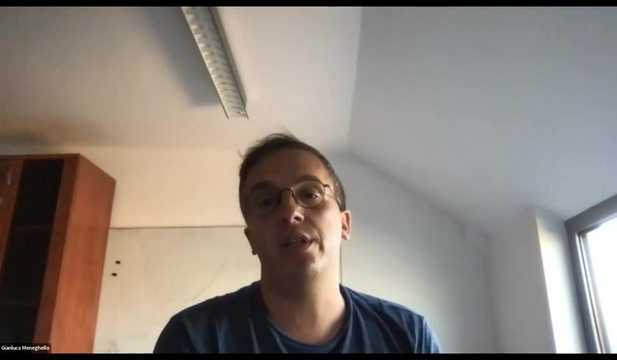 from Forsten Marcus from NASA- Thank you, Forsten. From Danielle Dickinson from the North Pacific Research Board- Thank you again, Danielle. And from Sandy Lucas from NOAA And, of course, thank you, Sandy, for joining us Again. the goal. what we would like to hear is about how. 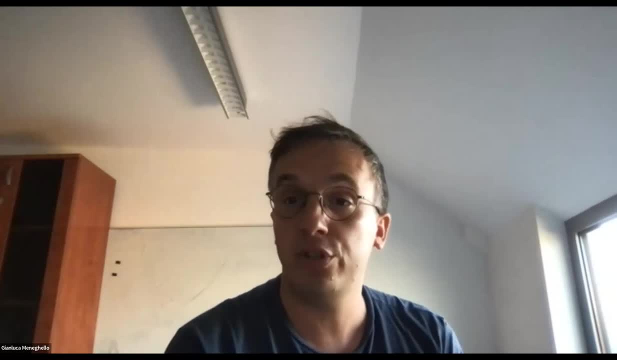 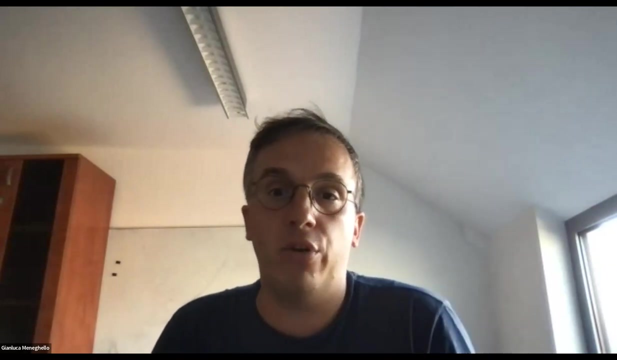 your program is planning to support the physical geography research and information you might have, but that is, of course, very welcome, And, after hearing from you, what we would like to do is to invite everybody from the community to express their ideas on how we could best contribute to. 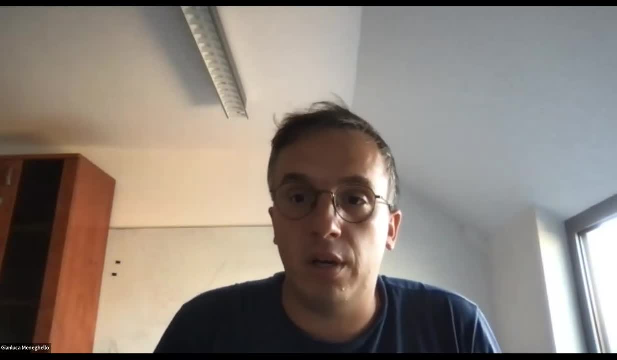 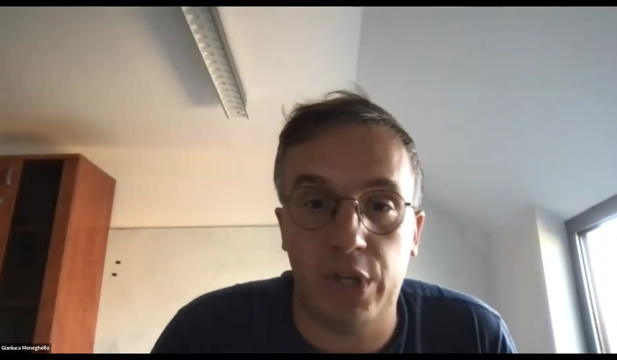 the plan. As a reminder, the goal of Physical Geography Community, the contribution of the physical geography community can give to the plan, is about Arctic system interactions, which is our main point, but the main priority area, And we would like to contribute to the fundamental activities, what are called data management. 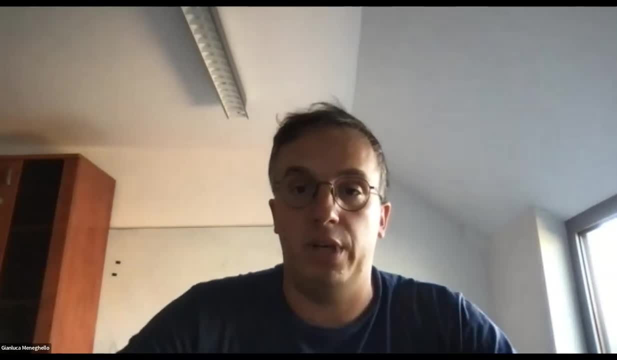 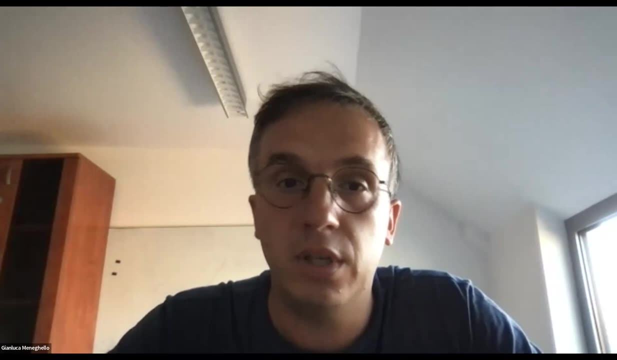 as well as monitoring, observing, modeling and prediction of the Arctic on the Arctic Ocean. I think we can start with, Serena, If you're unmuted, I don't know. Yep, I have some slides to share as well. Thank you very much. 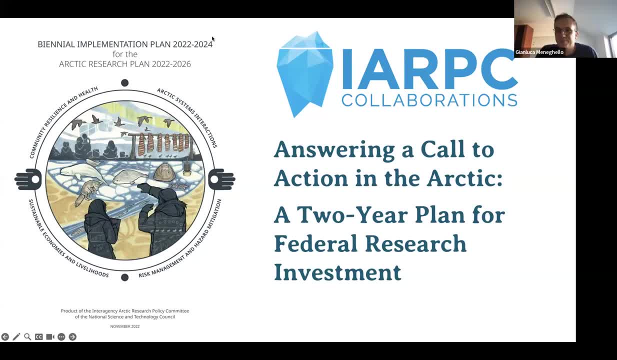 Can everyone see my screen? okay, That's great, Thank you, Yeah, Okay, Well, hi everybody. Thanks for the intro. My name is Serena Estala and I'm the Implementation Director for IARPC, And today I'm just going to provide. 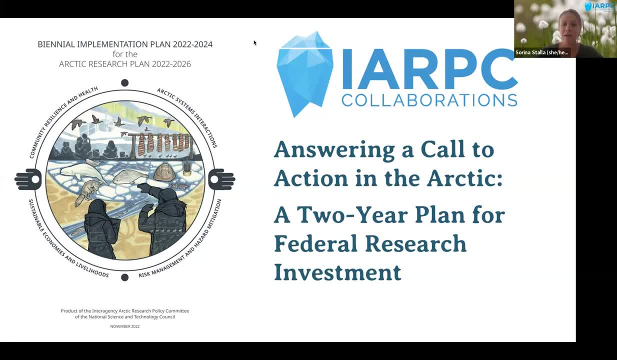 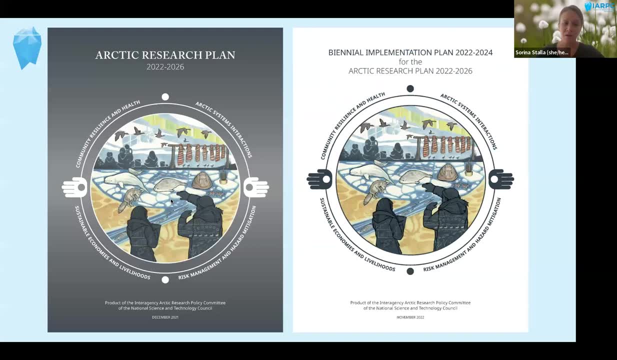 a short overview of the Biennial Implementation Plan and go over some of the areas that might be most relevant to the physical oceanography community of practice. And I'll start with some very general background which I think most of you are probably quite familiar with. 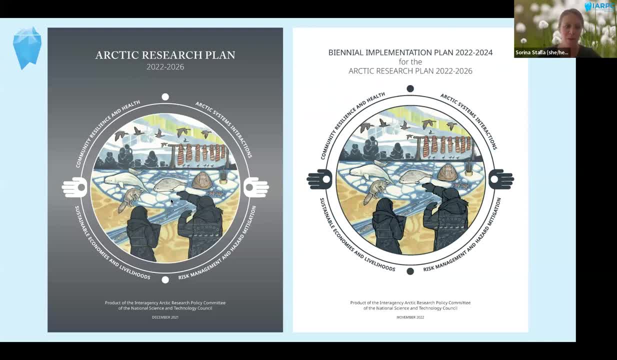 But just to take it back to the beginning, in December 2021, the White House Office of Science and Technology Policy released the IARPC Arctic Research Point, which is a plan to be implemented between 2022 and 2026.. And many of you participated in this. 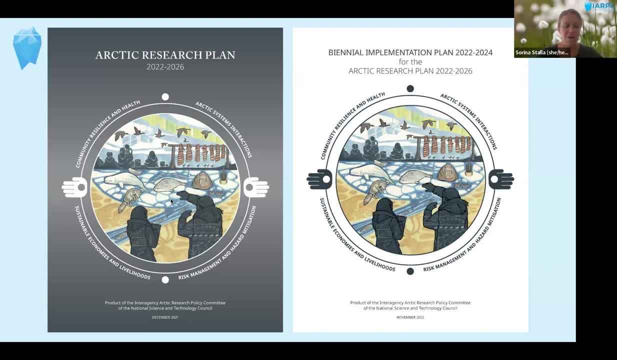 plan development effort. so we're very grateful for that and for your continued engagement. And the Arctic Research Plan was written as a high-level research strategy to address emerging research questions about the Arctic And it presents a research framework with thematic goals that kind of outlines a vision for federal agencies to address these emerging research. 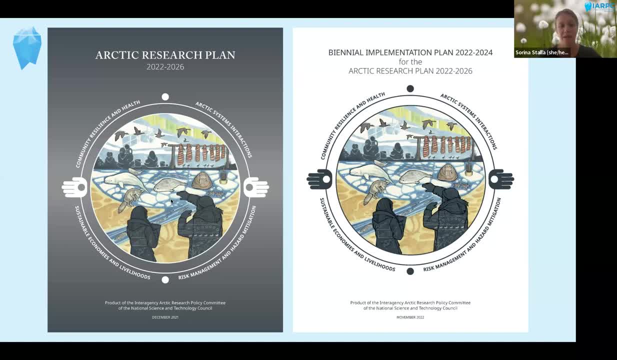 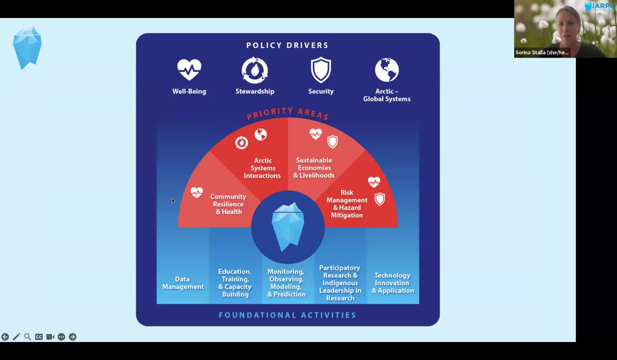 questions. And then research plan itself is implemented through biennial implementation plans which outline very specific research actions and research objectives and deliverables. So we're currently implementing the first biennial implementation plan, which is going to be implemented through fall 2024.. And again, like you, you'll probably be familiar with this framework diagram. 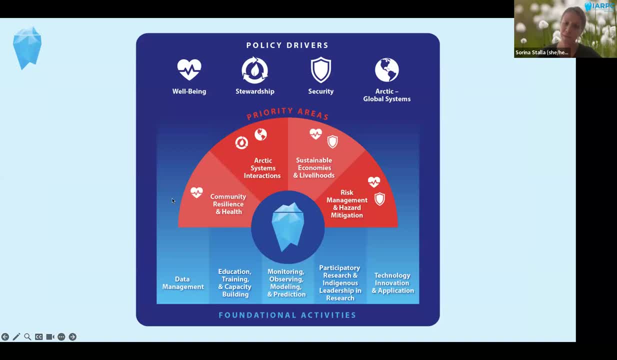 which illustrates the structure of the whole Arctic research plan. So, like I said, it's written as a high-level strategy that outlines research goals. These goals are linked to four priority areas, which are in the red fan: their community resilience and health. Arctic systems interactions. 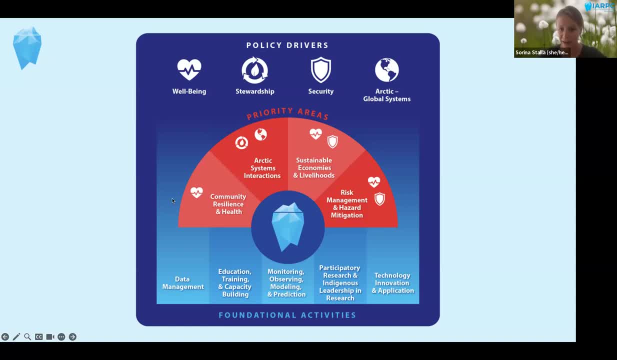 sustainable economies and livelihoods, and risk management and hazard mitigation. And the plan's also informed by five foundational activities, which are across the bottom in blue: their data management, education, training and capacity building, monitoring, observing, modeling and prediction. 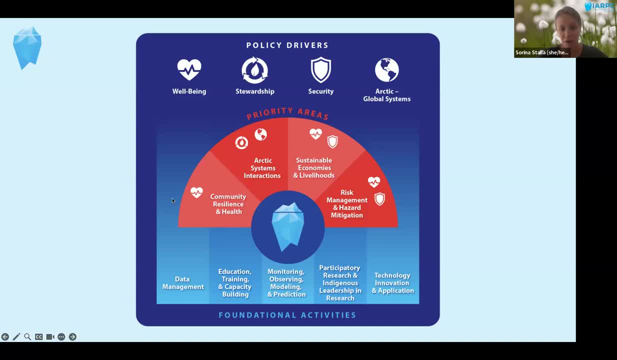 Participatory research and indigenous leadership in research and technology, innovation and application. So, building off of this framework in the Arctic research plan, the implementation plan includes objectives which are very specific: research, which are- they're pretty specific research actions that advance the goals of the Arctic research plan. And then it also includes: 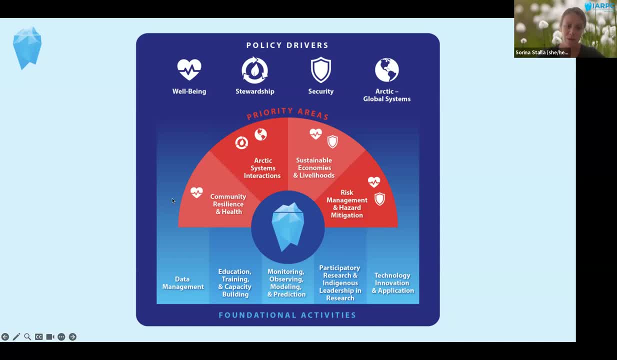 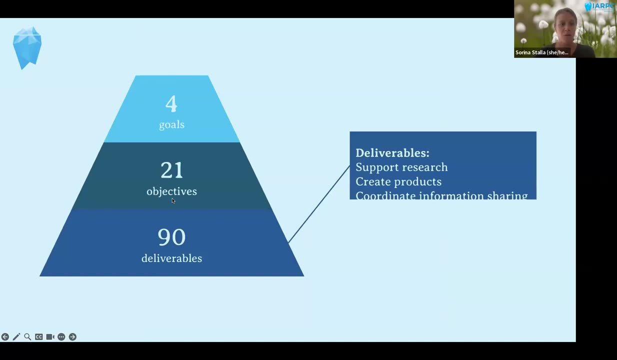 deliverables which are tangible, measurable and easily communicated, research products that demonstrates progress made towards achieving the Arctic research plan, And then it also includes objectives and goals, And then we make these products available to decision makers and partners across the Arctic. So we have in this biennial implementation plan that we're currently 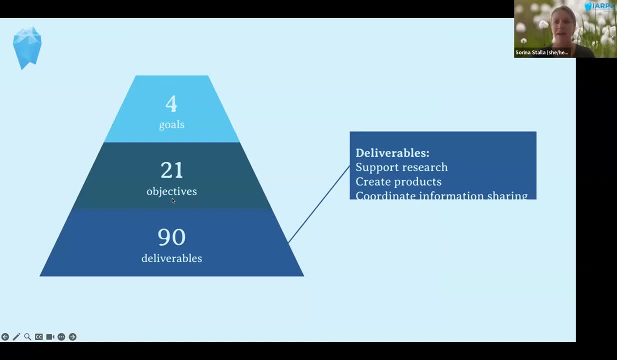 implementing. there are a total of 21 objectives. Each objective identifies deliverables, which again are research products, to be achieved in the next two years. This implementation plan has a total of 90 deliverables and they're centered around supporting research. So, for example, 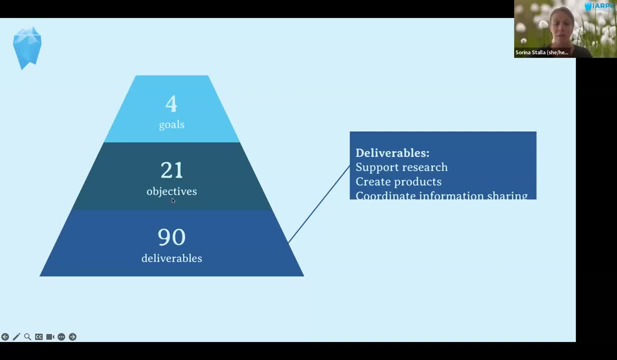 initiating funded projects with local partners creating products- So this could be a report or a synthesis or a tool- and coordinating information sharing. So, for example, this could be in the form of team meetings or workshops. So now, that's sort of the more general overview, And now I'll 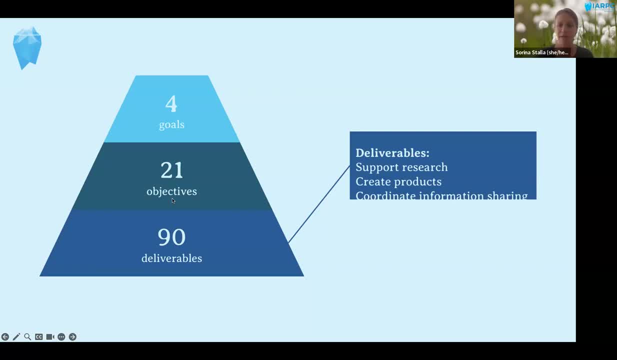 highlight some of the actions in this new implementation plan that are more relevant for the physical oceanography community of practice, But I do recommend kind of looking over the whole plan. The areas I'm going to go over are areas that this community is specifically tagged in, but I'm sure that your interests and your works are relevant to a lot of. 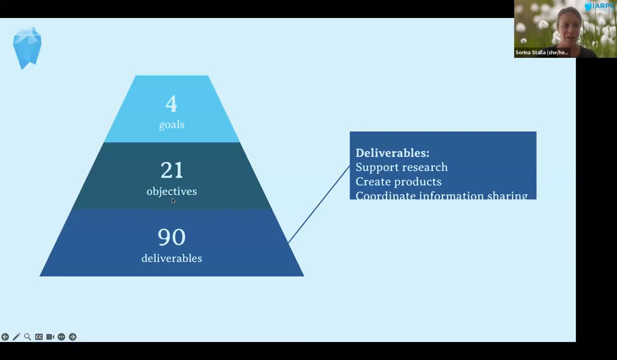 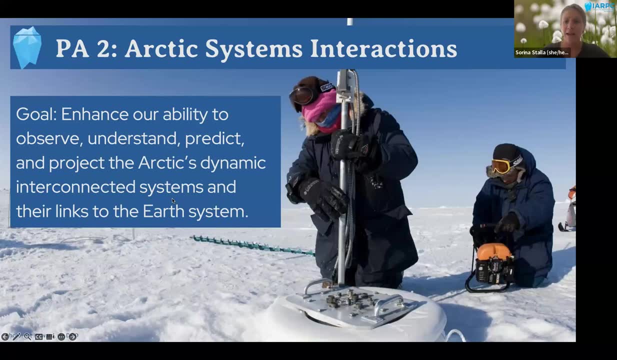 different areas, So always helpful to take a look at the whole thing. So first, our second priority area is Arctic systems interactions, And it has the goal to enhance our ability to observe, understand, predict and project the Arctic's dynamic interconnected systems and their links to the Earth system, And objectives under this priority. 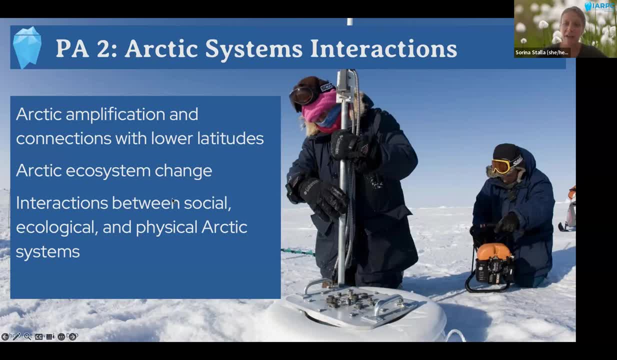 area focus on advancing understanding of Arctic amplification and the associated connections with lower latitudes, observing, understanding, predicting and projecting Arctic ecosystems change and the associated impacts on humans and the entire Earth system, and understanding interactions between social, ecological and physical Arctic systems, particularly 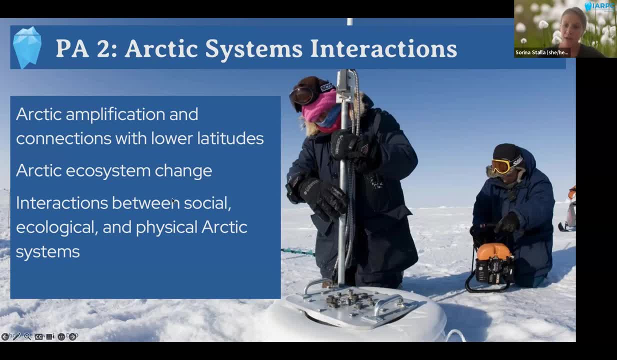 in the context of coastal climate and cryospheric change. So the physical oceanography community of practice is tagged under deliverables, under all three of these objectives, or sorry, yeah, objectives, And I'm not sure how to put this in the chat when I'm 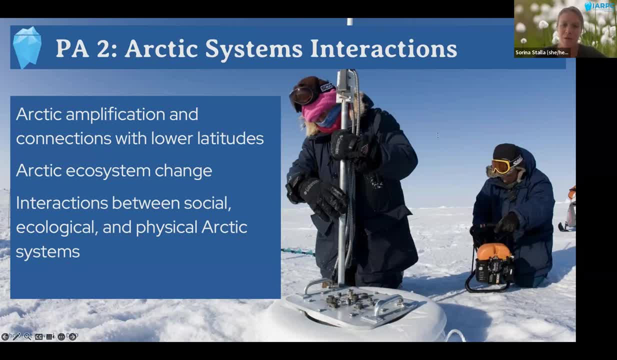 presenting, but I will put in the chat- or maybe Meredith you can- a list of all the deliverables under each of the areas I'm going to go through where the physical oceanography team is tagged, but just to highlight a few deliverables that are have that have been tagged. 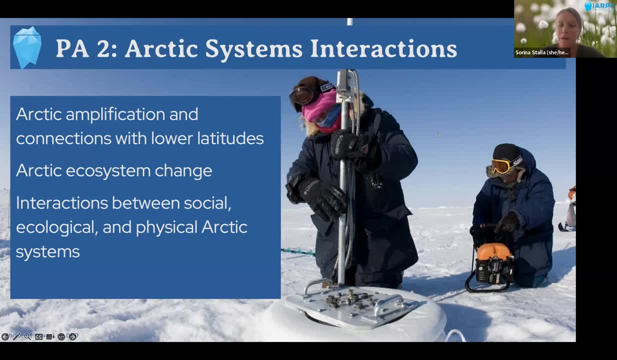 by the physical oceanography community of practice. One of them is to hold cross-collaboration team meetings and workshops and produce publications to explore results of high resolution and regional Arctic modeling, And these meetings will focus on the importance of model resolution to capture Arctic amplification and its relationship with the lower latitudes. 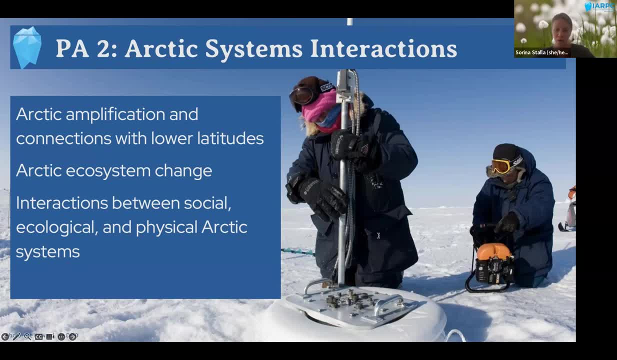 Another deliverable this community is tagged in is to continue coordinated interdisciplinary Arctic marine climate and ecosystem observations and share data and promote synthesis of field operations. And another is to improve high resolution models, ability to capture coastal processes that inter at the interface of ocean, land and atmosphere, by supporting targeted collaborations among model developers. 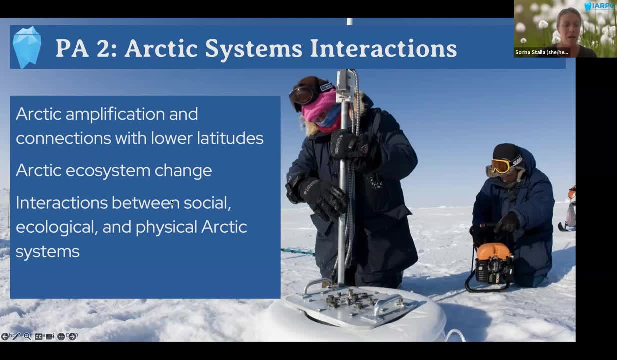 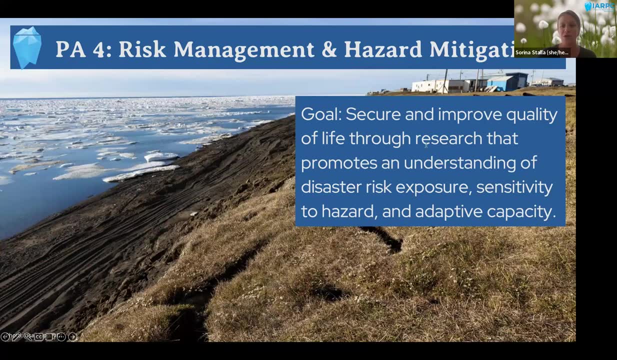 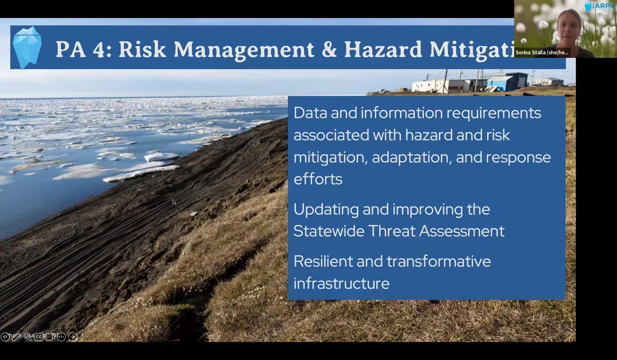 users and decision makers. Our fourth priority area, risk management and hazard mitigation, has the goal to secure and improve quality of life through research that promotes an understanding of disaster risk exposure, sensitivity to hazards and adaptive capacity, And objectives under this area focus on summarizing currently: 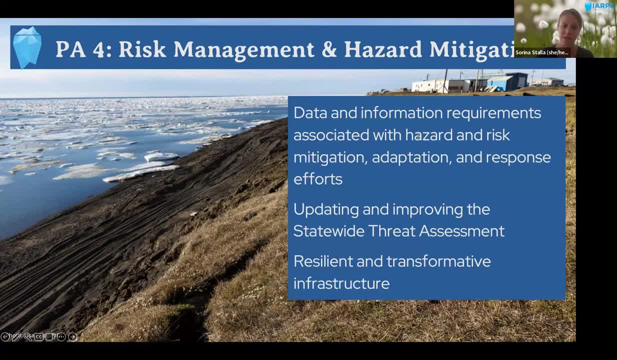 available data and information requirements associated with hazard and risk mitigation, adaptation and response efforts. synthesizing community led activities and information to identify potential needs for future efforts. updating and improving the statewide threat assessment, which is the identification of threats from erosion, flooding and thawing permafrost in. 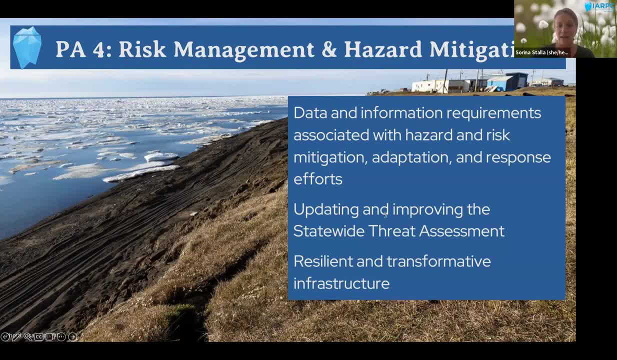 remote Alaskan, Alaska and the Pacific. And the fourth priority area is to continue coordinated collaborative work with the Alaska communities and conducting and supporting research for more resilient and transformative infrastructure to withstand potential impacts from acute and long-term hazards. The physical oceanography community of practice is tagged under the first two. 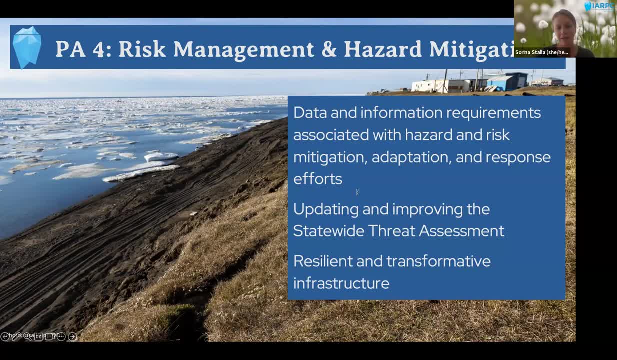 objectives on this work. Some of those deliverables include conducting a study to identify where information used in decision making and planning can be improved through access to newer, additional data sources, And the other is to undertake a study to identify the top 10 threats or hazards to communities and critical remote state, and. 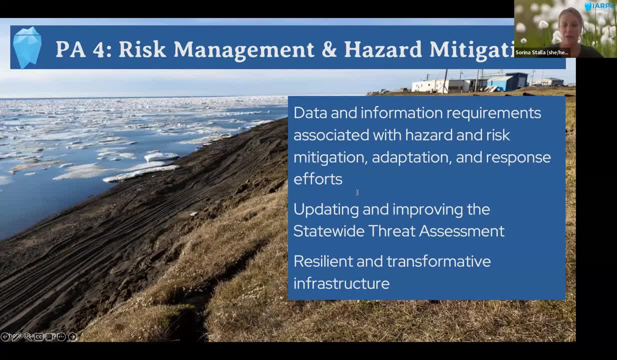 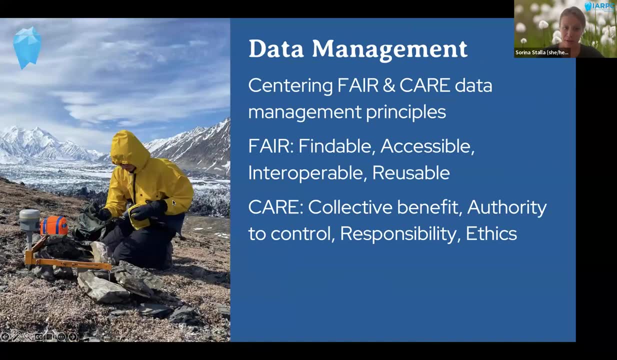 federal government infrastructure in the state of Alaska that should be included in the statewide threat assessment. The data management foundational activity collaboration team is working to encourage and implement fair and care management data management principles in the Arctic And the physical oceanography community of practice is tagged under their fourth objective. 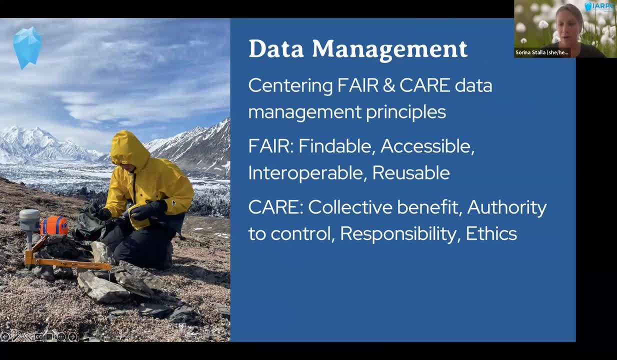 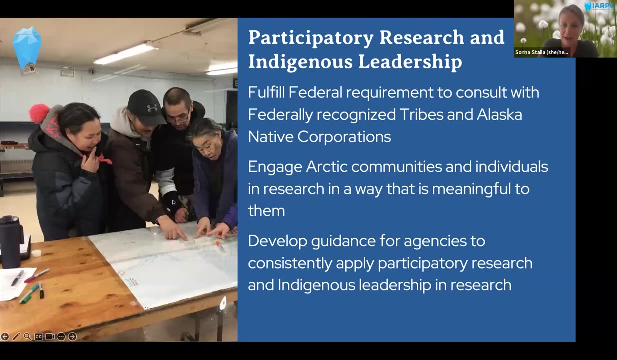 which is to convene quarterly seminars, discussions and training on fair and care data management in the Arctic and ensuring a diverse group of presenters and contributors are represented in these activities. And then, finally, the physical oceanography community of practice is tagged under all of the deliverables in our participatory research and indigenous leadership. 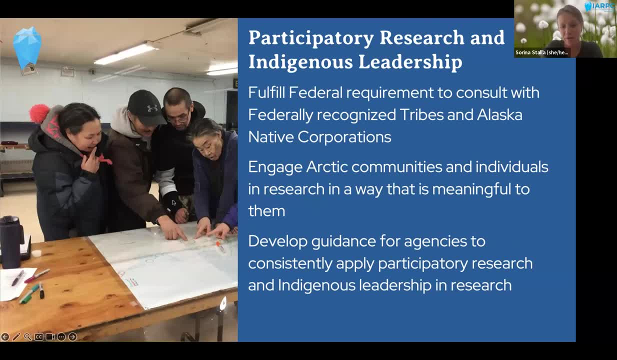 in research foundational activity, And they are focusing on work to fulfill federal requirements to consult with federally recognized tribes and Alaska native corporations, engaging Arctic communities and individuals in research in a way that's meaningful to them and developing guidance for agencies to consistently apply participatory research. 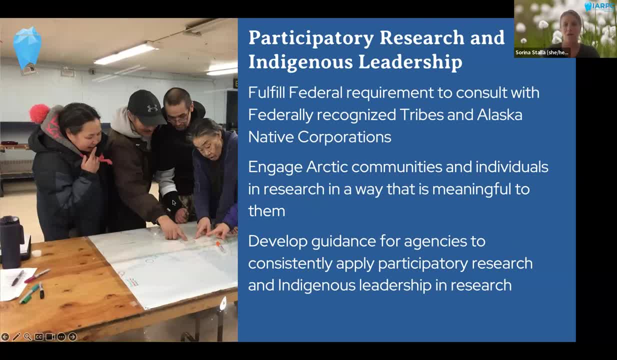 and indigenous leadership in research. So again, you can look at the website for a full list of every single deliverable where the physical oceanography community of practice is tagged. and this is just. these are some kind of key examples from across the implementation plan. 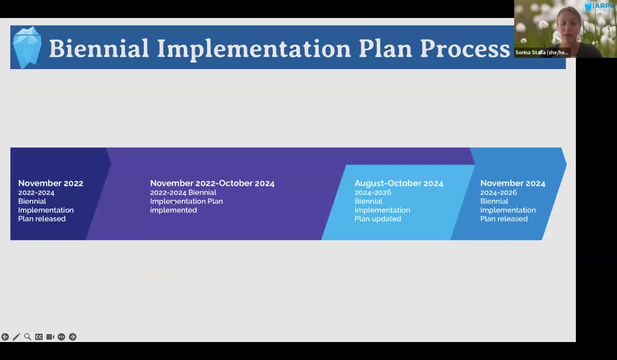 And, like I said, we're currently implementing this first implementation plan. We're going to start the process of updating it late next spring. The update process will be a lot less extensive and kind of happen over a shorter period of time, but that's another way to kind of engage. 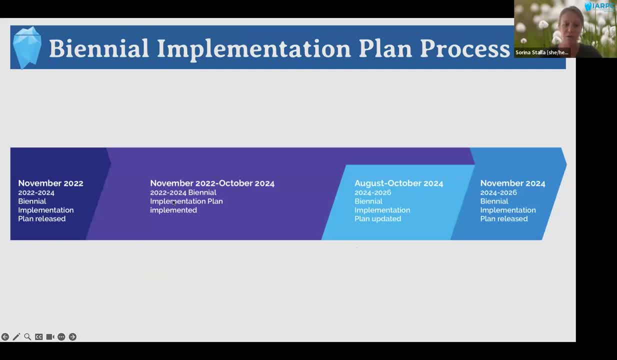 when we start to update, to think about if there's things that are missing or things that should be tweaked. We will begin that process next year and then that updated plan will be released in November 2024.. And we're going to be doing a lot of work to make sure that we're getting that processして. 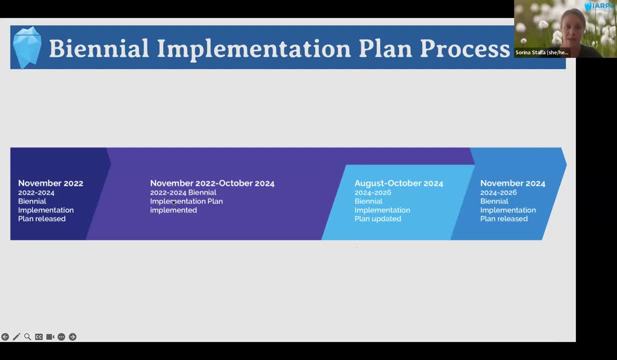 going forward quickly and to make sure that we're getting that process through the next several years and to make sure that we're not just regrowing it but getting it out of the abandonment process. the will be sharing a lot more information about what that process looks like in the coming months. 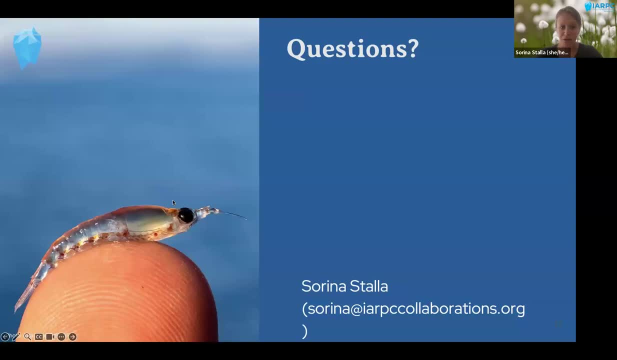 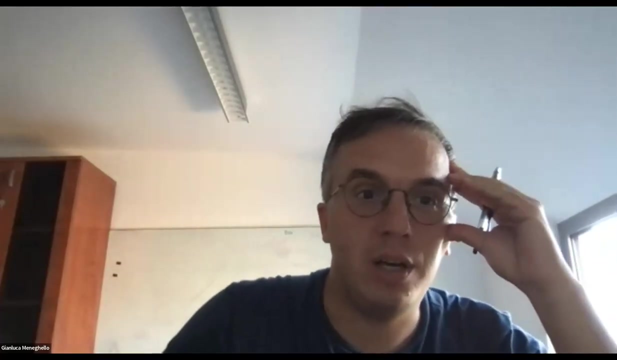 Yep. so that's what I've got for you. I'm happy to answer any questions and appreciate you all engaging with IARPC and on these important research questions. So thanks everybody, Thank you. Thank you, Serena, for your presentations. I would suggest maybe we can. 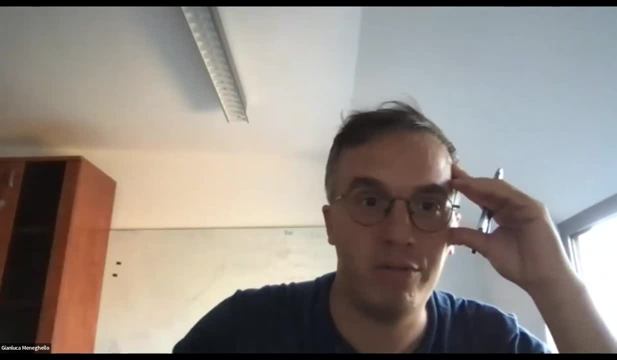 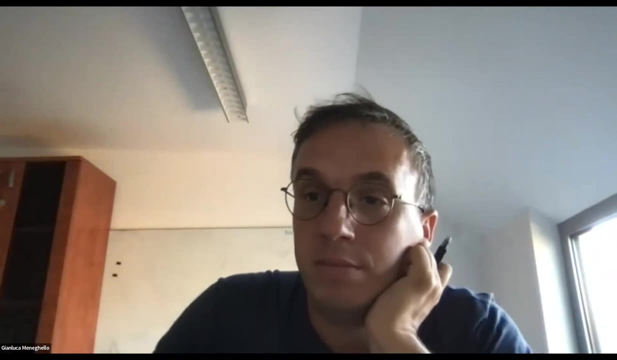 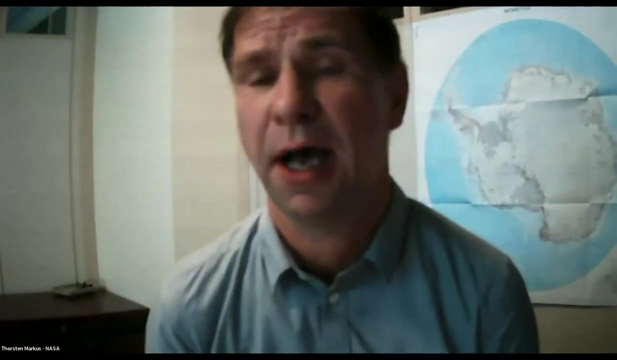 go through all the speakers and then have questions at the end to collect everything together. So next up, Thorsten Markus from NASA. Thorsten, if you want, Yeah, hi, Good afternoon or good morning, wherever you are. So I'm Thorsten Markus, I manage the. 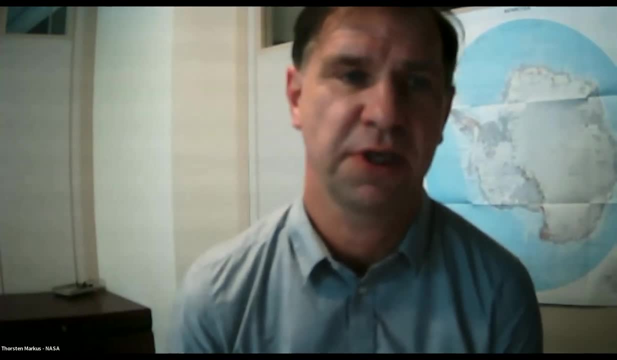 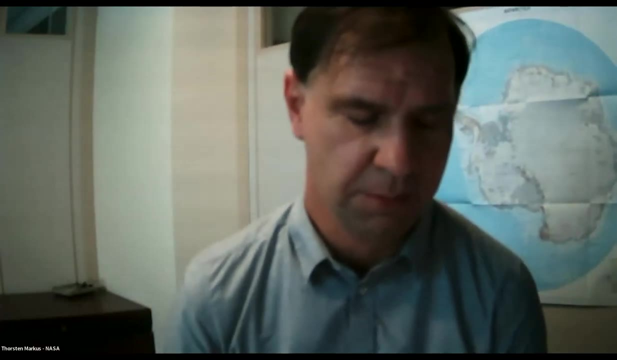 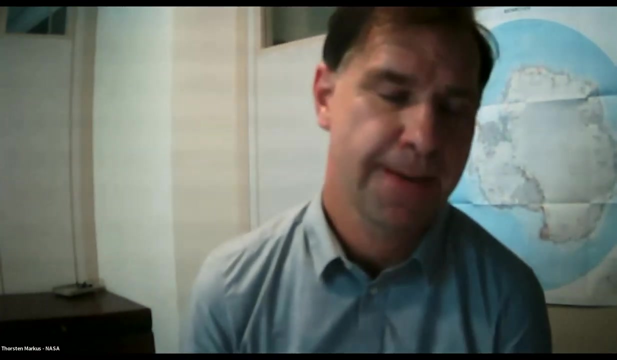 cryosphere program at NASA headquarters and I am also the program scientist for the ISAT-2 mission and the CRYSTAL mission, the Earth System Explorers, as well as the National Snow and Ice Data Center. So you know changes in the Arctic Ocean, especially the decline of the sea ice. 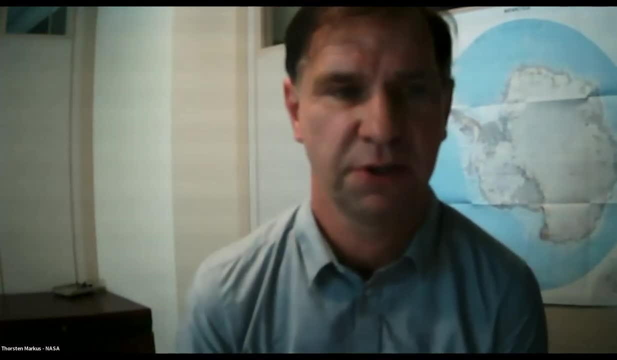 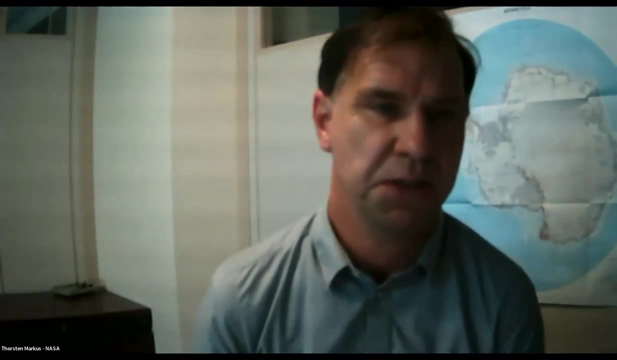 among you know, obviously you know the clearest harbingers of climate change And, you know, maybe directly related to priority area two, you know, while a lot of science is happening in the Arctic Ocean, fundamentally you know climate change is happening in the Arctic Ocean And you know. 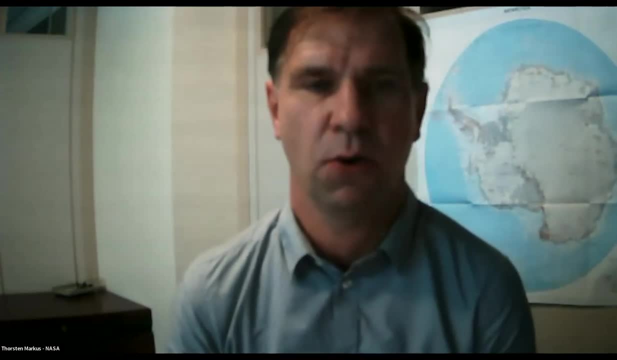 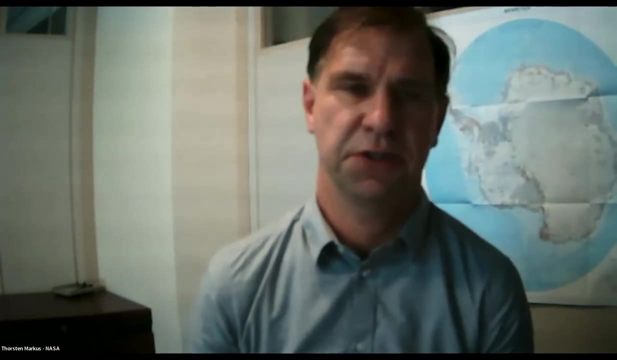 you know, while a lot of science is happening in the Arctic Ocean, fundamentally, you know, by NOAA, by NSF, by NASA, by, you know, the ONR Office of Naval Research, many of the processes are still not sufficiently understood And models still have a hard time replicating. for example, 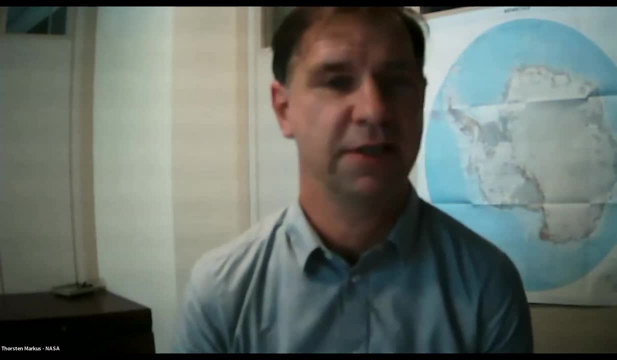 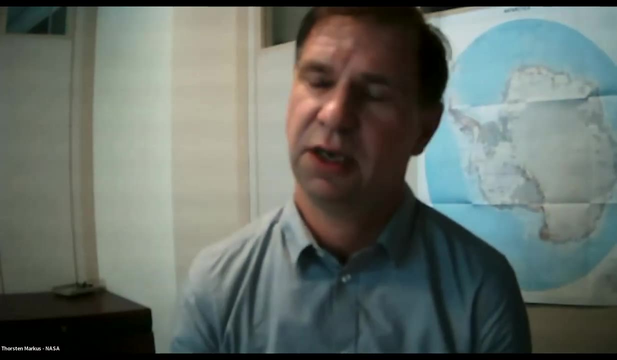 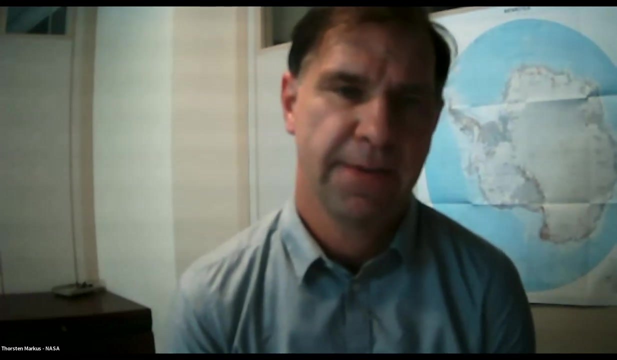 the summer sea ice cover Models cannot still not predict it, And there are various reasons for it, And you know. and then it's largely because our understanding of ice, atmosphere, oceans, interactions still need to improve And in the Arctic there are many small scale processes, for example melt ponds. 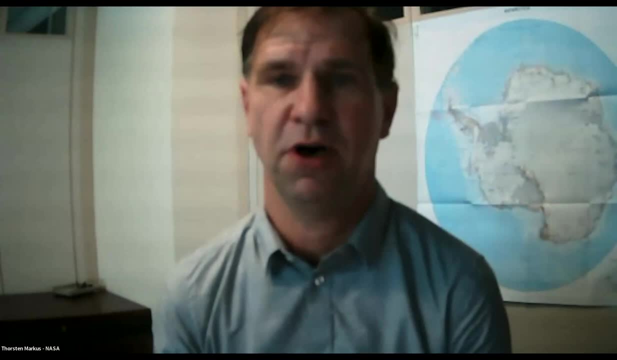 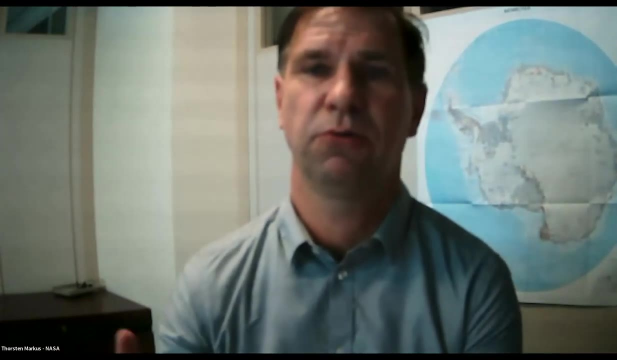 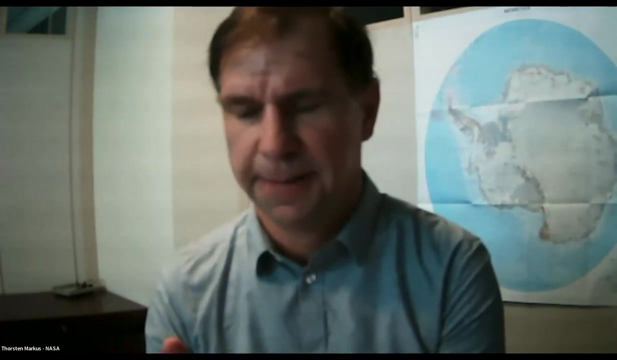 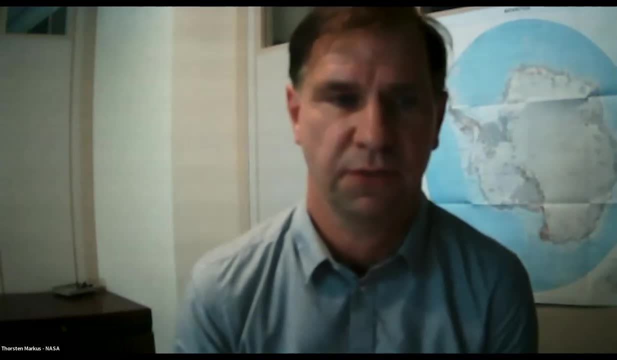 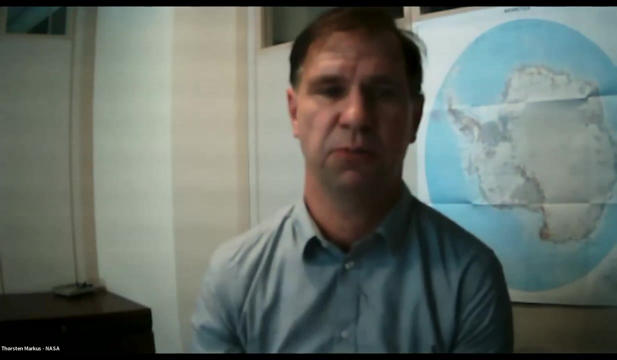 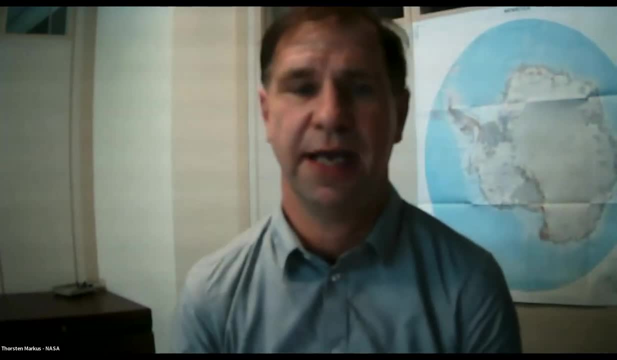 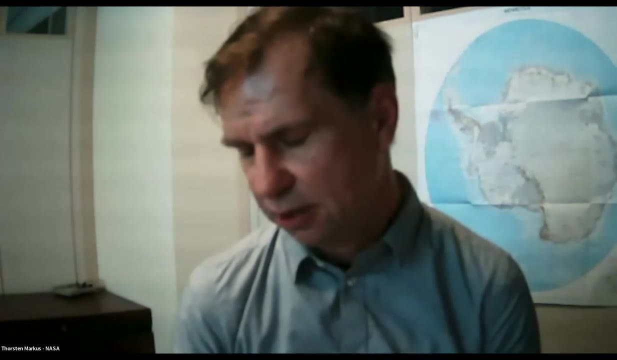 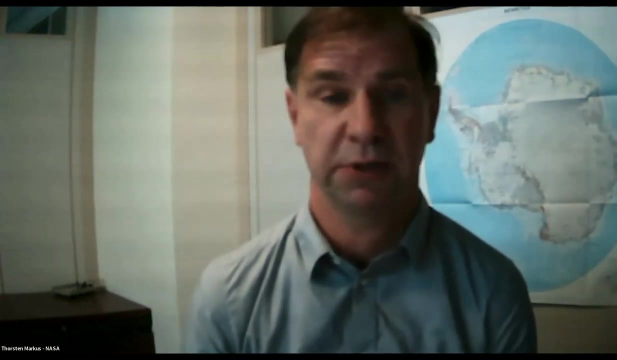 so rapidly to, you know, to the changing changes in atmospheres and and atmosphere and ocean conditions. So at NASA Arctic physical oceanography is generally covered and supported via several programs. You know there is obviously we do have physical oceanography program which is led by 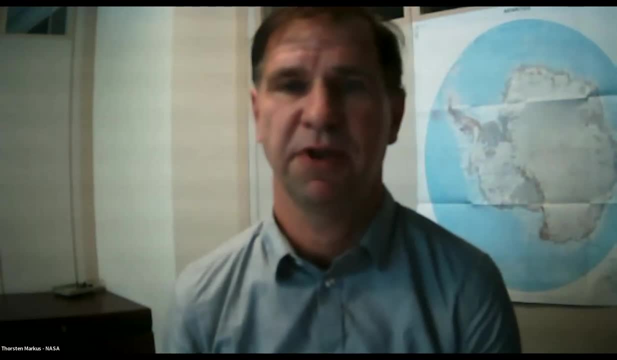 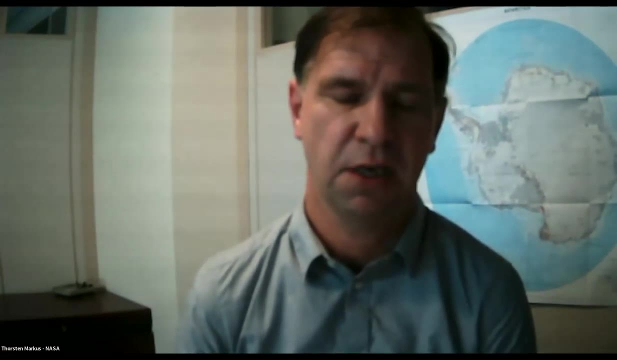 Nadia Rino-Gordoba-Schiffer. We have the cryosphere program that I manage. We have the modeling analysis and prediction program, which is managed by David Considine. We have an interdisciplinary program. We have the OBB ocean biology and ocean biochemistry program. 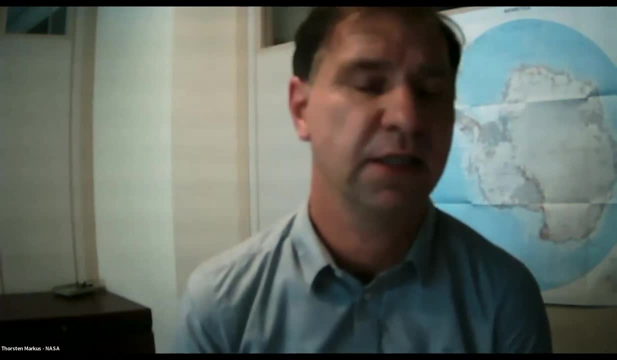 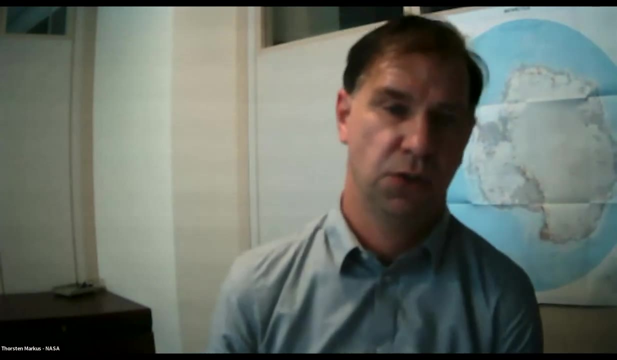 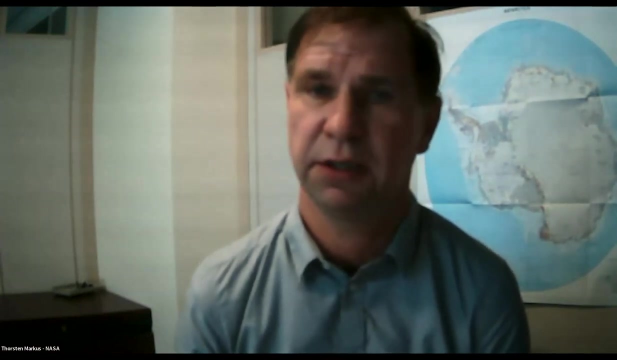 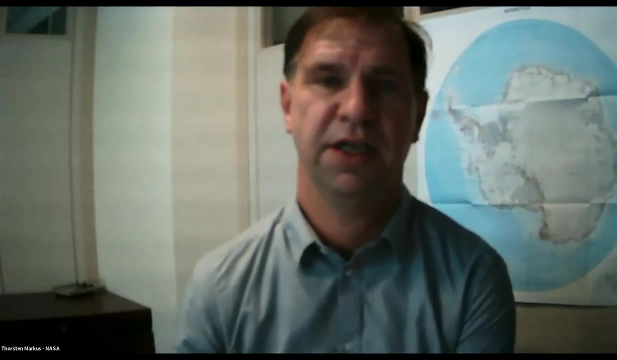 And then we have lots of missions, mission science teams like SMAP, SWAT, ISAT-2, that you know provide relevant data for the Arctic. We also had a longer-term effort called OMG- Ocean Smelting- Greenland, where the focus was on understanding how the ice sheet and the 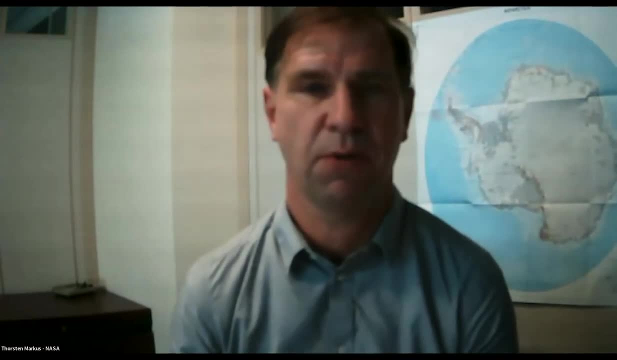 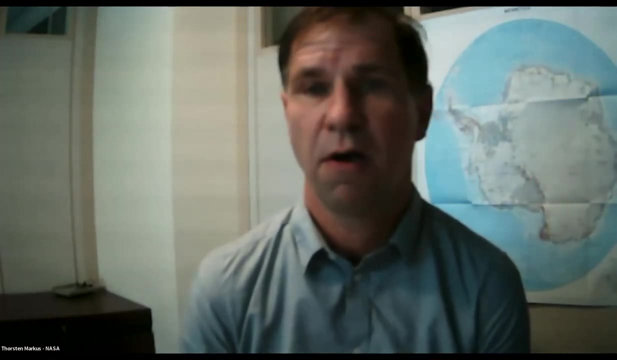 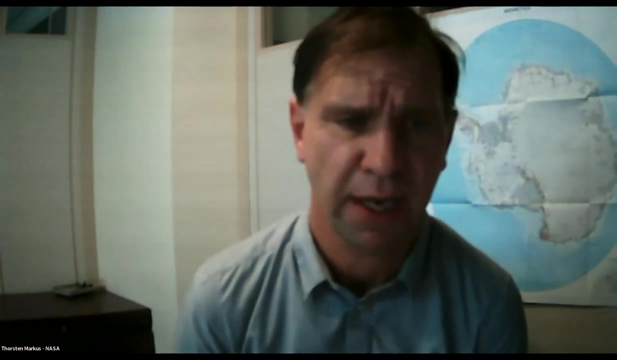 ocean interact with each other. It was a combined. it was an effort that used airborne data, that used gliders in the ocean to better understand what's happening under the outlet glaciers of the Greenland ice sheet, And we also had supported a field campaign. 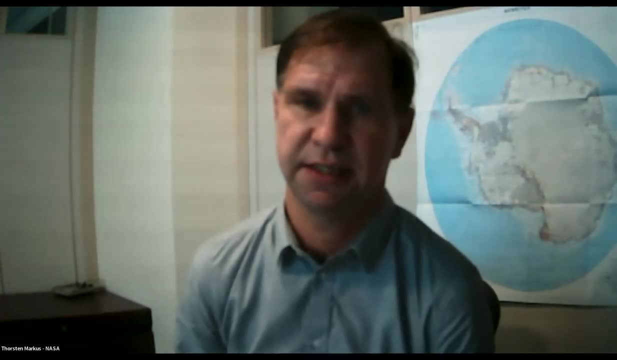 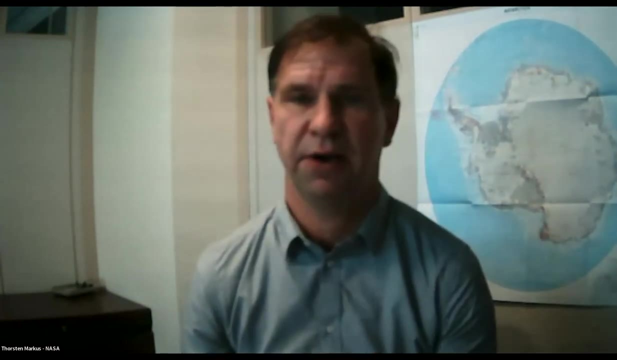 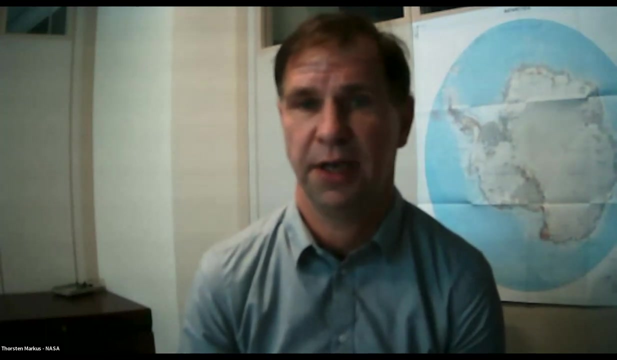 last year called SASIE, S-A-S-S-I-E, which stands for salinity and stratification of the sea ice edge, where people collect the data of the sea ice of the ocean underneath, etc. to better understand What's going on at the marginalized zone. Because, as I said in the beginning, those are the processes. 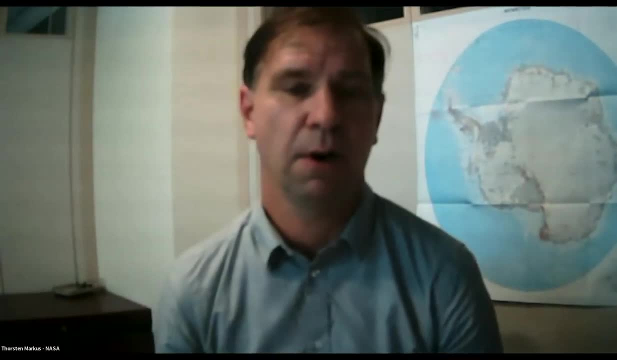 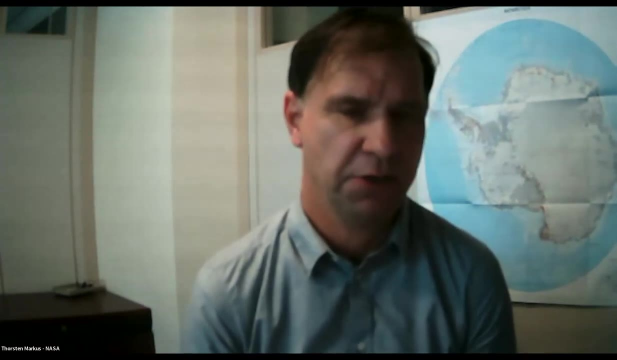 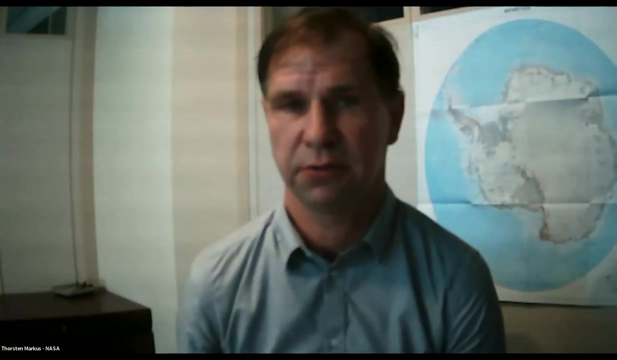 that are so hard to model, so hard to observe, And we support, you know, within the cryosphere program that I manage we have, we support a lot of efforts that deal with sea, ice, ocean interactions, often using remote sensing data, but we also support a lot of modeling. 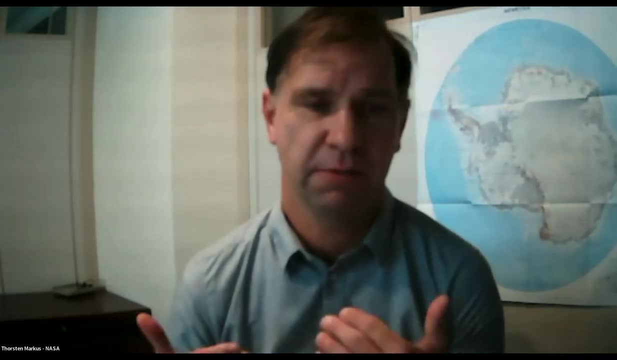 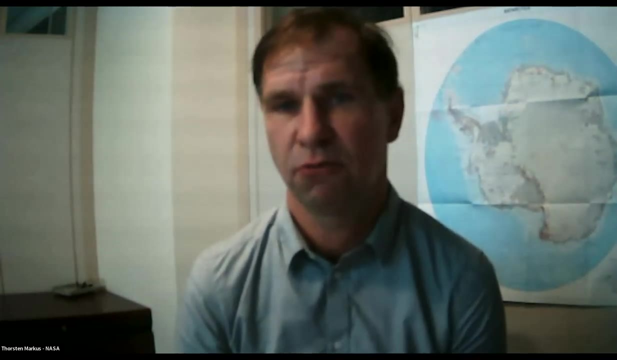 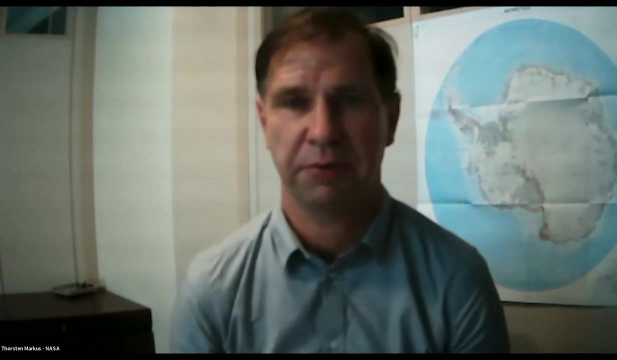 So we- I don't know, you probably know this- We scientists can apply for funding using our annual ROSAS calls. ROSAS stands for research opportunities in space and earth sciences, which comes out every February, And I encourage you not to look. 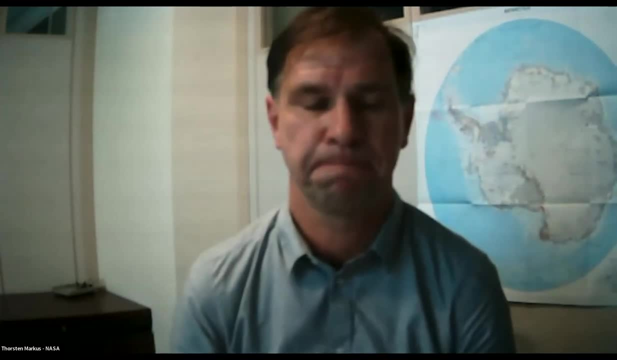 at the physical oceanography opportunities. but there are other opportunities like ocean surface salinities, such as MISS EXPLNижу, the Classic U pool, fiberhub, навер, whatever. So there needs to be unique organizations that are based in those areas. 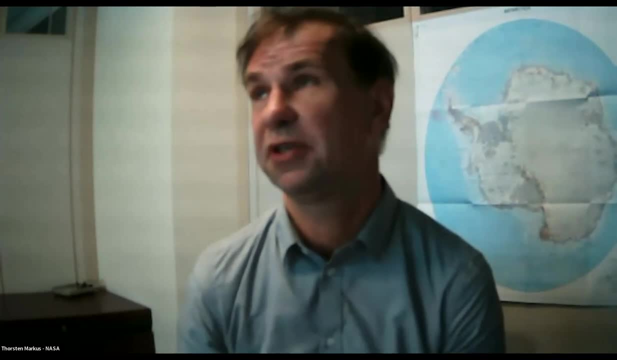 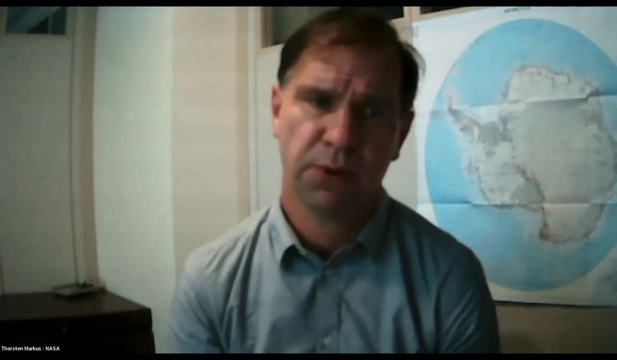 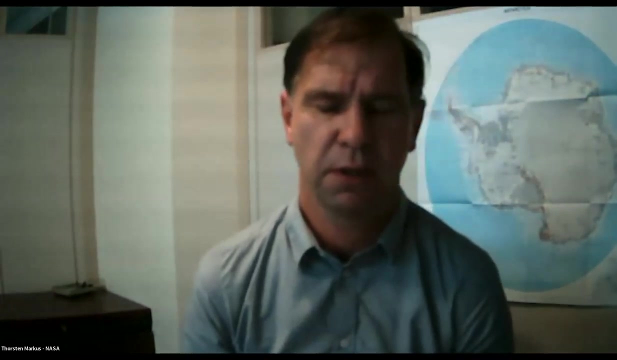 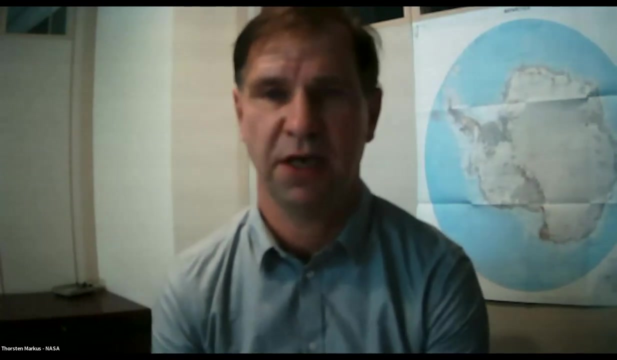 team, ocean surface topography team, the modeling calls that are coming out, the cryosphere calls that are coming out and reports like the IARPIC research plan, like the IPCC report, are often mentioned in our calls because they guide us, you know, to what we should be funding. 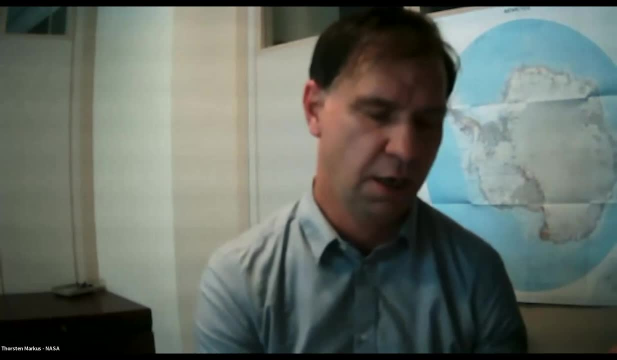 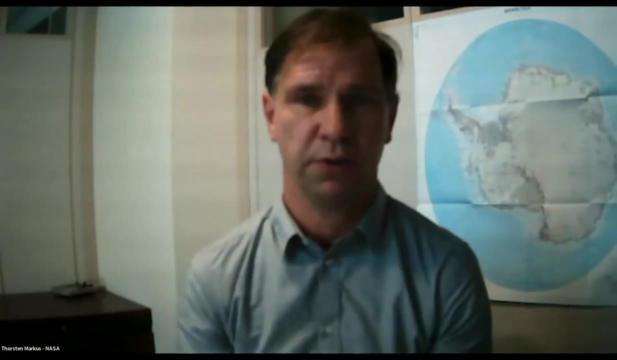 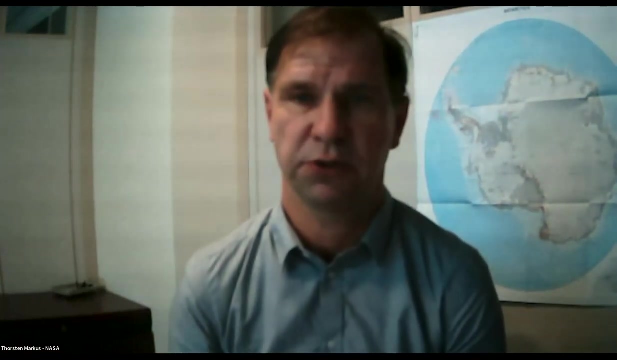 what we should be focusing on. So these efforts like IARPIC, IPCC, obviously CLIC, climate and cryosphere, those reports are very important to give us a guidance of what we should be supporting. So we often mention those reports, like the Arctic research plan, the IARPIC Arctic research. 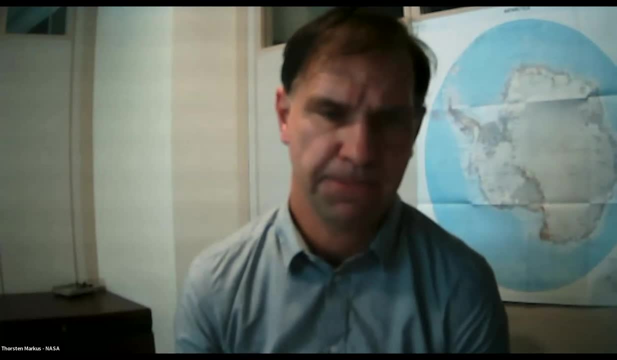 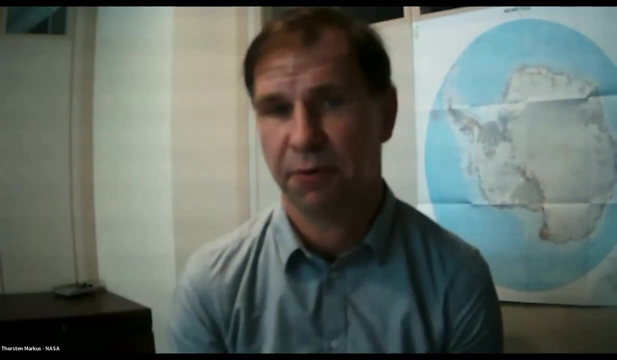 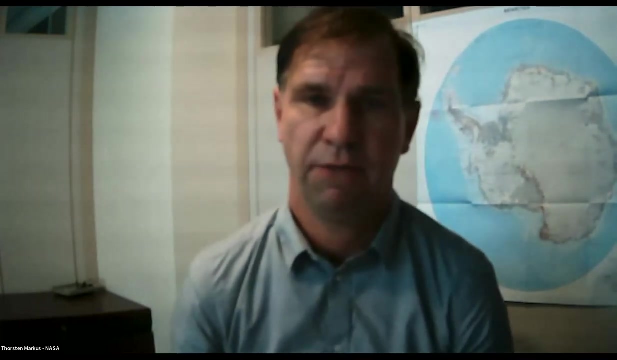 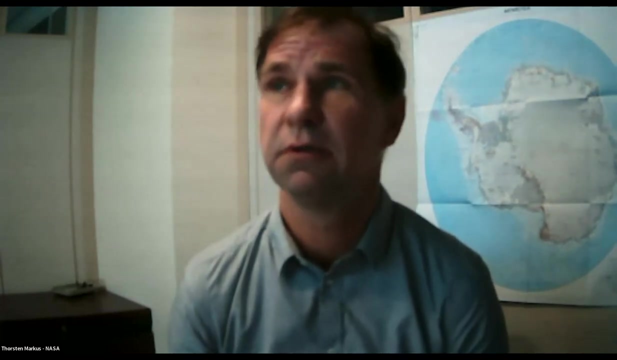 plan in our calls For the scientists of you all, of our satellite data and derived geophysical data. you know physical products are publicly available via our data centers for physical oceanography. We have the physical oceanography deck, the distributed active archive center at JPL or 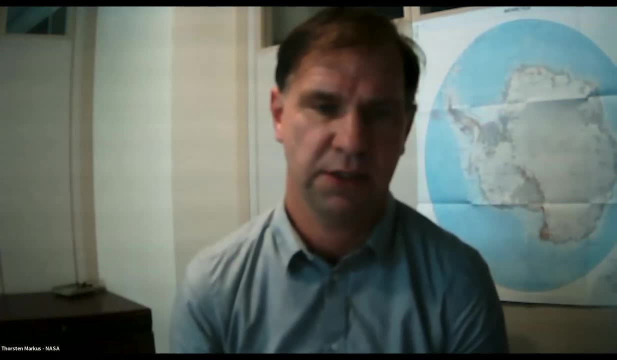 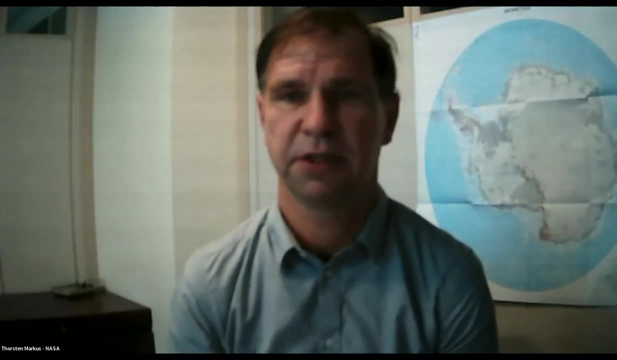 it's for the cryo data, it's at the National Snow and Ice Data Center. As I said, all those data are freely available. all those products are freely available And I realize sometimes that you know the data is available. 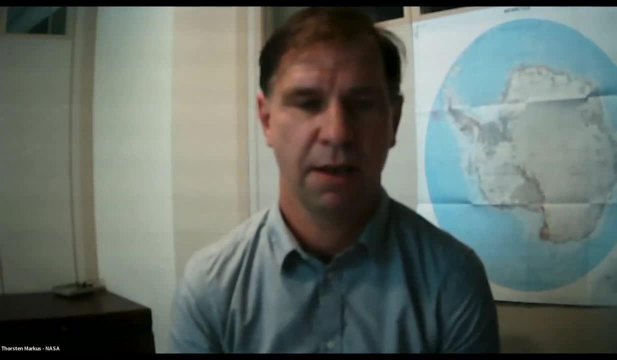 And I realize sometimes that you know the data is available. And I realize sometimes that you know the data is available, But it's probably less people know about them at times that I expect. So I'm just making another announcement. 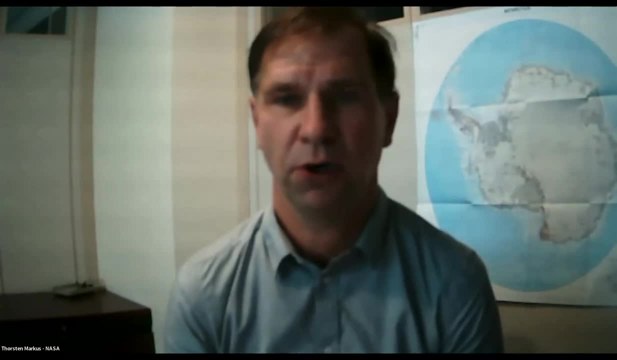 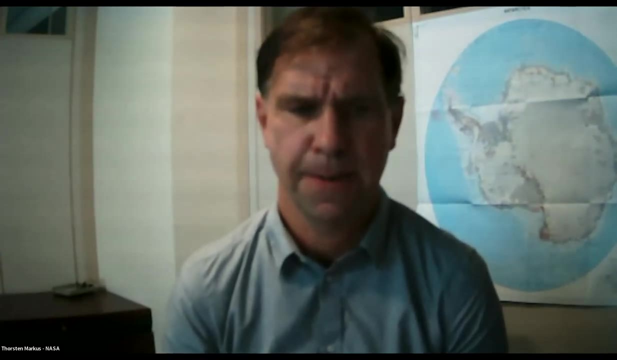 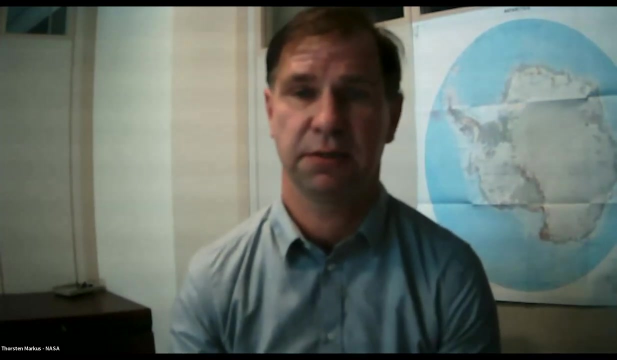 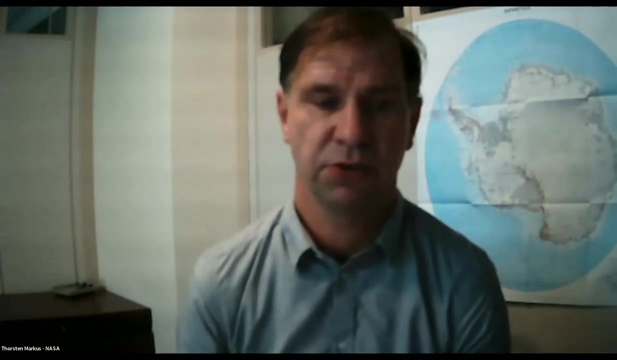 You know, please check out the data. You can also go to earthdatanasagov to check out what data are available to the public community. We have an open data policy, So all data that are collected through NASA funds are publicly available. That includes airborne data, in situ data, et cetera. 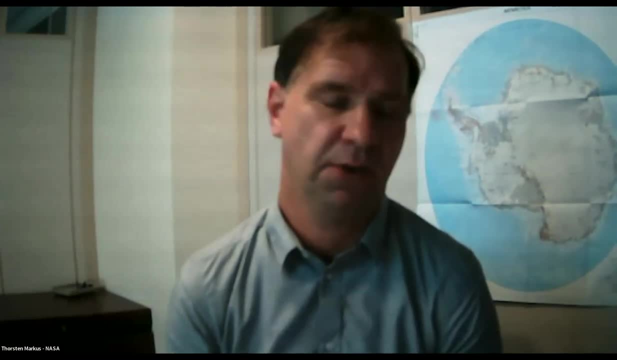 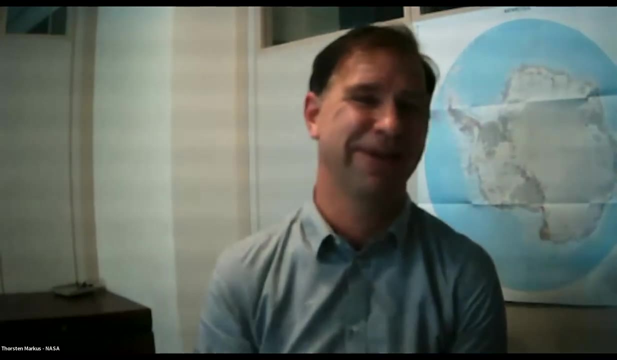 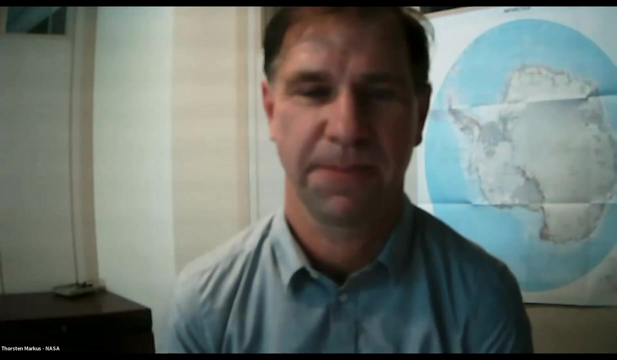 So they're all publicly available somewhere as well, depending on the discipline, And I think that's my five minutes. I can talk forever, but I wanna stick to my five minutes, Thank you. Thank you very much for your presentation. I'm a big fan of the NASA data. 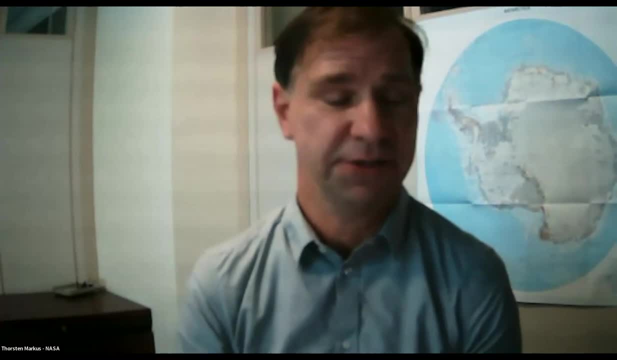 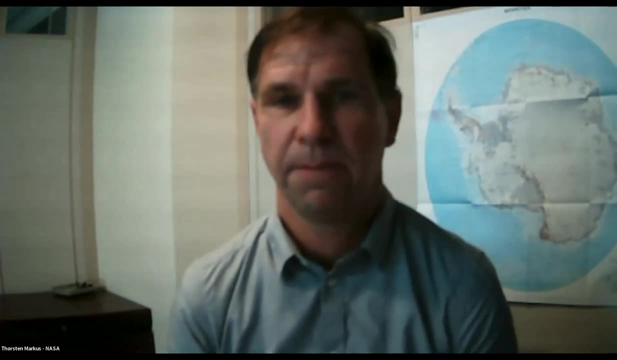 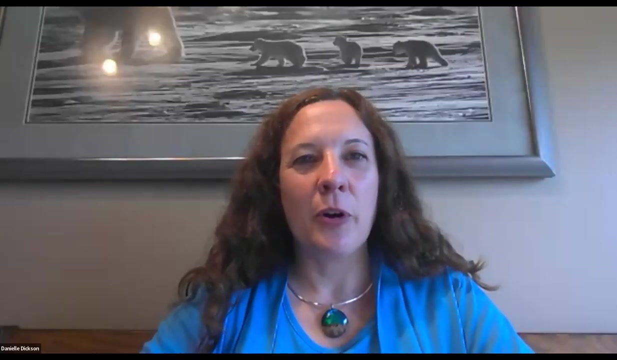 and I've been using them a lot, so I will have a question about it later, probably. Next up is Danielle, are you there? I am Thank you for having me. So hi, my name is Danielle Dixon. I am a program manager. 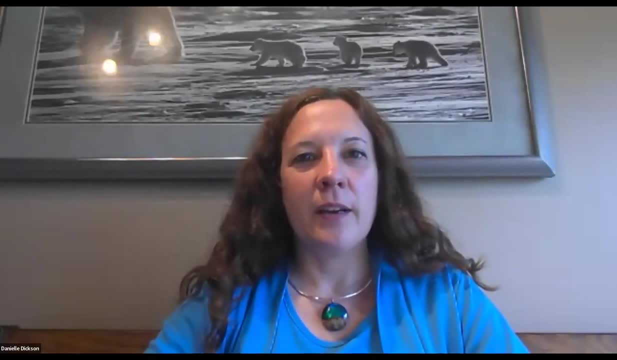 with the North Pacific Research Board, So we are not a federal agency. We are an organization that provides funding for marine science research in Alaska waters And our mission is to fund research to address ecosystem data and information needs and pressing fishery management needs. 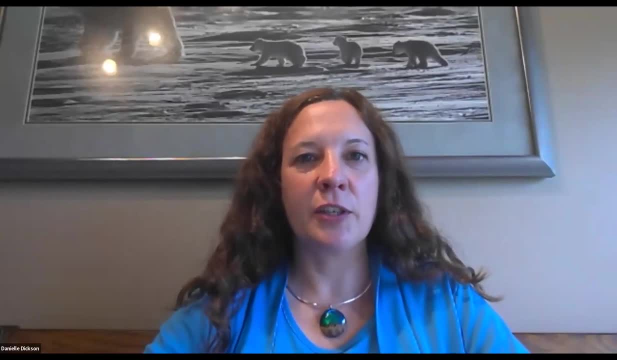 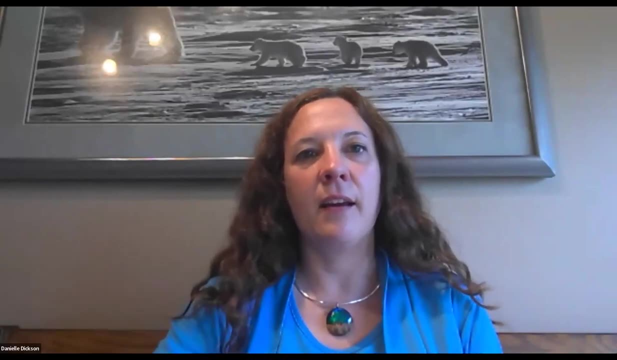 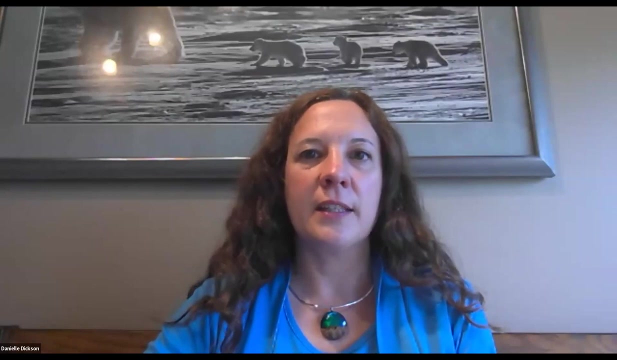 So I'll just highlight a few things for this group to think about that I hope will prompt some conversation during the breakout or afterwards during the Q&A and prompt you to think about some ideas for your next proposals. So NPRB is interested in a number of things. 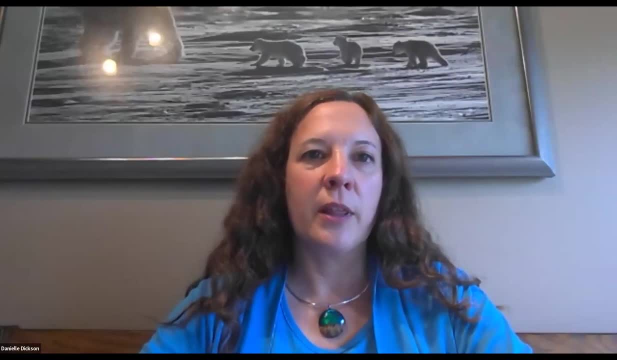 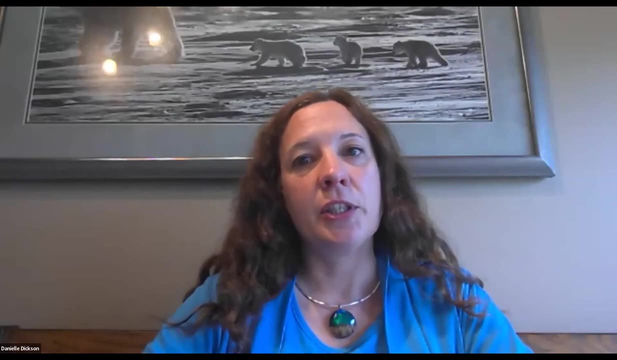 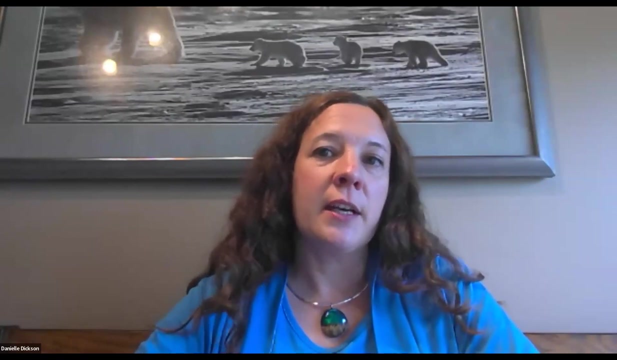 But, for example, there are some clear intersections with the IRPIC Arctic research and research aufmerksam plan and the biennial implementation plan, things like opportunities to support co-production of research with Alaska communities and research as relevant to communities, including projects. 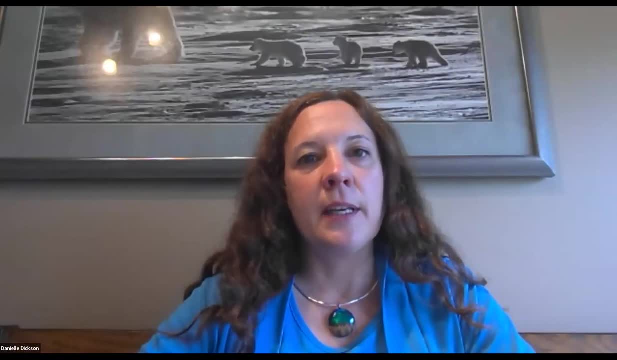 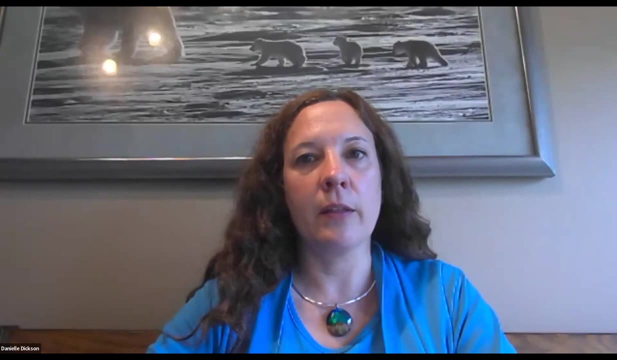 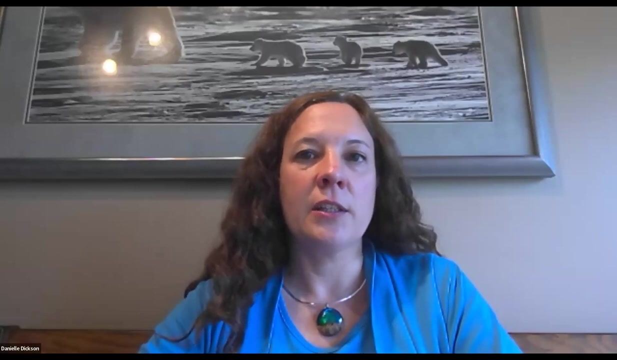 that cooperate with community-based observers. So some examples about you know where communities might be interested in collaborating with the physical oceanography community of practice include things like looking at how physical oceanographic conditions, including water temperature, stratification, light penetration and nutrient inputs from a terrestrial system. 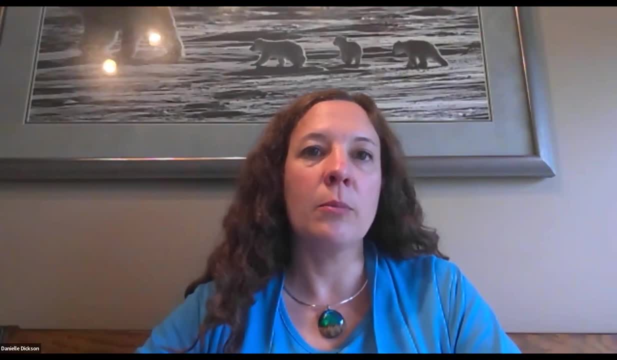 influence the magnitude, location and timing of harmful algal bloom events that have some real pose, some real threats, not only to the marine ecosystem but also to people living in the Arctic, with respect to food security and health, for example. Another 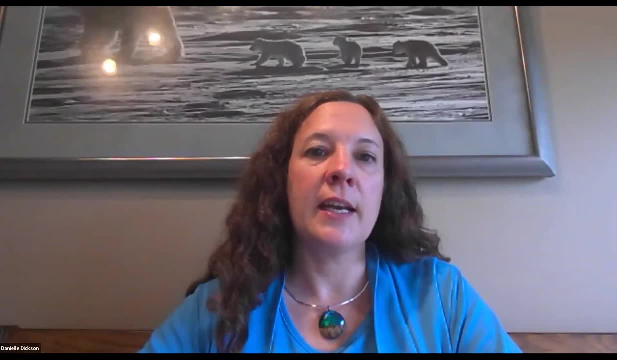 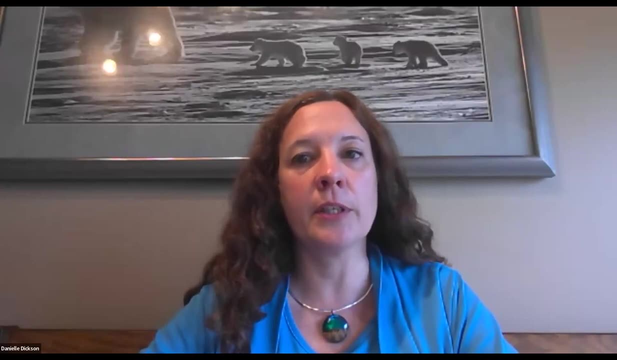 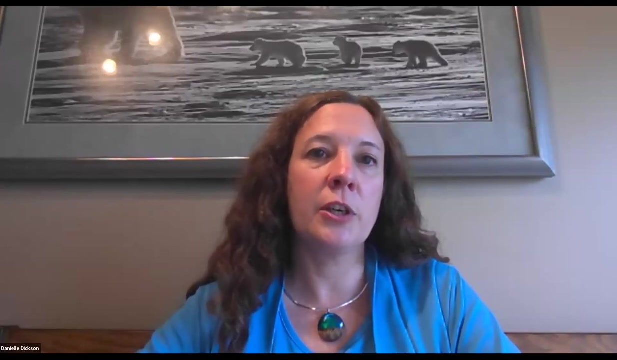 example might be how interactions among the ocean, the sea ice and atmosphere influence sea ice stability and sea state. that affect the safety of Arctic community members when they're going out to do things like subsistence harvests. that affect their own safety but also the food security of. 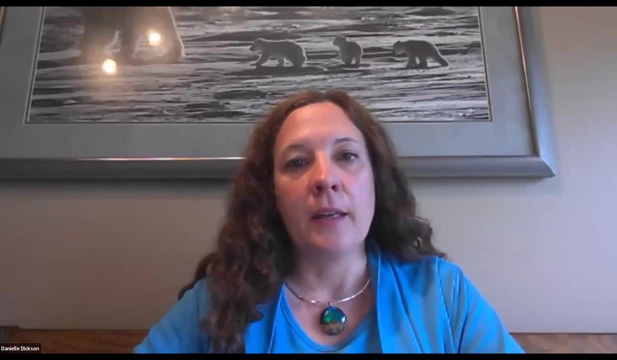 the communities that they're providing for. And then NPRB is also quite interested in opportunities to support multidisciplinary collaboration to better understand things like the factors influencing the climate change and the climate change in the Arctic. So you know, we're also interested in how the fishing community is influencing the distribution. 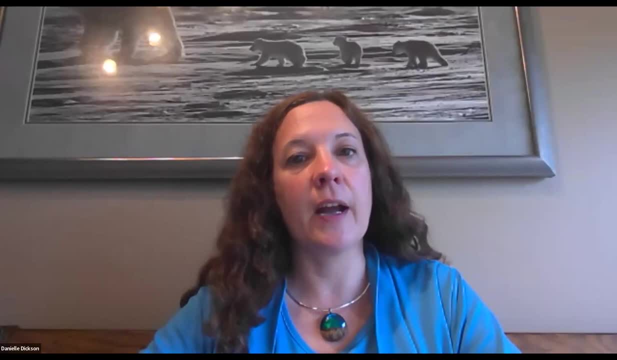 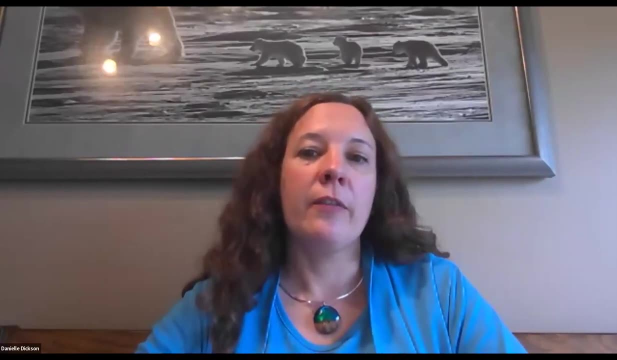 abundance and condition of marine species, for example Pacific cod, walleye, pollock, crabs, salmon, protected marine mammals and seabirds. So think about how the physical oceanography community of practice could perhaps provide indices that are relevant to monitoring. 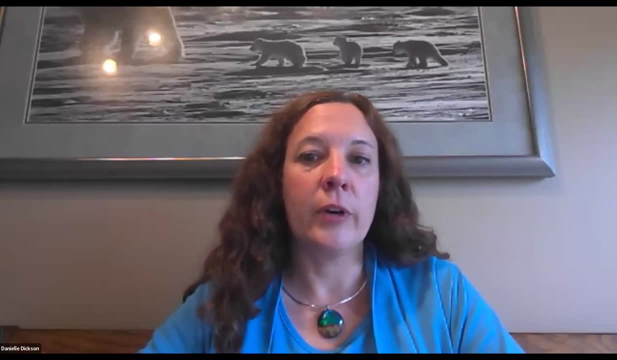 these resources And can we advance capacity for forecasting on time scales that are more relevant to fishery management and other resource management? We also, I think, need to consider reducing the number of fishing areas in the Arctic, as well as reducing the number of areas in the Arctic. 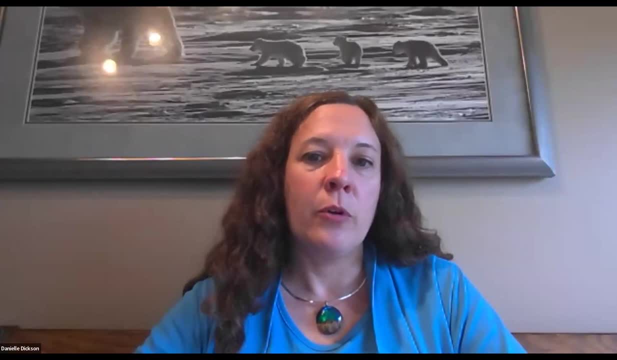 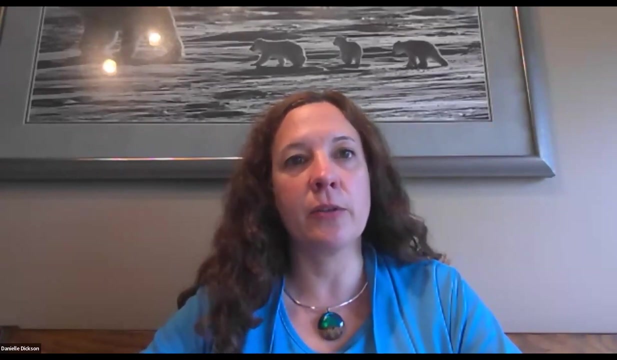 We also, I think, need to think about how the marine environment can be used as a means of more information on winter and early spring oceanographic conditions that influence marine ecology, and maybe some technology development that could make that information more readily available on timescales that are relevant for management. So sea ice cover poses a real 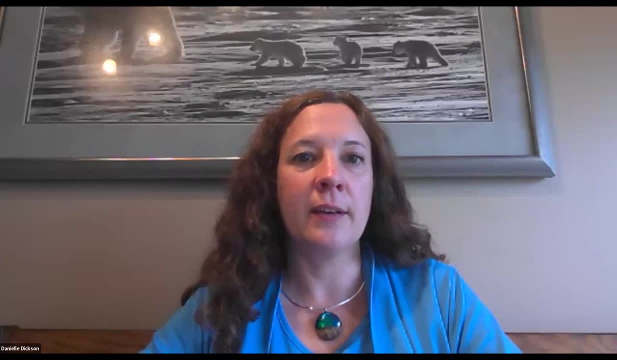 challenge to telemetry data from the ocean in near real time. in the Arctic So often we have moored instruments that sit on the seafloor and the data are collected once per year, but by the time fishery management has that information they've kind of missed the mark for setting. 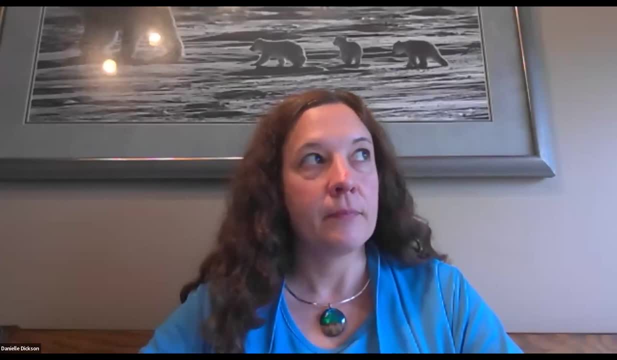 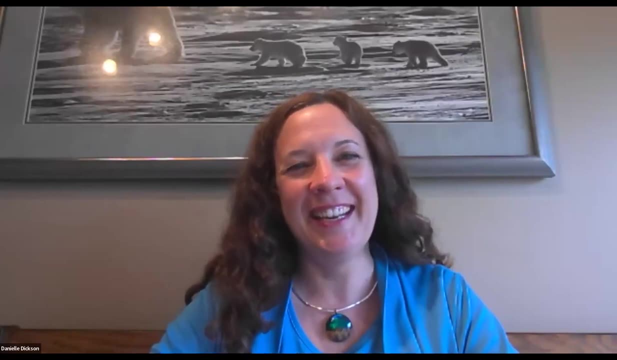 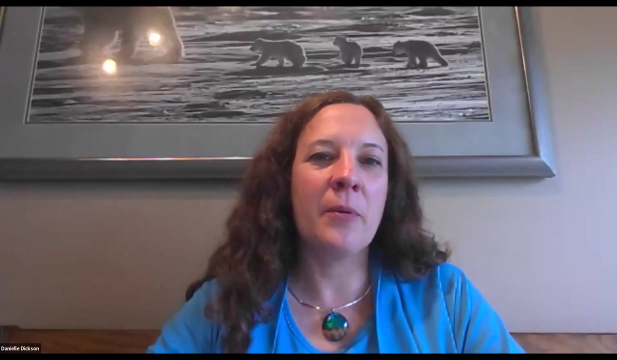 management for managing the resources. And then the other thing I put down in my notes is just always the interest in improved understanding of exchange between offshore and neoshore ecosystems. We have people that do research in offshore and there are people that do research in the neoshore. 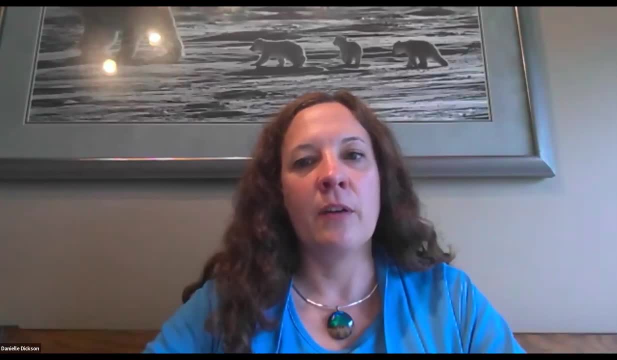 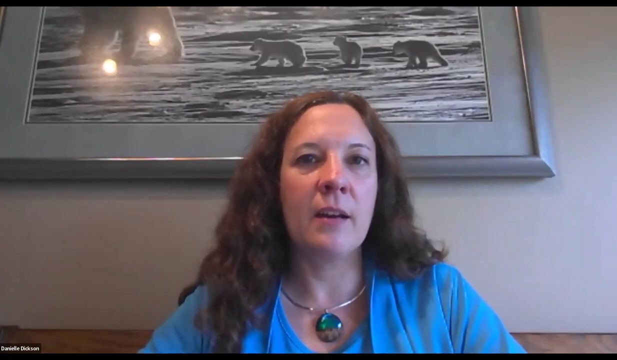 but really making those connections between offshore and neoshore conditions and how they affect the resources that people are trying to harvest, for example. So that's what I wanted to say with my five minutes. I'll just really briefly hit on some things that North Pacific Research. 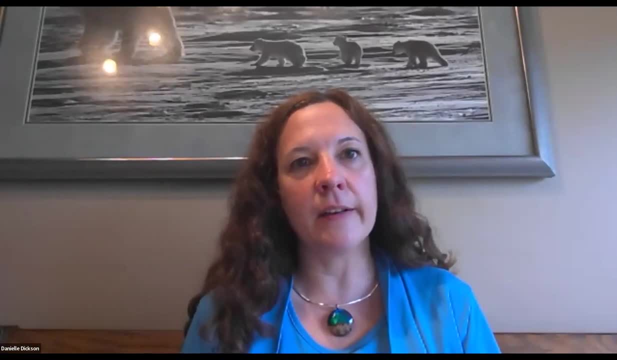 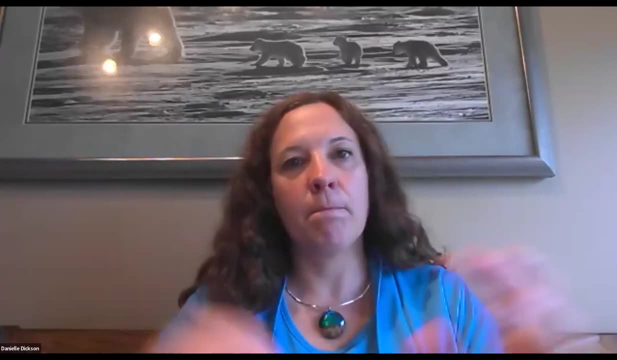 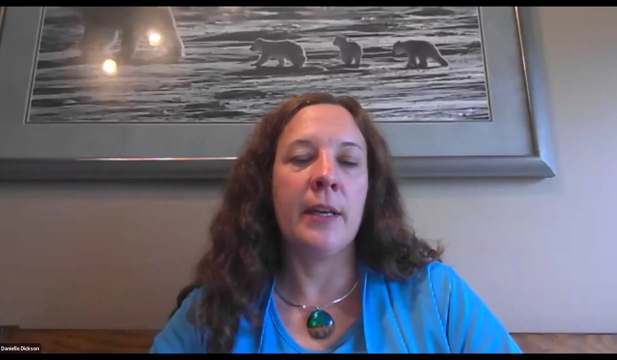 Board is funding now and the programs that we offer funding under. I manage an integrated ecosystem research program. So these are programs that kind of bring together a number of scientists to collaborate over a scale of maybe five or six years to really look at those marine ecosystem processes in detail that connect the physics 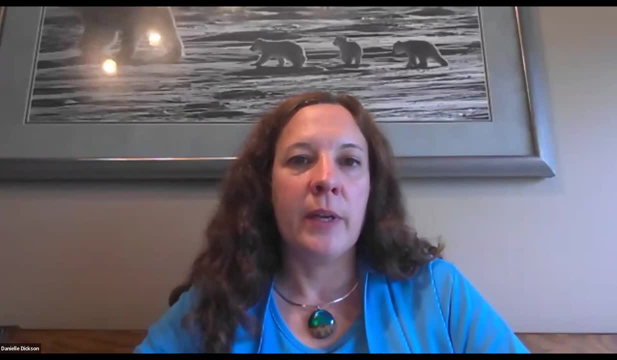 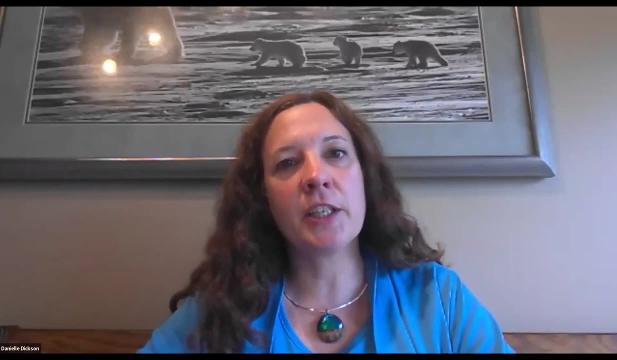 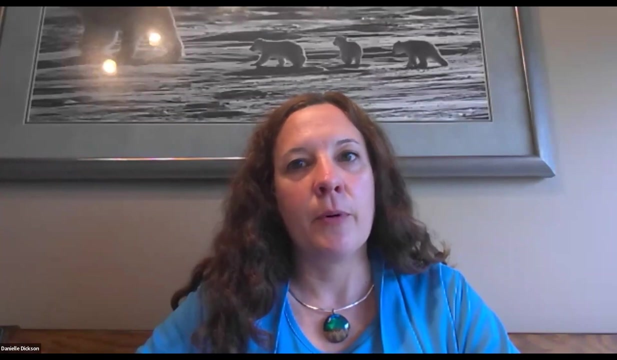 and chemistry all the way up through the food web, And so we recently had an Arctic-focused program that focused on Bering Strait and the US Chukchi Sea, And that one's finished. now, If you look at our website, PRBorg, you can see all the data collected by that program and the reports and some videos. 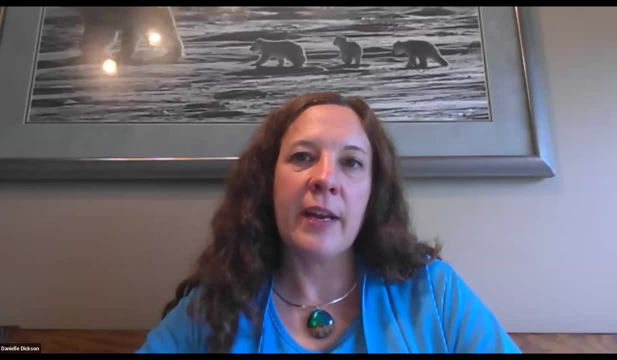 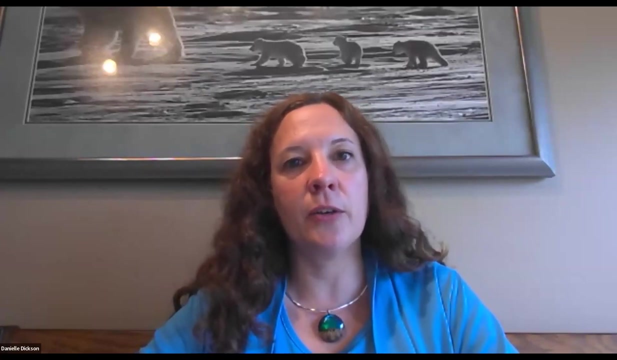 about it And we're in a synthesis phase right now And Sandy's program she's going to talk about is co-funding that synthesis. So it's taking field data collected by our program and others and using them to update models, So ecological models and models that look at nutrient dynamics. 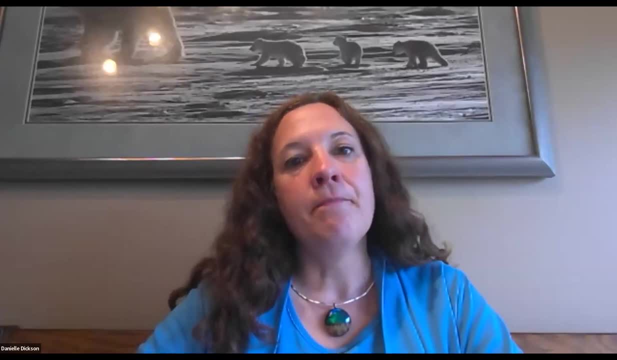 that fuel primary production, for example, And we're about to launch a new North Pacific Research Program, So we're going to be doing a lot of research on that. We have a Northern Bering Sea-focused Integrated Ecosystem Research Program and we expect to 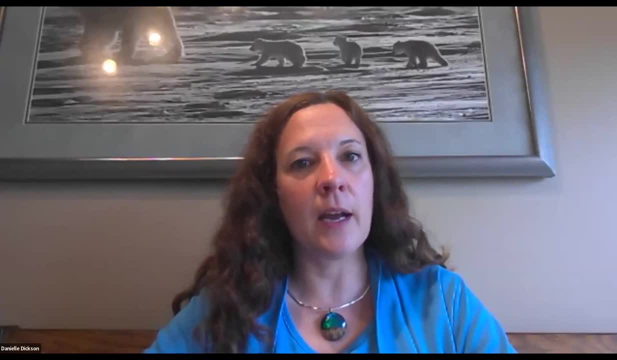 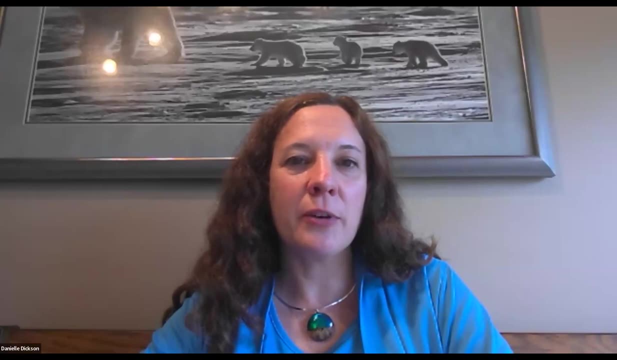 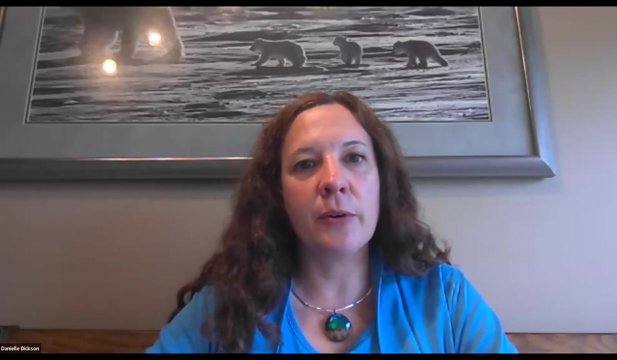 release a call for pre-proposals next month for that program. So that'll be kind of our next decade of research in the integrated sphere. We also offer funding under a long-term monitoring program. So, for example, for 10 years we've been funding a Chukchi Ecosystem Observatory. It's an array of 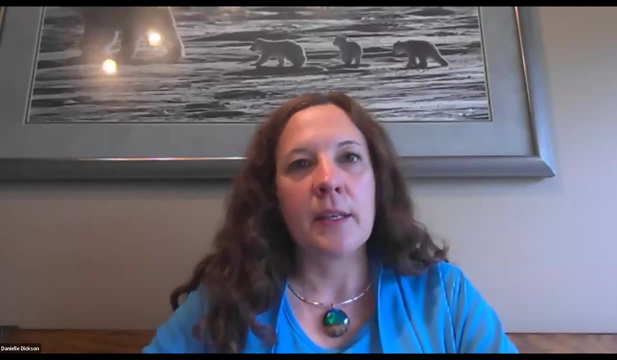 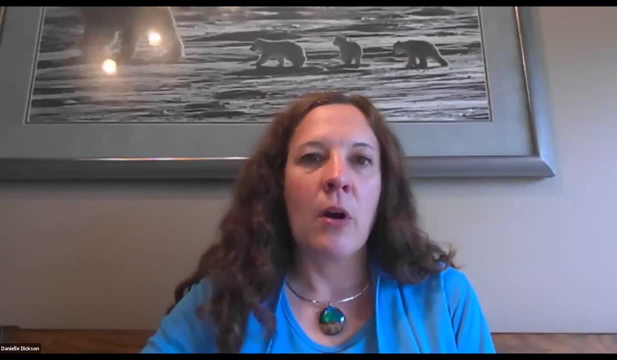 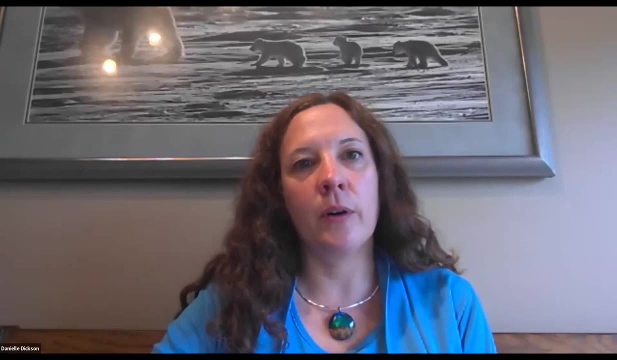 So that's kind of relevant to this program, I think, and what we're talking about today. And then we also offer a core program that provides funding on a mostly annual basis, And there is a category for oceanography and lower trophic level productivity And under there, 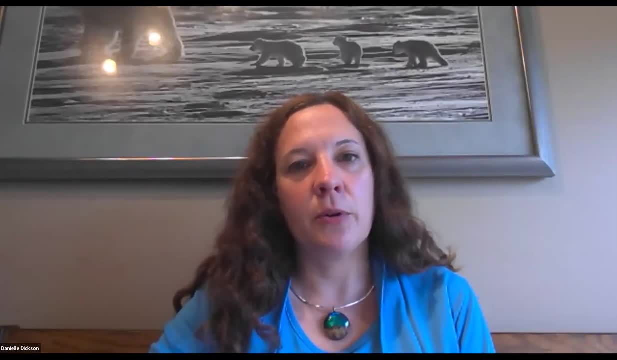 we provide funding on a more regular basis for smaller scale projects- two or three years to look at something specific. So I encourage you to look at our website And I'm happy to take questions later. Thank you so much. Thank you, Thank you, Danielle, very much. 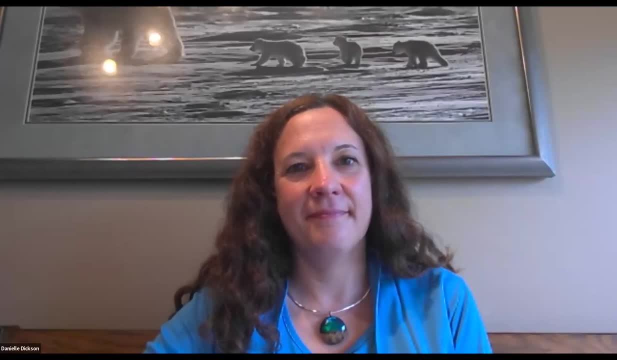 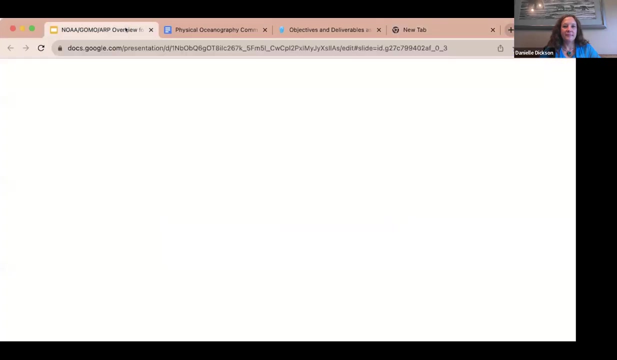 And, last but not least, we have Sandy from NOAA, Yeah thanks. So Meredith Meredith is going to show some slides. for me, This is my first time engaging with the physical oceanography community of practice, So I thought I'd give a bit of an introduction to the GOMO's Arctic Research Program. 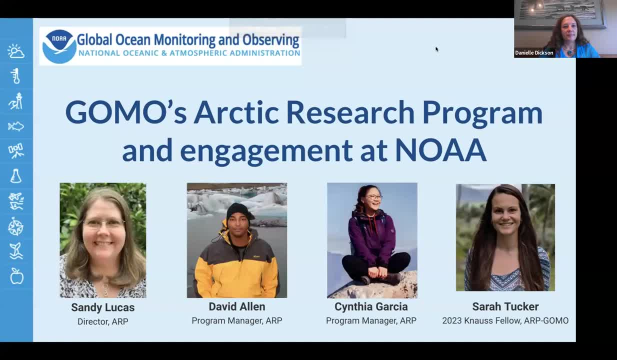 The Arctic Research Program within GOMO, the Global Ocean Monitoring and Observing Program Office. we're a smaller size program compared to others at NOAA. I'm the new director. My background is in physical oceanography and atmospheric sciences. Before coming to GOMO, I was at the climate program. 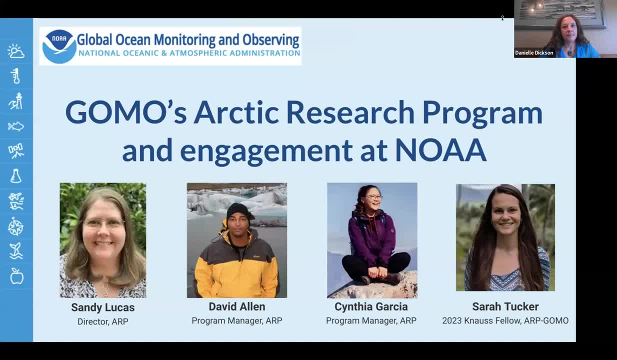 office under the climate variability and predictability program, So you may have heard my name through that side, But I came on board at the end of last year, beginning of this year and I'm still getting up to speed on a lot of things, So I'm looking forward to having a rich. 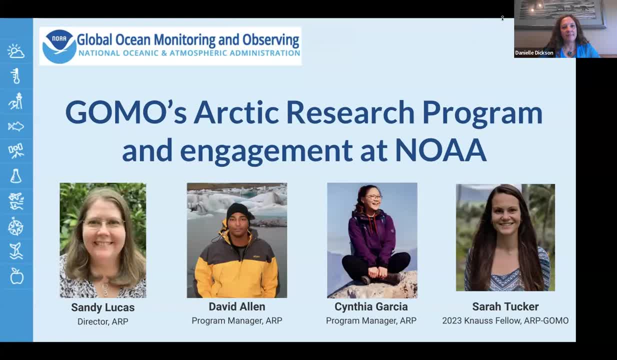 discussion today and seeing all the connections that are going on through IARPIC. My program management team are David Allen. He's the senior program manager for ARP. I'm sure you've engaged with him a lot across the different communities of practice in IARPIC. The second: 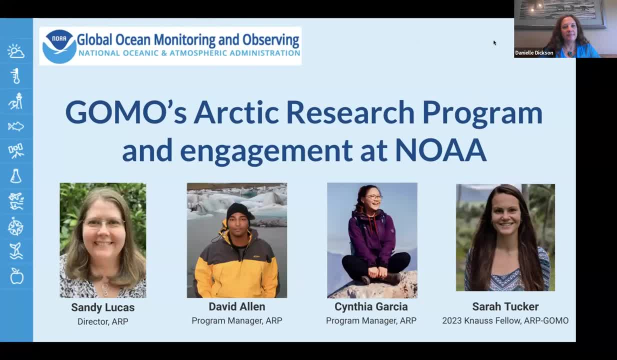 program manager newly hired on is Cindy Garcia. She's taking on some new roles this year, different from when you probably engaged with her last time. She was a Knauss fellow working with some of the community of practices in the secretariat. 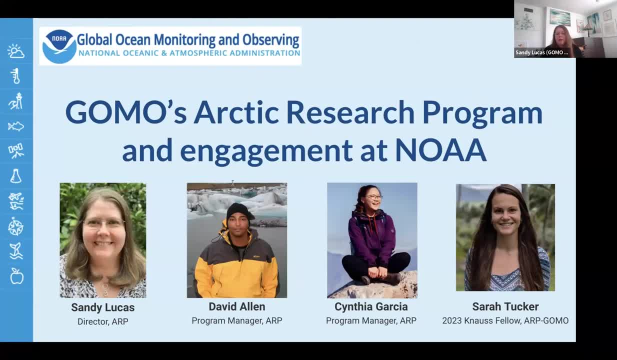 Additionally, Sarah Tucker is our Knauss fellow. She's been working with us for a long time. She's a Knauss fellow for ARP this year and she's taking on the field operations working group or community of practice, vessel matrix website and planning. So I hope you've engaged with her in. 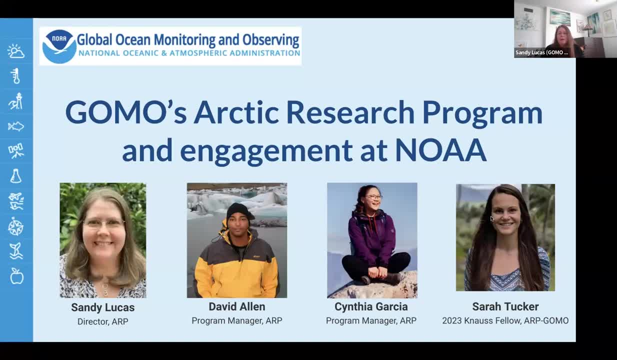 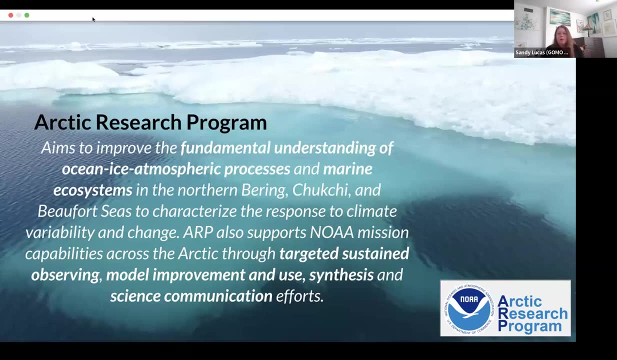 the past as well. So that's our ARP team, as I said, within GOMO Next slide- And I'll be talking not only about GOMO in the first set of slides, but also another program through the climate program office, So the Arctic Research Program. it aims to improve the fundamental. 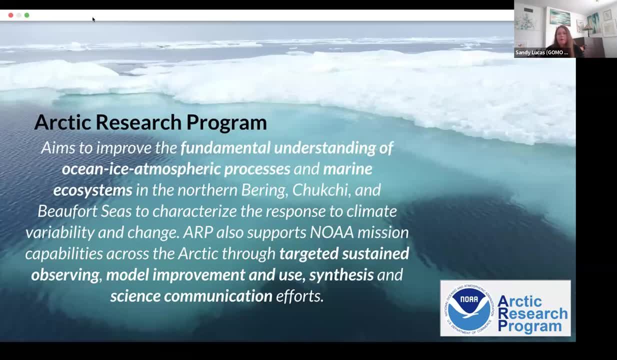 understanding of ocean ice, atmospheric processes and the marine ecosystems in the Northern Bering, Chukchi and Beaufort Seas, And this is really to characterize the response to climate variability and change. The Arctic Research Program also supports no emission. 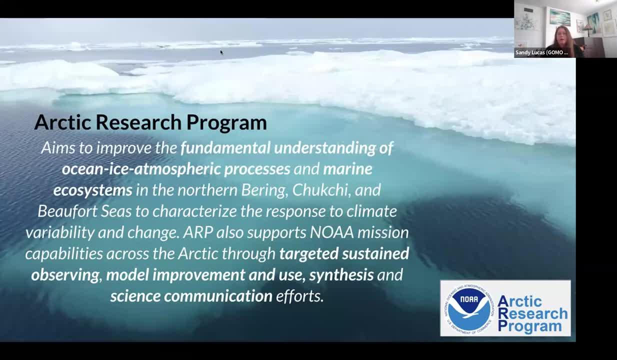 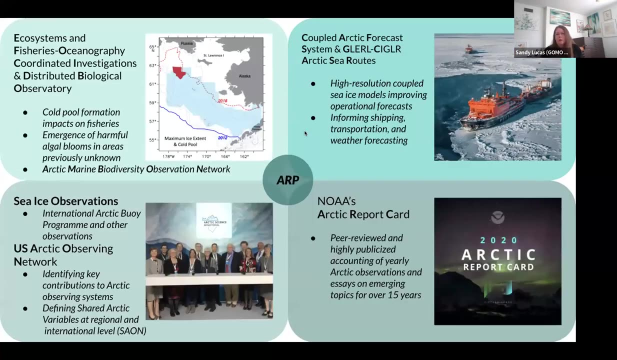 capabilities across the Arctic through our targeted and sustained observing, through the investment in model improvement and the use synthesis and science communication efforts. So next slide is showing the portfolio And this can really be broken into sort of four areas of our major investments. 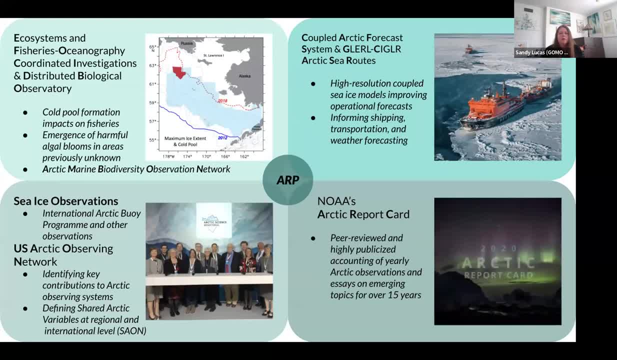 So the first is the Ecosystem and Fisheries Oceanography Coordinated Investigations. It's ECOFOCI That has both long-term observations in it, some modeling work and connections out through the fisheries decision that Danielle was recently talking about in the synthesis efforts That's. 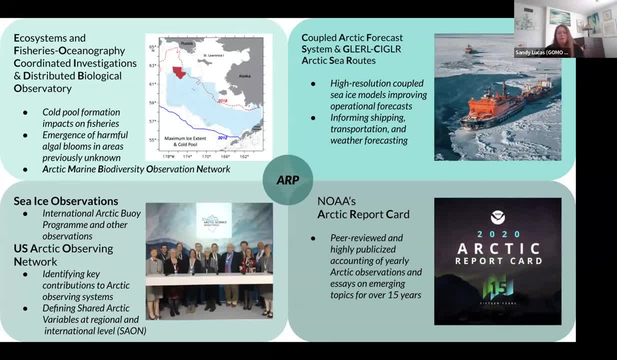 tied in hand in hand with a distribution of the Arctic Research Program. This is a large group of biological observatory. They have shared cruises and shared observation products, So they're really looking at the cold pool formation, the impacts on fisheries, changing sea ice locations. 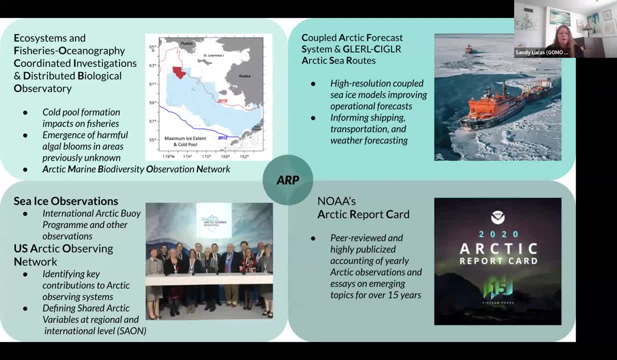 and those impacts and the emergence of harmful algal blooms in areas that were previously unknown in the recent past. And that also includes an individual project called the Arctic Marine Biodiversity Observation Network or NMOM. So the second major area under ARP is modeling. 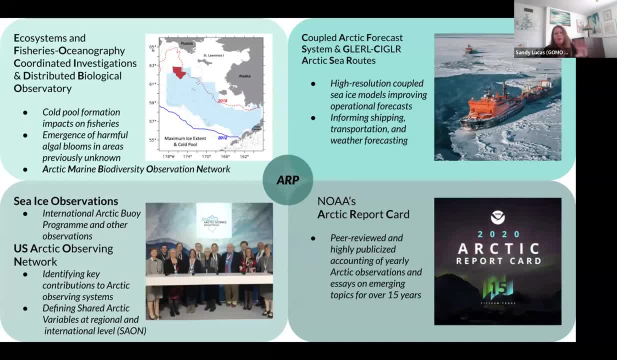 and improvements to modeling. I should say that the ecosystem and fisheries- the EcoFoci group is mainly at PMEL and at the Alaska Marine Sciences Fisheries Center And the next set is for the Arctic modeling and model improvement. The next set is for the Arctic modeling and model improvement. 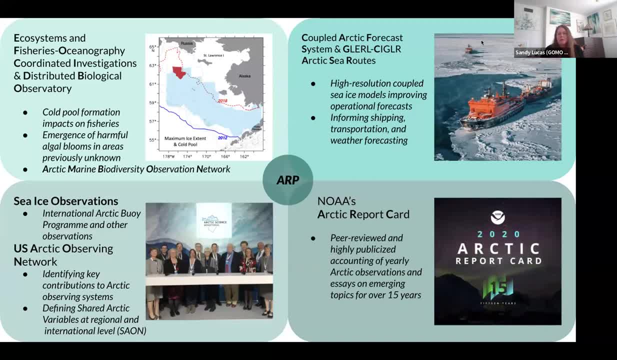 The next set is for the Arctic: modeling and model improvement. Those are through two teams. One is at the Pacific Sciences Laboratory at NOAA's PSL in Boulder, Colorado. The second is at GLERL, the Great Lakes Environmental Research Lab, in Ann Arbor, Michigan. 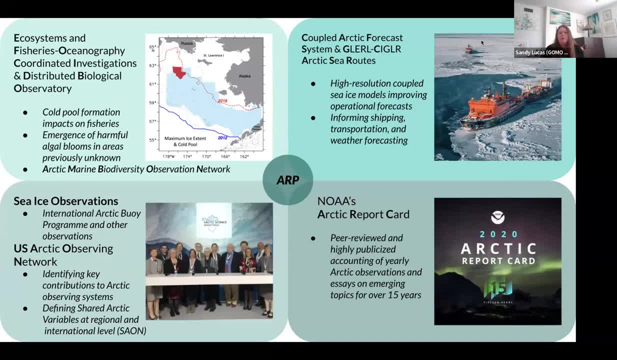 So the PMEL group has CAFs, the Coupled Arctic Forecast System, And that work is advancing quickly and transitioning in the next couple of years through to NOAA's newer UFS Unified Forecast System. So those are things that they're working on: the high-resolution coupled sea ice models. 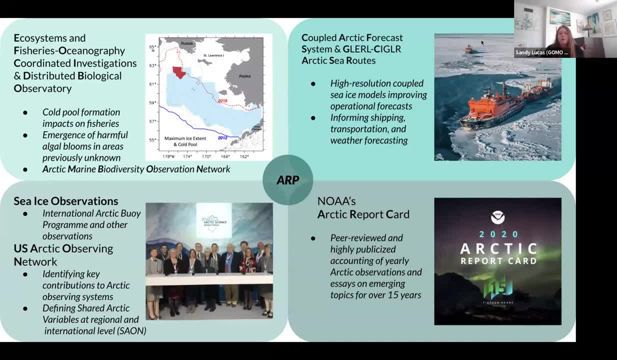 for operational forecasts And the work at GLERL is looking at the sea ice routes or the- I'm sorry- the shipping routes through the Arctic Ocean area. So that's information for shipping, transportation and weather forecasting. Another major area of the ARP portfolio are observations specifically for sea ice. We fund the coordination. 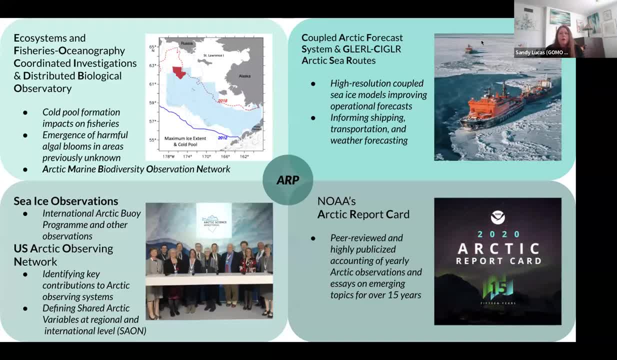 of the International Arctic Buoy Program. We also have the Sea Ice Mass Balance Buoys in the High Arctic as well, as we are the core funder for the program office and director of the US Arctic Observing Network, USAON, which is coordinated here through IARPIC. And that's identifying the 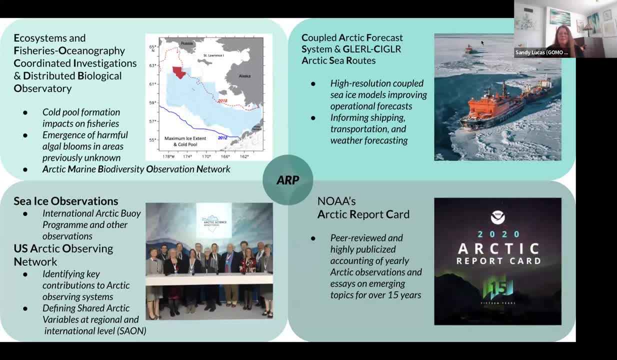 contribution. And then, last but not least, we have our communications and transitioning, all of the great Arctic science that's going on through the NOAA's Arctic Report Card. It's a peer-reviewed and highly publicized accounting each year of the yearly change based on Arctic science, And we're also working on the Arctic. 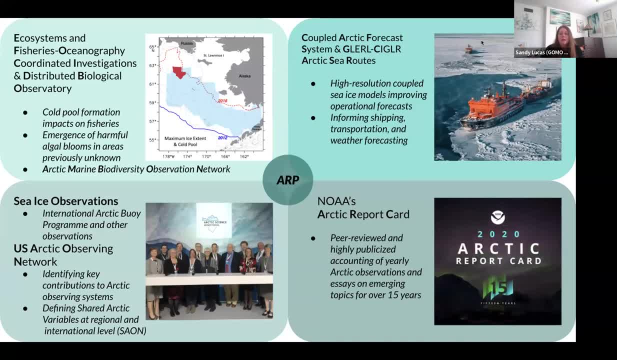 Observing, And it comes out as a series of essays and topics that have three areas. One is a core set of variables that are looked at year over year. The second area is emerging topics, And then the last area is updates on topics that get refreshed every couple of years. So that's frostbites, indicators and the 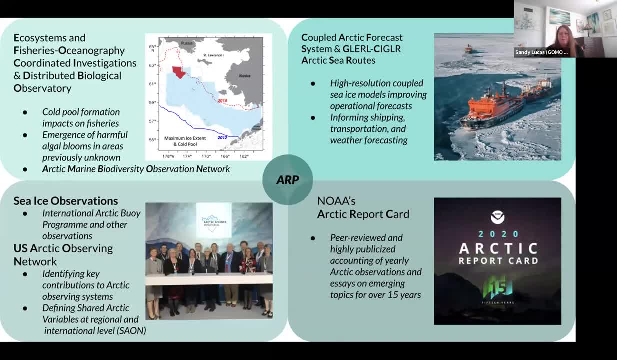 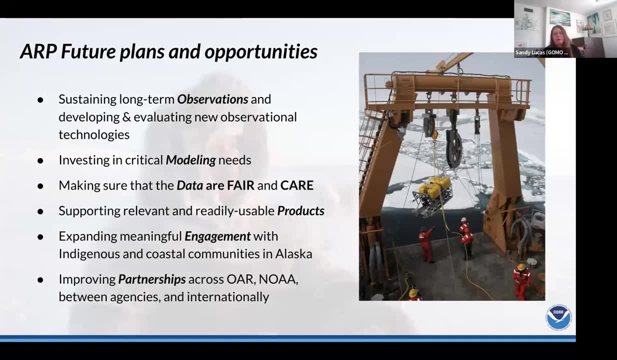 Consistence Index. So next slide. So you asked about what, where our future opportunities and plans are for Arctic Research Program. This is specific to my program. We're interested in sustaining the long term observations and developing, evaluating new observational techniques, as as the budget allows. 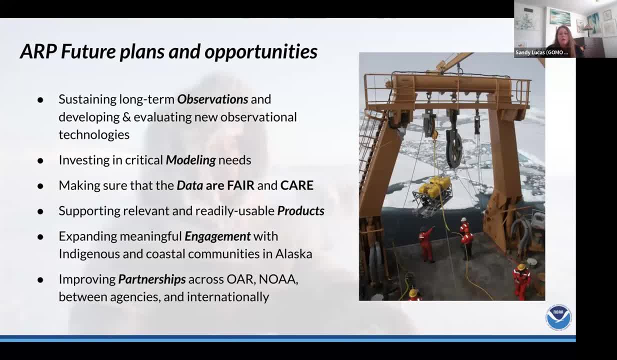 We're investing in modeling needs, both with a focus on NOAA's missions, but also supporting the societal connections through transportation and needs of the Alaskan and Arctic region. The next is that we are making sure that our data is helping to support fair and care practices. We've recently expanded the ARP website to include data. 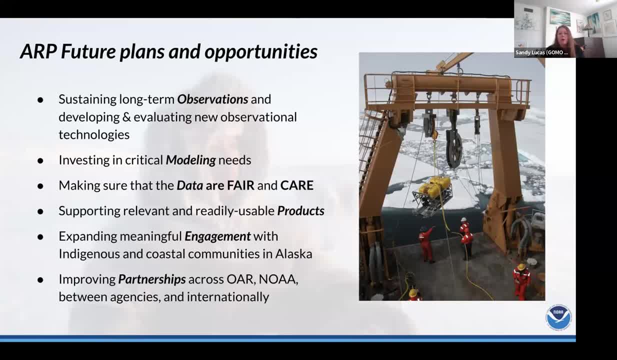 landing pages, which makes a more accessible path to the data that the Arctic Research Program is developing, a path so that people can find our principal investigators' data more quickly. We're also supporting relevant and ready-to-use products. We're expanding our meaningful 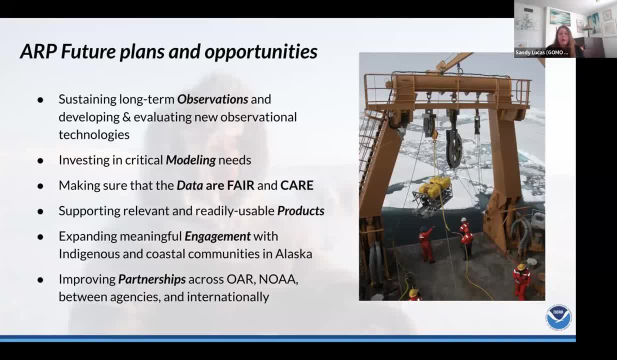 engagement with Indigenous and coastal communities in Alaska. We have an opportunity to engage, through our partners at NOS, with several community groups and I can give you details of that offline. The last is improving our partnerships both within NOAA across the United States and across the United States. We're also developing a path to 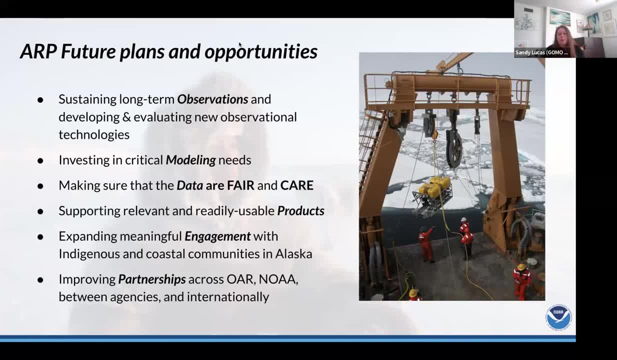 make sure that our partners at NOS and across OAR, NOAA and between our agencies, like through IARPIC, plus internationally through our other groups. So next slide, This is the transitioning to the Climate Program Office, which is a different program office from. 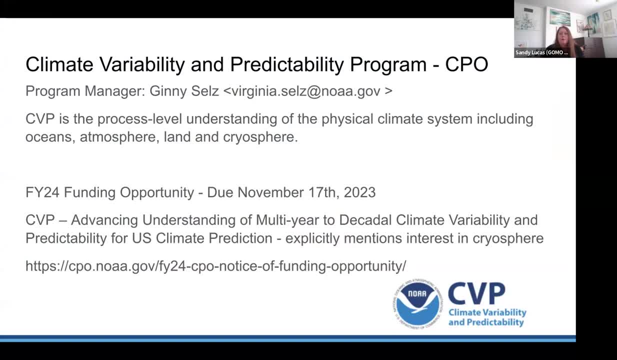 where I'm sitting, The Climate Program Office has a program called the Climate Variability and Predictability Program. The program manager there is Ginny Seltz. That's her email And I wanted to alert this group that there is a current call for proposals. 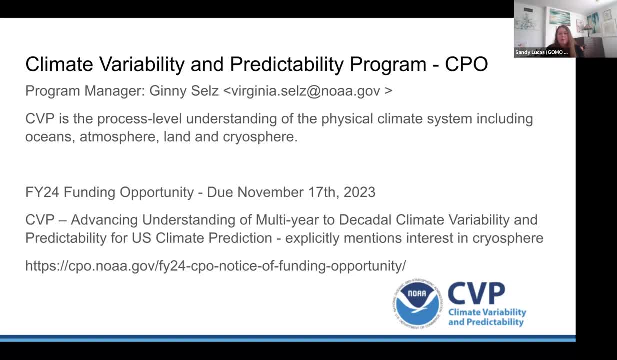 and the climate variability and predictability program is the process-level understanding of the physical climate system. So that includes ocean, atmosphere, land and cryosphere, So fairly broad. But I wanted to highlight that they do have a call for proposals for fiscal year 24.. 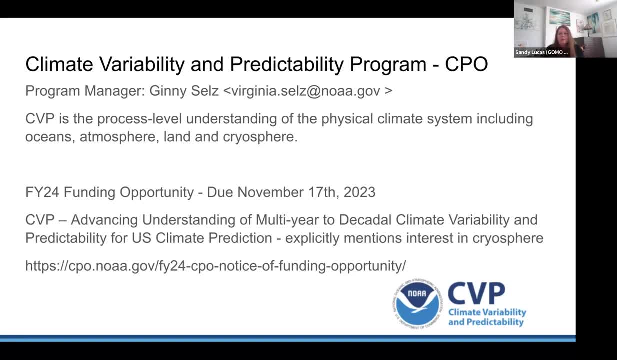 It's due in mid-November. The date for the letters of intent have already passed, but you could reach out to Ginny if you have a project that you think that might be appropriate. The title on it is Advancing Understanding of Multi-Year to Decadal Climate Variability and. 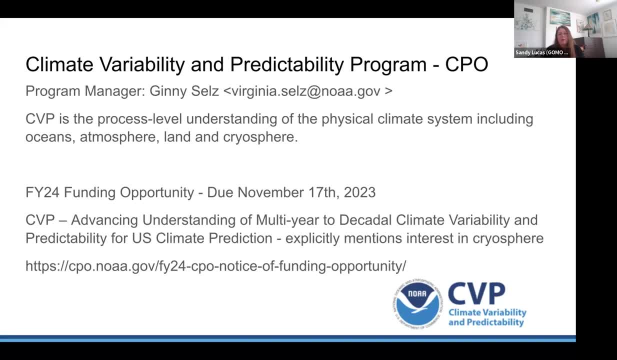 Predictability for the US Climate Prediction, And I highlight this because it does explicitly, amongst the other key processes, call for a cryosphere, And the link to that funding opportunity is there. I'm going to circle back a little bit Right now. the Arctic Research Program. 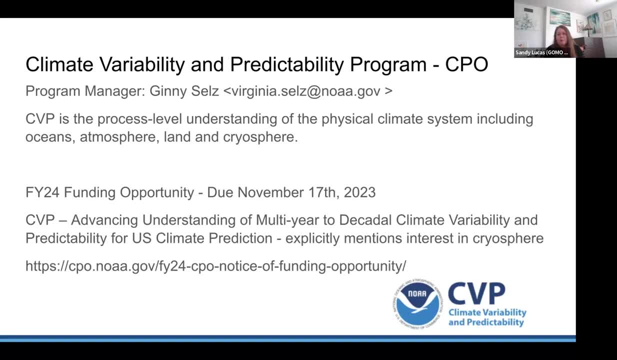 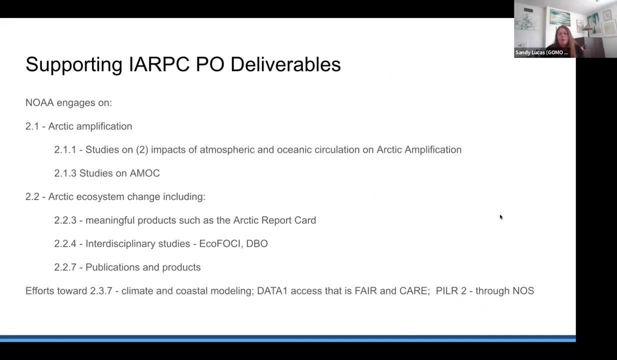 does not have any open calls for proposals. We mainly do core and direct funded funding, But hopefully in the future that will change as funding becomes available. That's of interest to us. So next slide: I wanted to do just a crosswalk quickly on supporting the IARPC PO deliverables. 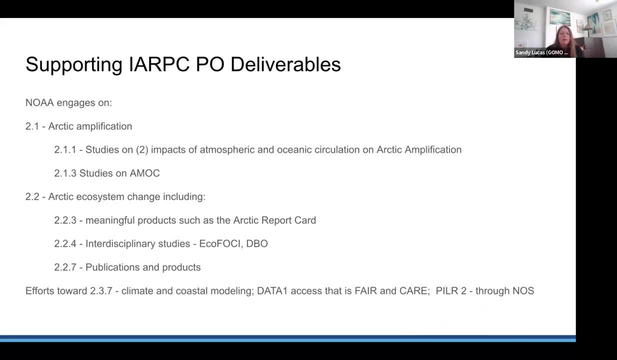 So Arctic engages in work for Arctic amplification. So specifically on 2.1.1, we have studies that are the impacts of atmospheric and oceanic circulation on Arctic amplification and on connections to lower latitudes. So that's something that we've been working on for a long time. 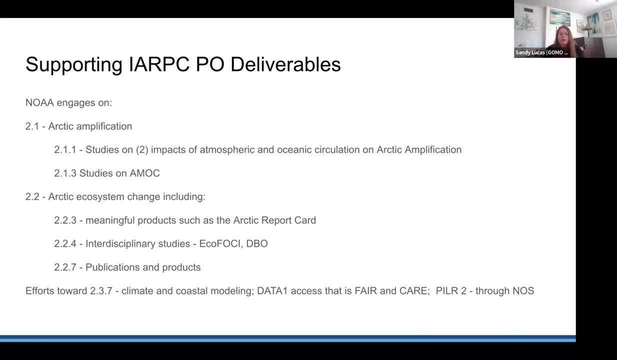 So that's something that we've been working on for a long time. So that's something that we've been working on for a long time. We have a large suite of projects that are on studies of AMOC. We also support 2.2, the Arctic. 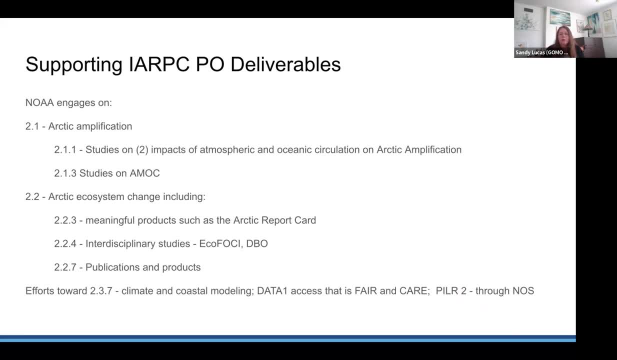 ecosystem change, and that includes products, meaningful products for 2.2.3, such as the Arctic report card. We also have the interdisciplinary studies under 2.2.4 for ECOFOSAI and DBO, Just calling out two examples. there's many more, And we also have a suite of public. 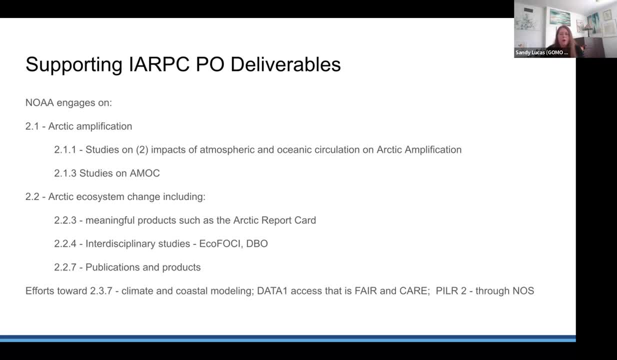 publications and products through many of our service delivery and through our core ARP projects. We also have efforts towards climate and coastal modeling, observing improving those models under 237.. And of course, we align with data. one, the access to fair and care. plus, we support pillar. 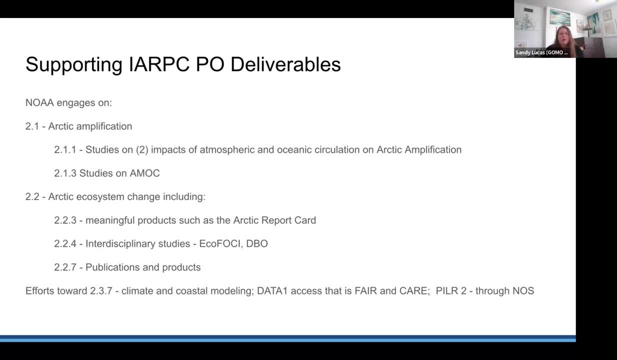 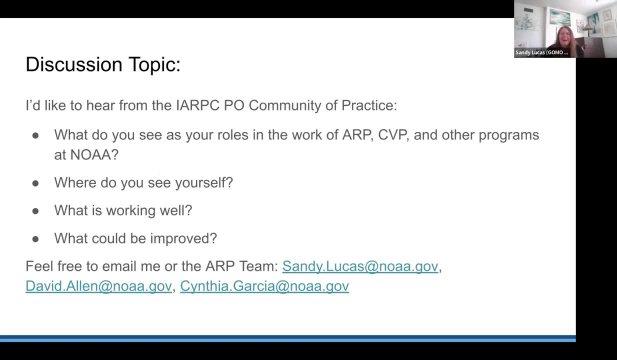 two with engagements through communities, specifically through NOS. Next slide: I think it's maybe strategic that I'm going last here because I put a slide in for discussion topics. I'm new to the IARPIC community, the physical oceanography group, as well. 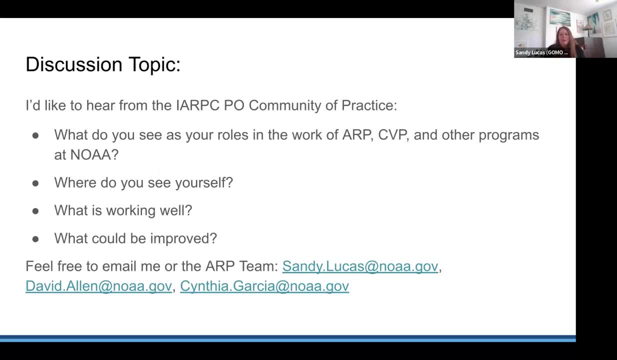 And I'd really like to kick it off with what do you, as our community, see your roles in on the work for ARP, CBP and the other programs at NOAA? Where do you see yourself? Where do you see the community at large? 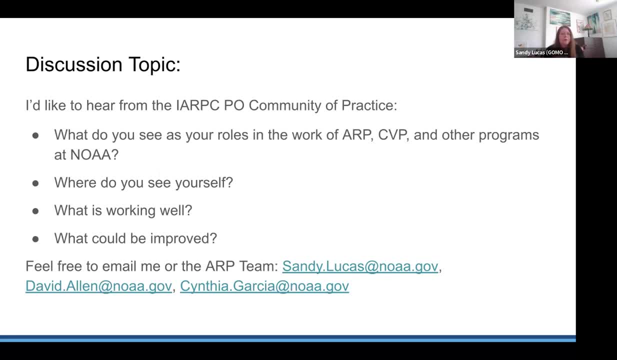 What's working well, What could be improved, And if you don't have time or if that's not of interest for the co-chairs here, feel free to email me or the ARP team. Our emails are there. Look forward to engaging. 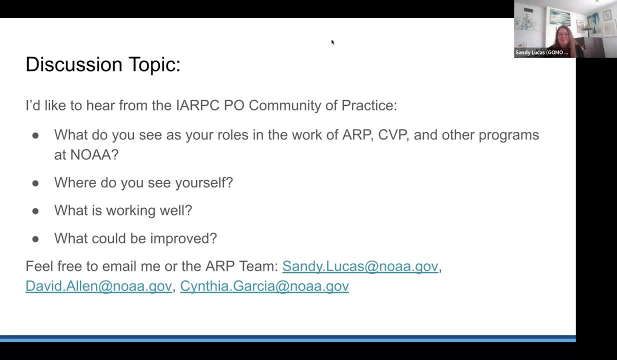 Thanks everyone, Thank you, Thank you, Sandy, And thank you everybody else for your talks. I think we are opening the floor to anybody who has questions. I would take advantage of me being the first one to speak to ask a question, actually. 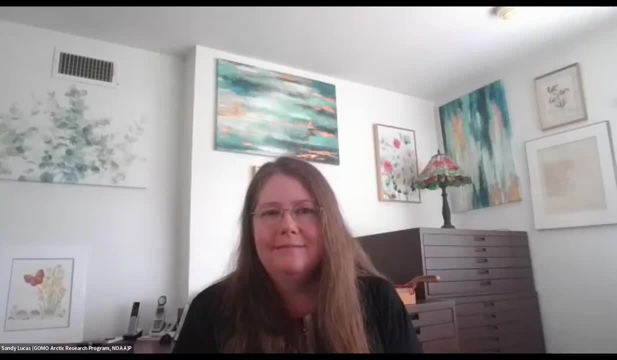 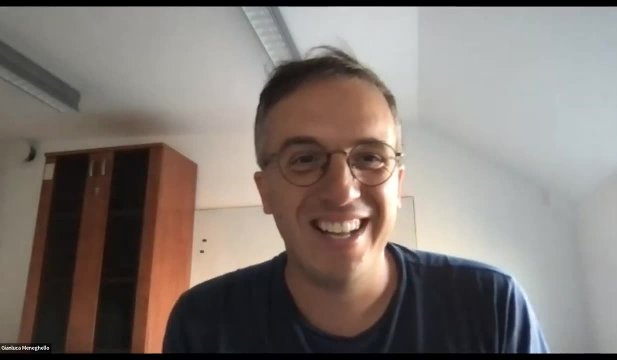 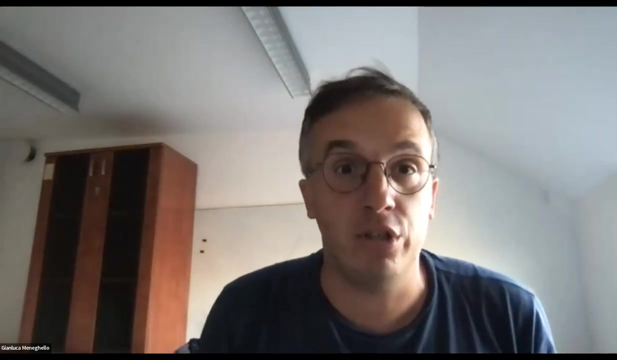 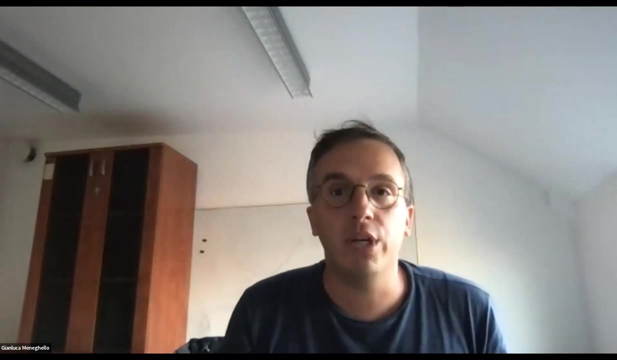 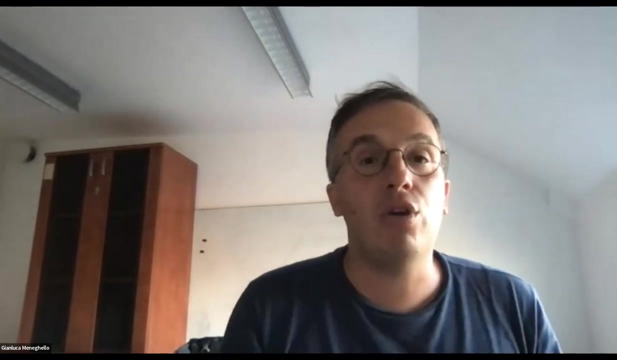 if I can, You all mentioned a lot of the observation and observational systems and the sustained observations, And one question for me is: as a physical visionographer, we would like to use them as much as possible. You have a big picture on what is done and what are we doing and how well are we using. 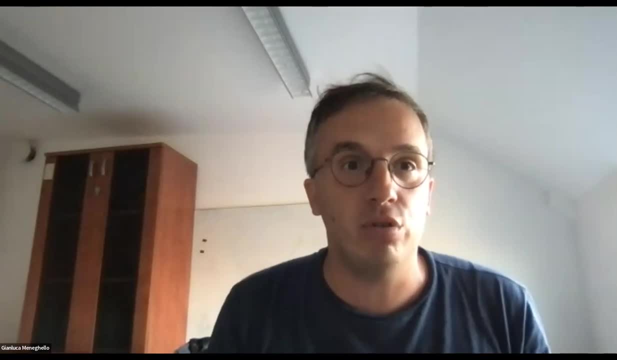 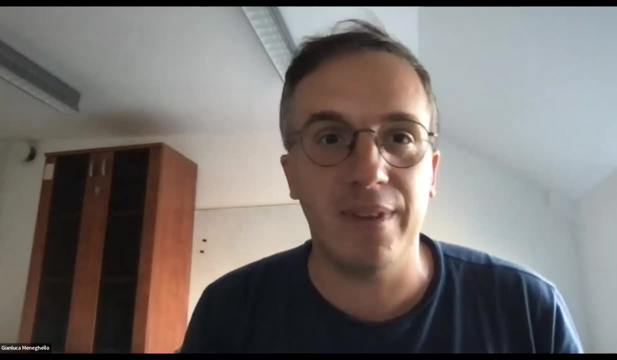 the observation. Do you have any feedback on that? Do you think there are gaps that we should look into about using this observation to inform our studies, Or do you think we're actually doing a good job? I think we are open for criticism, in case. 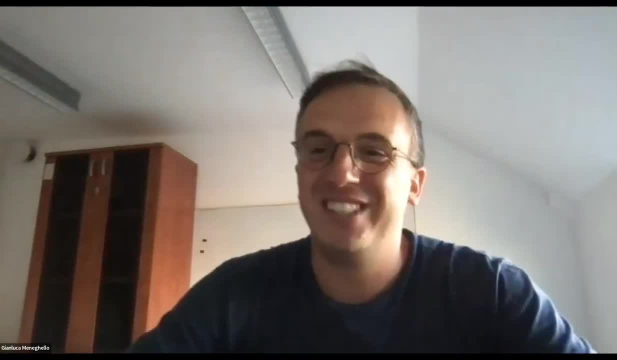 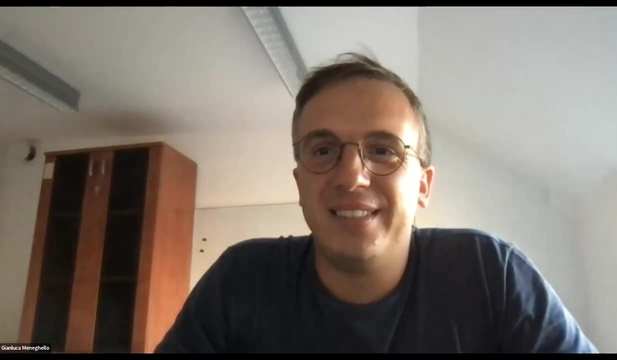 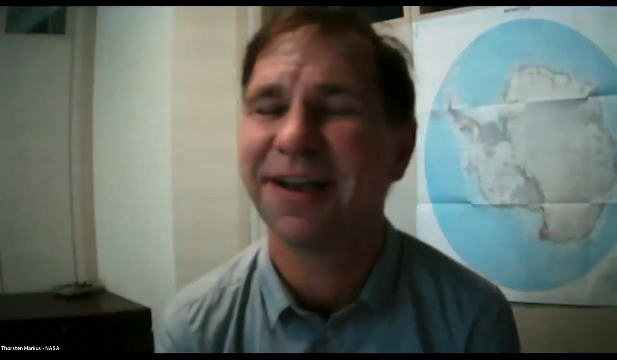 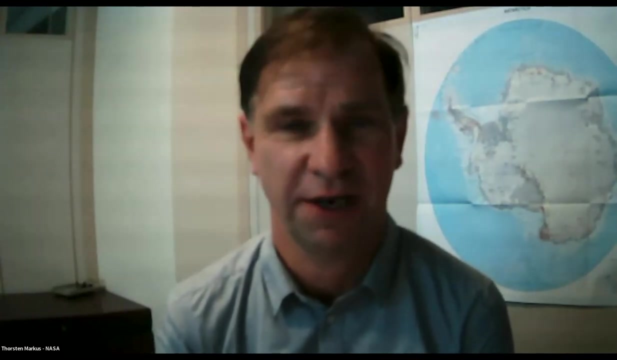 I don't know who wants to start, but that was my question. We are doing a No, no, It's funny, It feels to me. it's a question for the community because I would be really interested in hearing: are those data useful? 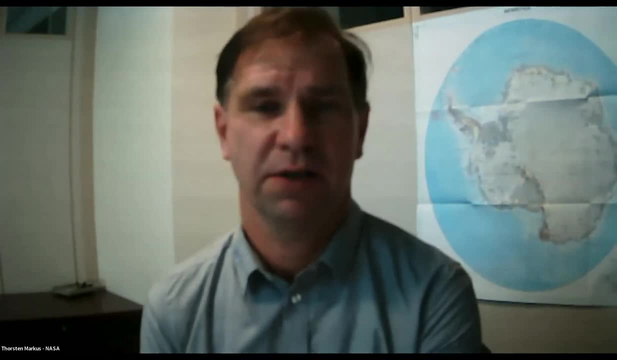 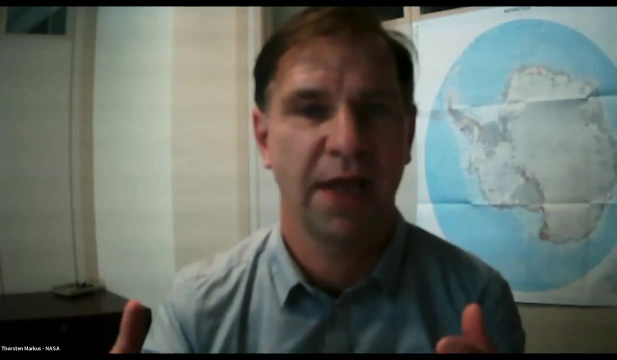 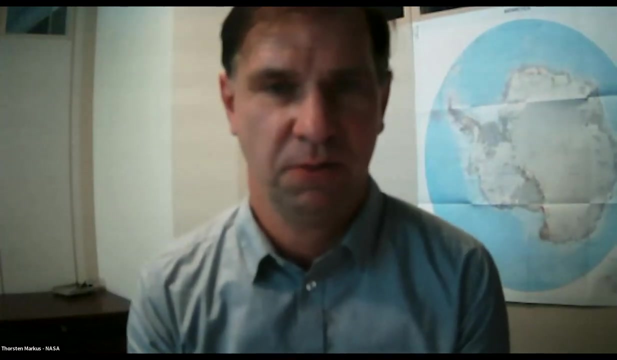 What data are especially useful? What are the data needs? When we did the year of Arctic prediction, I was marginally involved, but it was a discussion about what do we need to do? What observations do we need to have? This was all a short scale. 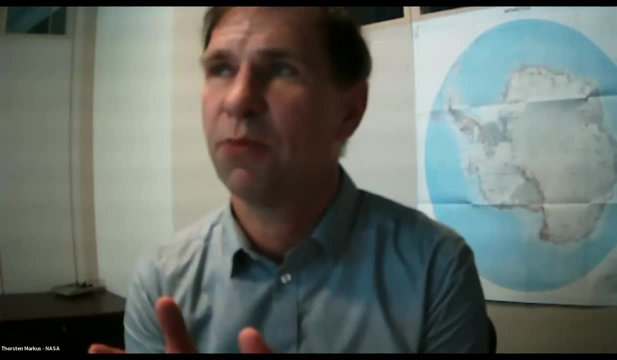 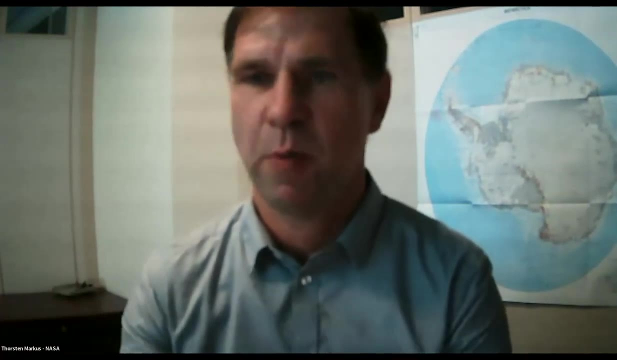 It was weather scale. York was weather scale, But it was great to have that discussion with the community: what data are most critically needed And one outcome. One of the things I've been talking with people from ECMWF was near surface winds. 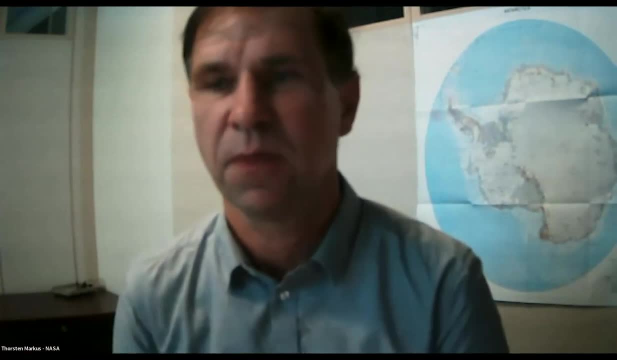 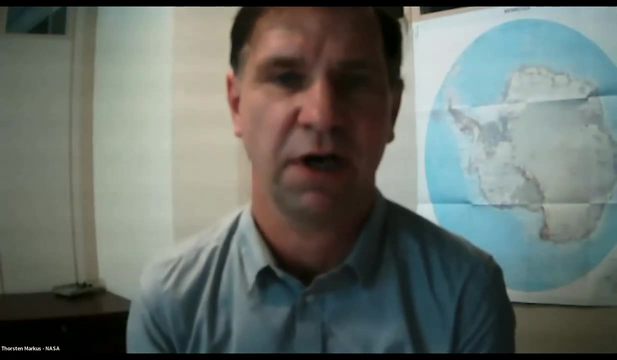 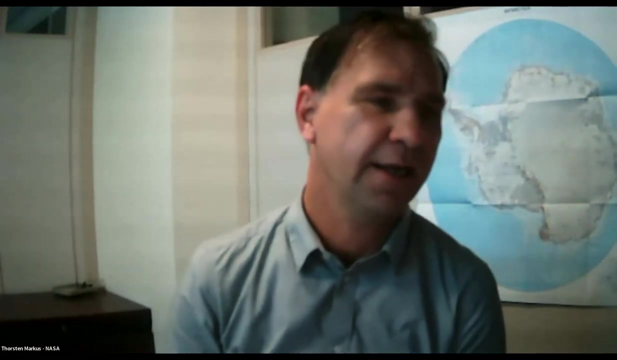 It's so difficult, It's so difficult to observe And you know, as you know, it affects sea ice draft tremendously. If the sea ice, if the near surface winds are wrong, your best model sea ice reality, doesn't help if the forcing is wrong. 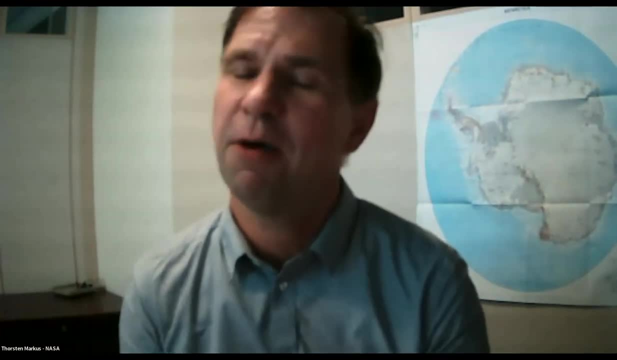 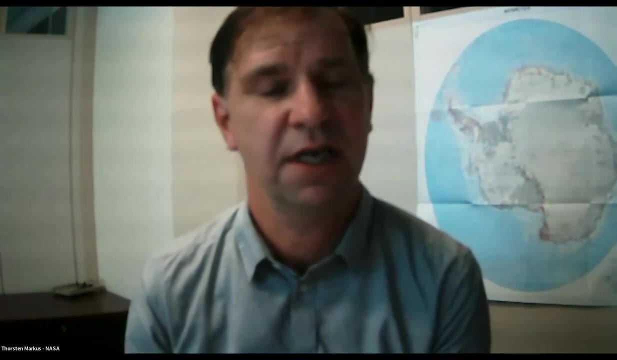 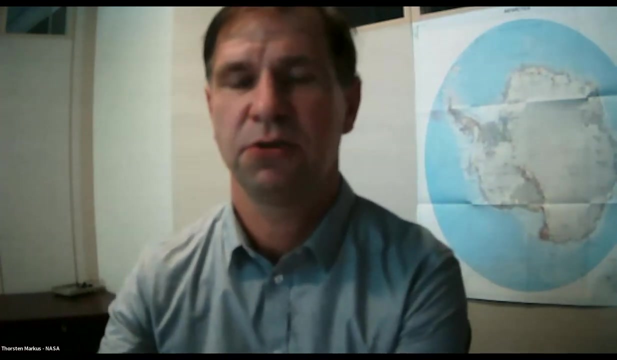 And so that's something, you know, I'm very interested in And we have, you know, a call out for missions, We have mission proposals, And near surface winds is actually an observable identified by the Decadal Survey from the National Academies. to hey, can we do something you know about near surface winds? 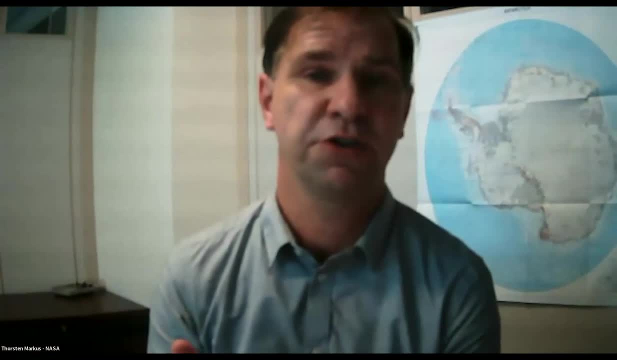 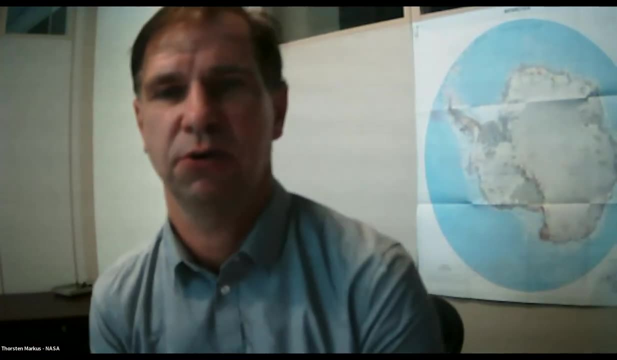 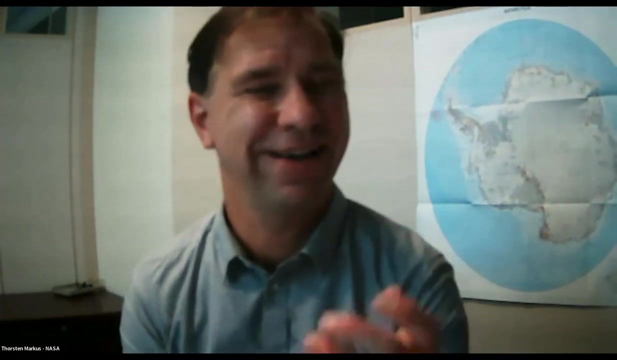 So I'm just throwing out this as an example, because I would be really interested in hearing: what do you need? And we know where our data took, course, you know in terms of resolution, in terms of temporal resolution as well. So I think it's an excellent question, but I was going to right throw it back to you. 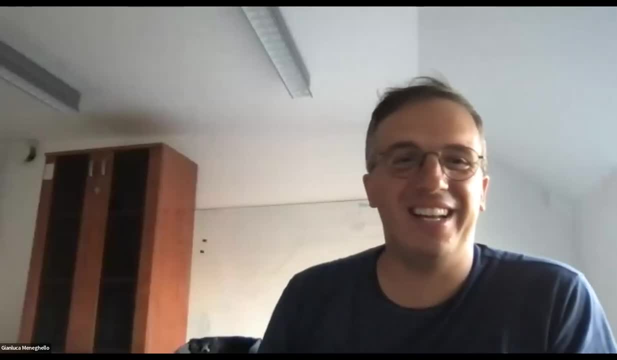 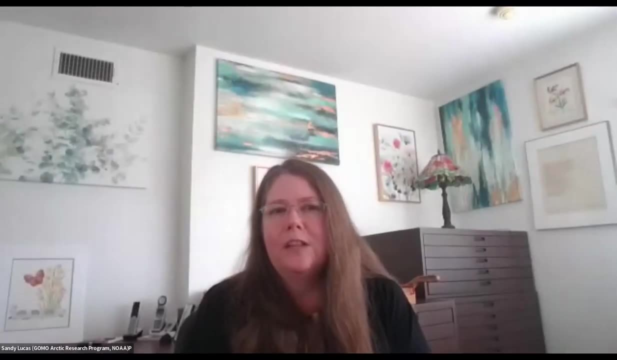 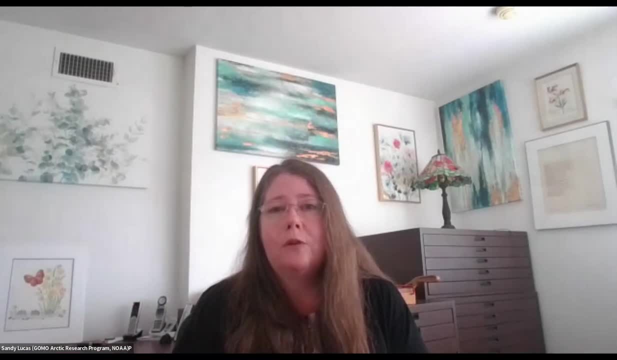 me, for instance, about the data from the IDP, and also I've heard feedback from all the time that it's for, you know, large scale models. it's really difficult to ingest point measurements And therefore it's not worth the time and effort to try to even take that on. 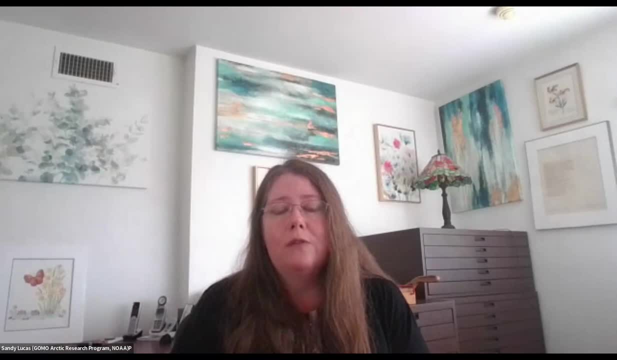 But I also hear the flip side, which is how can you model something if you've never observed it or not observing it well, in a high quality? So it's a it's a chicken and egg problem, but if you but getting a set of requirements, 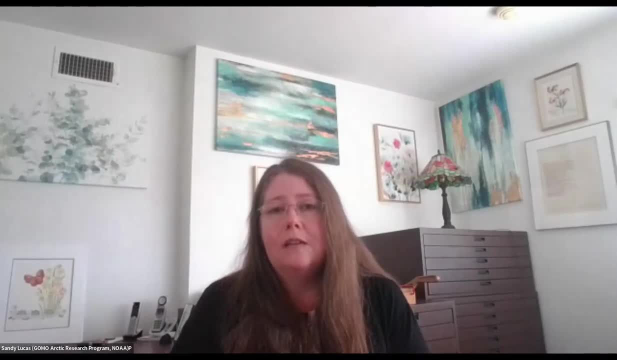 and emissions. you know the, the, the, the, the, the data. you know data the data is. you know directions and needs from the community. can be very powerful in driving the direction of the community to really help support this area. And I know that Arctic is not an emerging 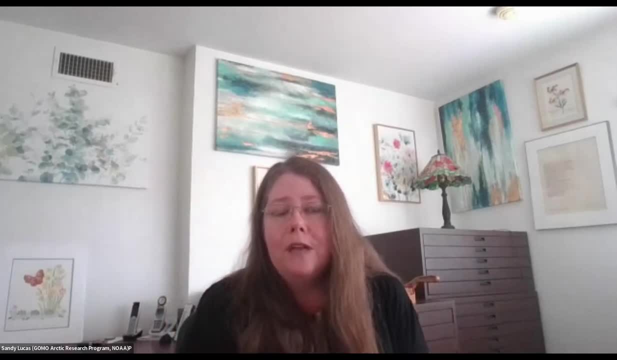 research topic. However, it oftentimes feels like it keeps re-emerging year over year as hot topics come up. So I feel right now that Arctic is going to be getting a lot of focus, if not, you know, focus in the rapid changes that are happening and the impacts that are. 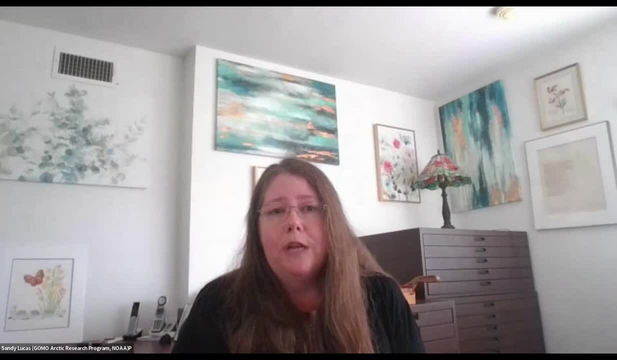 really beginning to come clear as the rapid changes are beginning to set in. So I think we need to be at the ready to understand our sustained observing networks And I think we need to be at the ready to take on some of that maybe heavy lift of talking about what? 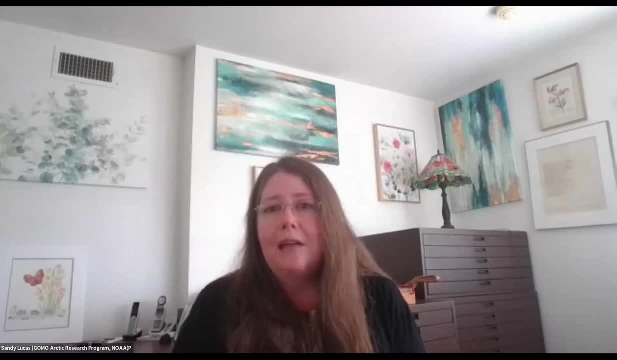 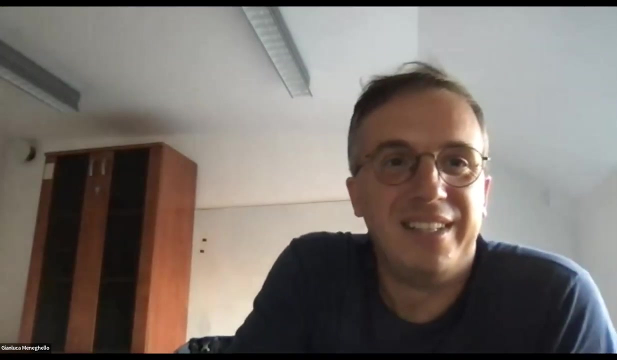 not only talking about, but producing the answers for what are the needs for observing in the Arctic and Alaskan waters at large. So looking forward to engaging Any comments from the participants. Hubert, Yeah, I mean, it's clear that the Arctic is really 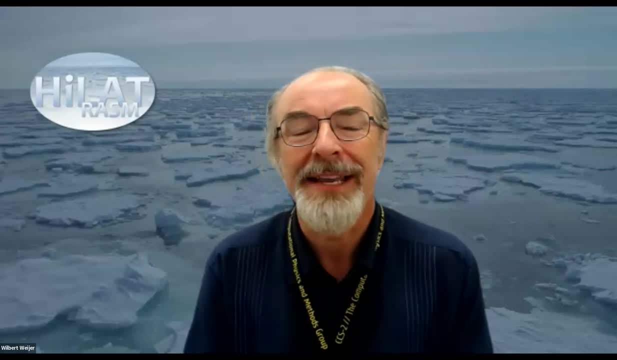 kind of underrepresented right in the observation space. I mean it's really hard to get, at least for the physical oceanography part. it's really hard to get satellite observations, of course, in these ice-covered regions And the Argo network doesn't really work there. 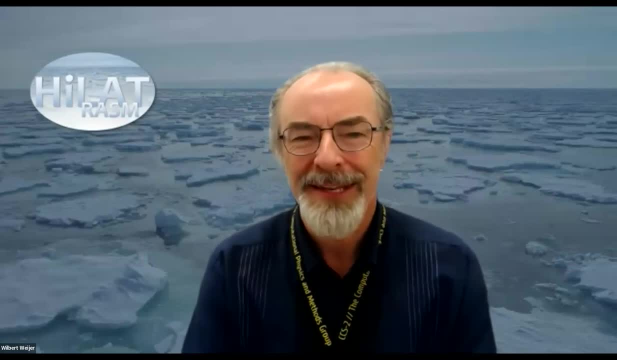 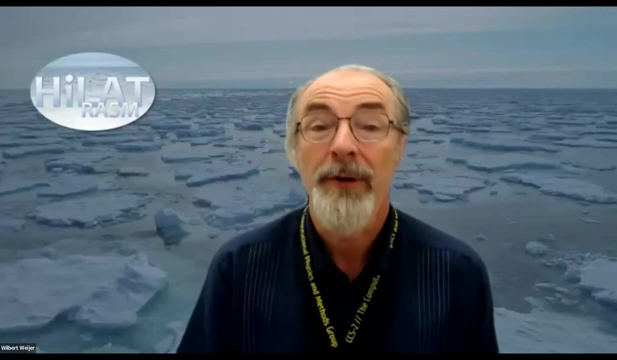 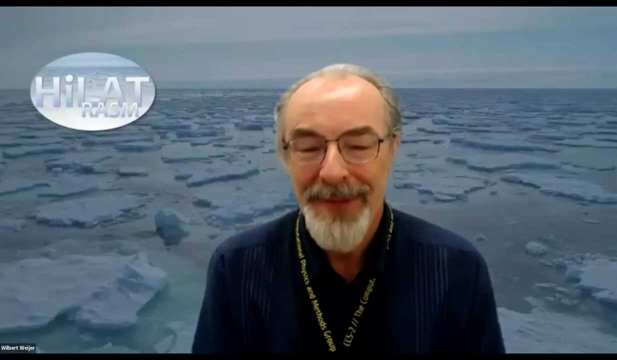 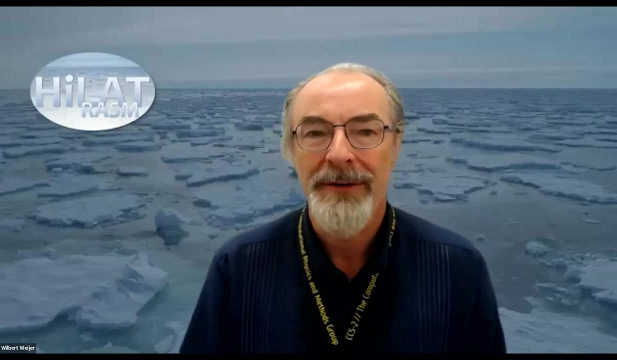 So there is a very significant data gap in the Arctic compared to the number and the techniques of observation that are available for the rest of the ocean. basically, So yeah, from a modeling perspective, I would definitely be interested to hear opinions about what other technologies can be used to. 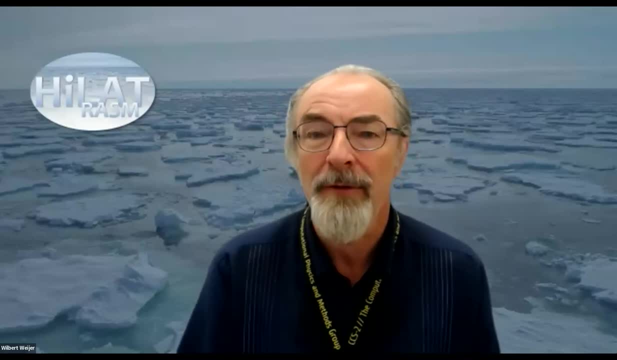 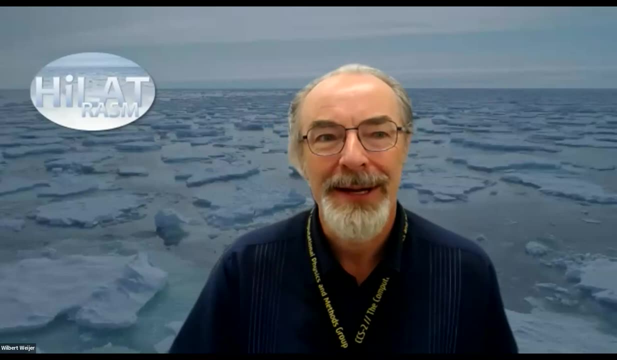 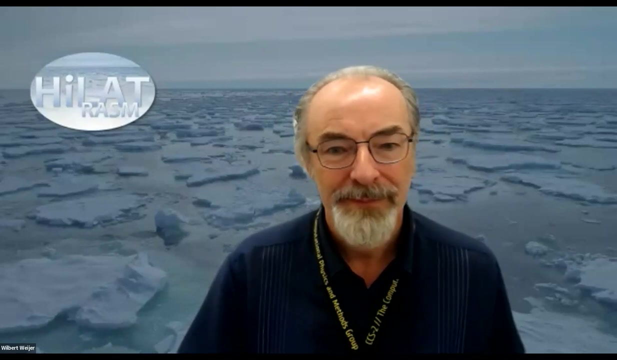 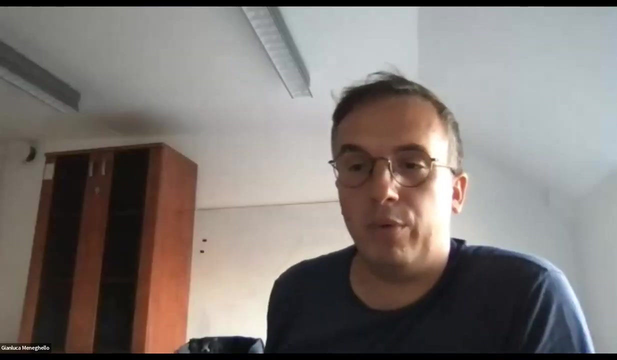 observe Arctic and Arctic Ocean And, of course, isosceles. profilers are one option, But it's very sparse, of course. So very interested to hear more about this from the rest of the community. One question maybe that would be, I mean, comes to mind to me- is what the best way to 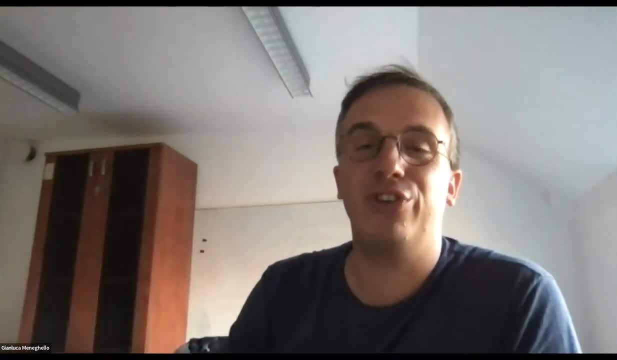 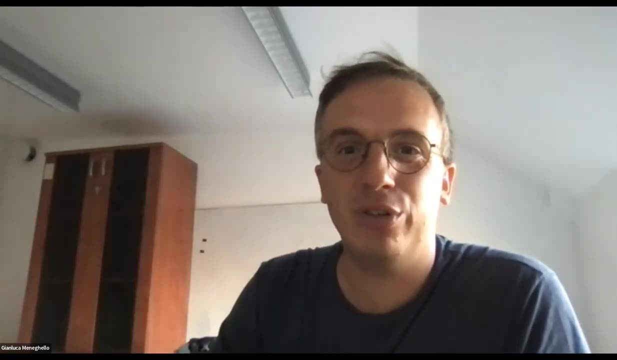 interact to somehow submit our requests to physical oceanographers? Is it just simply get in touch with you and have a phone call Or, which is, I think, very good way, Or is there ways to participate to bigger projects or calls to? I think everybody would be interested in knowing how to better contribute to. 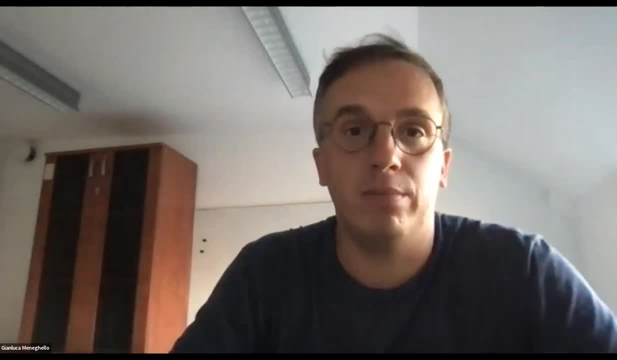 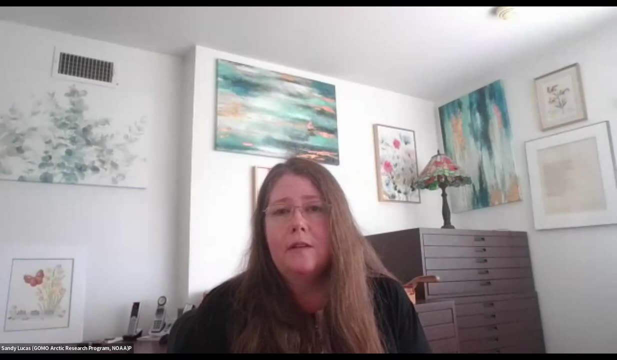 this effort to coordinate, Especially as a coordination problem? Well again, I'm new to IRFIC, so maybe this is my question to you as co-chairs: Does IRFx- physical oceanography community of practice- develop and write recommendations for future work, such as the observing needs? 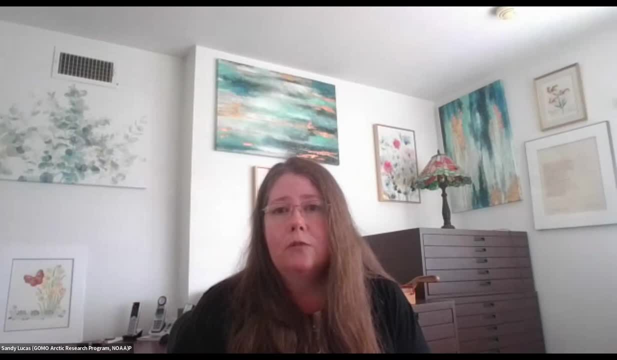 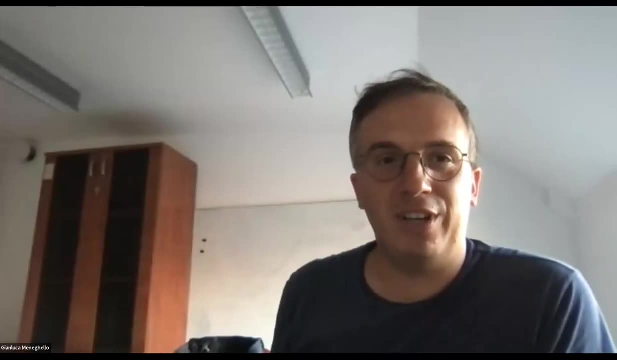 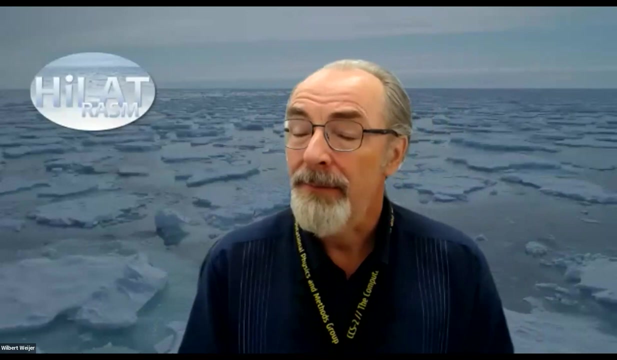 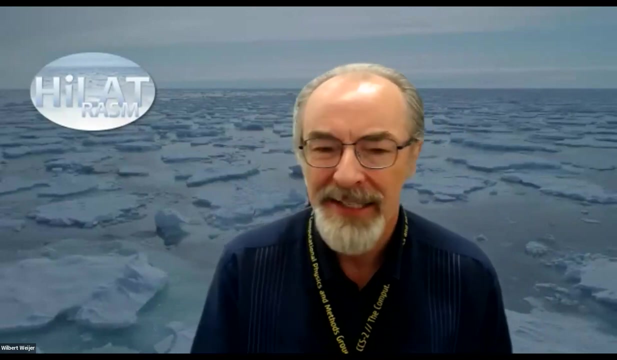 Are you making recommendations to the agencies through your groups? I will leave this one to Wilbert. She has been here for longer. I guess we have not. Of course, there is this the month foundational activity that I think David Allen is co-leading that. 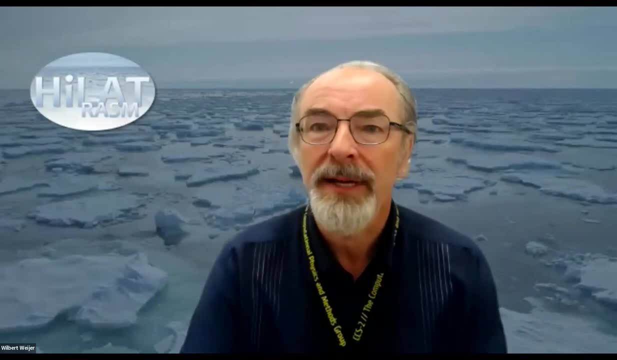 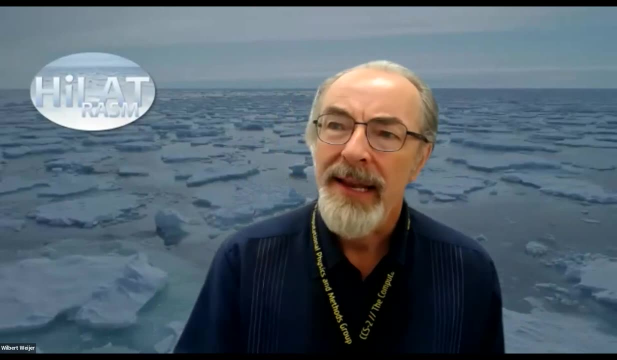 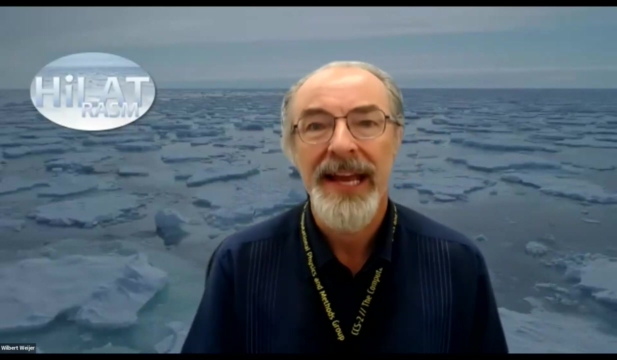 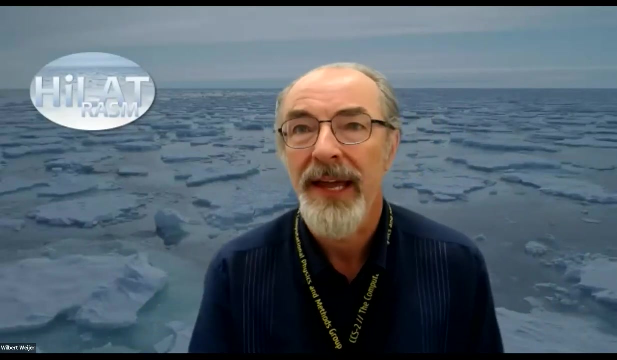 So maybe that is something that we as the physical oceanography community should be more active in, in trying to make those kind of recommendations. I noted that the US Climber Summit that we had a couple of months ago in Seattle, this topic about data sparsity in the Arctic came up and with some co-leads of the POS panel, 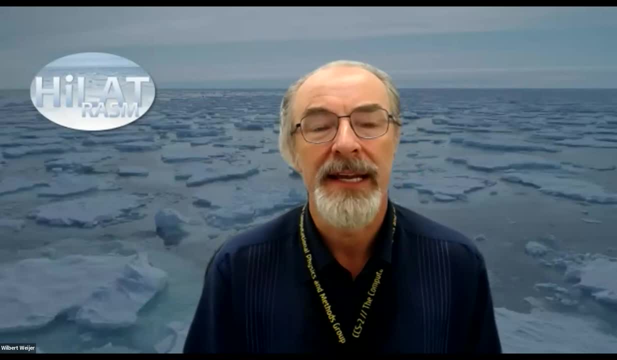 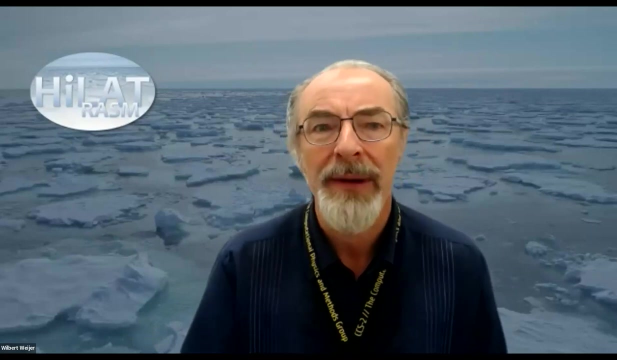 Dimitri Dikoskoi in particular. we are kind of interested in developing maybe a workshop to address this problem head on, and this might be a good forum actually to come up with maybe a kind of white paper or set of recommendations for funding agencies on how we can address this topic in more active terms than we have been able to do in with this IRFx framework. 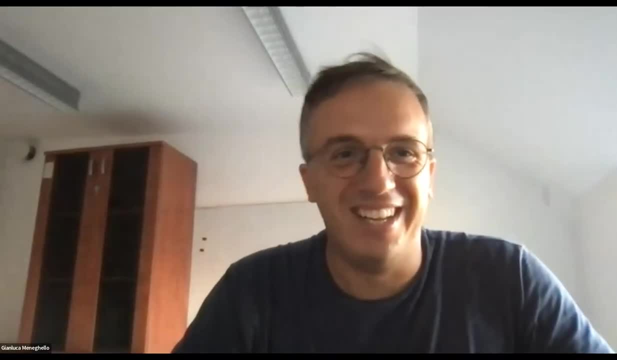 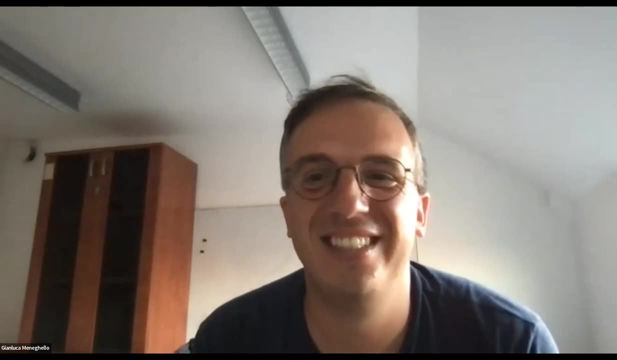 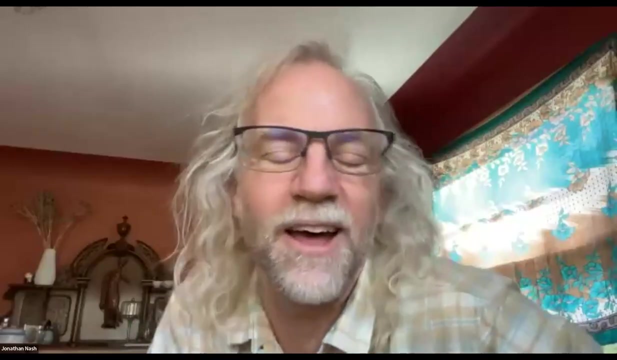 I really feel I've been talking too much, so if there is anybody else, I don't think we have time for any more questions. but if there are any other questions, please feel free to put them in the Q&A box and we will get to them as soon as we get to the end of the session. 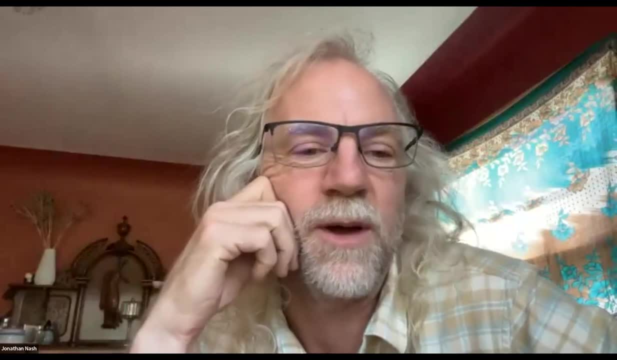 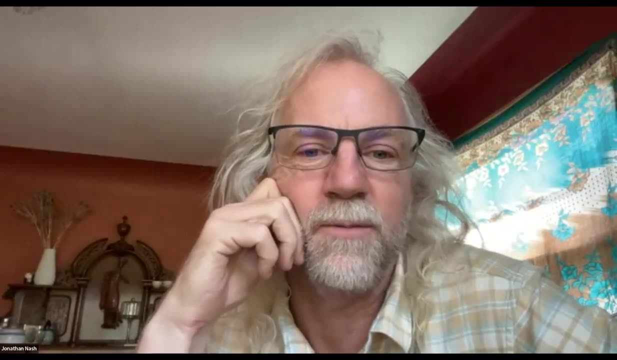 Thank you. Thank you, Jonathan has appeared. Well, yeah, I'll just. I just want I'd have to go to another meeting, but I just wanted to thank you actually for putting this on, and especially on behalf of the, like the more junior, early career researchers. I think this is a really useful thing to start this conversation and sort of continue it going to. 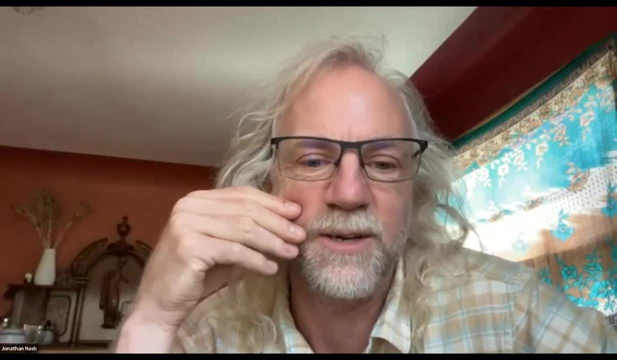 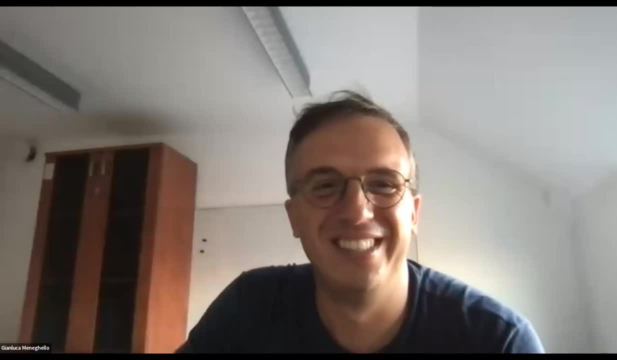 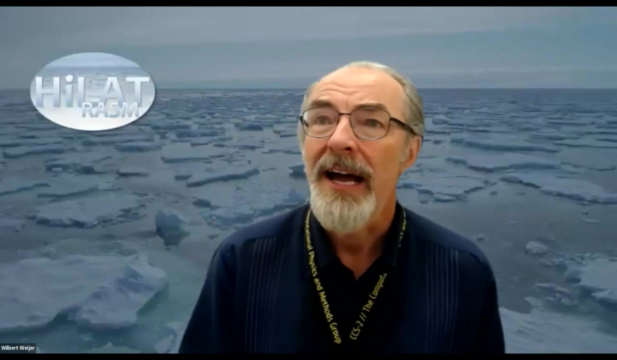 Thank you. Thank you very much. Thank you very much. Was that? your hand is up again? is it from before or No? this is new. I don't want to knock the time either. I do have a question for for Thorsten, and it may not be in a program with them in your portfolio, but I was wondering if you could say a few words about the NASA Arctic colors project, that interdisciplinary Arctic. 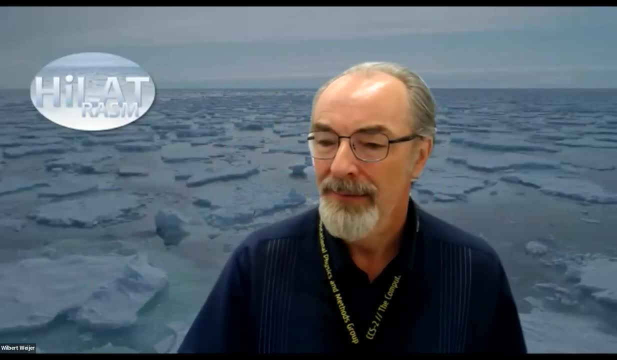 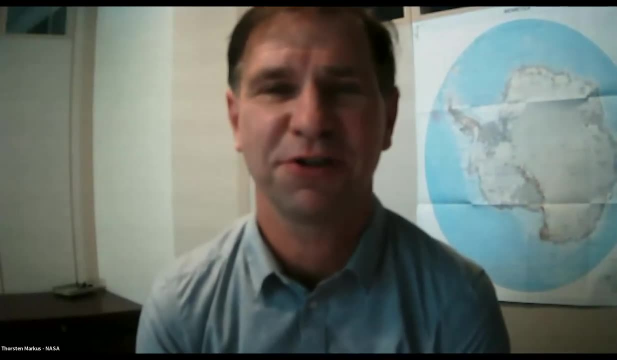 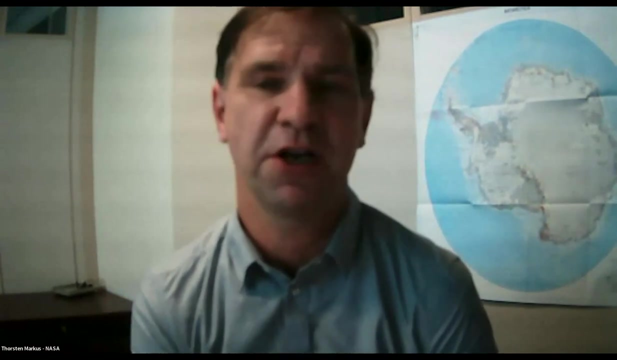 um, arctic coastal activity. you know, totally fair question. um, i, you know i don't want to talk too much about it because i don't know too much about it. you know, you know fair enough, that's. that's spinning up. um, you know, as many as you may know, by laura lorenzoni, who runs the ocean biology and 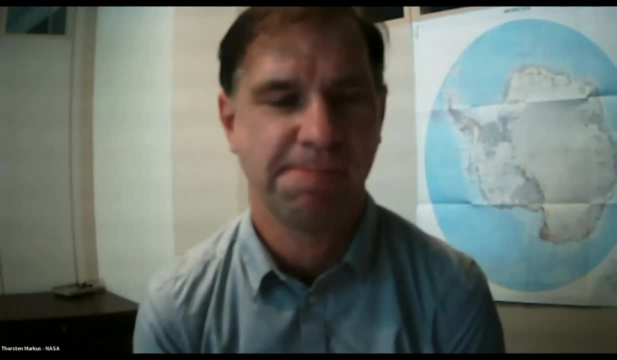 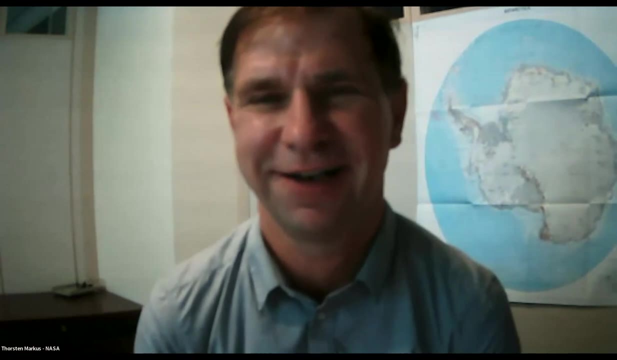 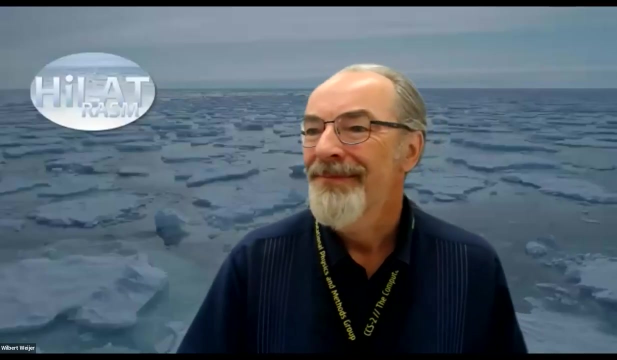 ocean chemistry. uh, effort, um, it's, it's, it's a good i. i don't know too much about it to have a good answer and i don't want to say the wrong thing. sorry about this, that's right, thank you, no, certainly so. uh, one thing i really know joseph. she was supposed to be here, but she couldn't make it. 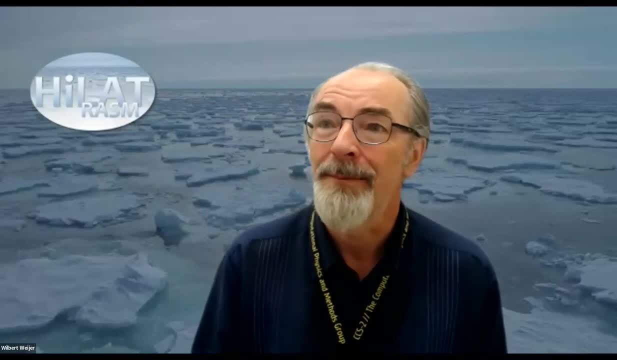 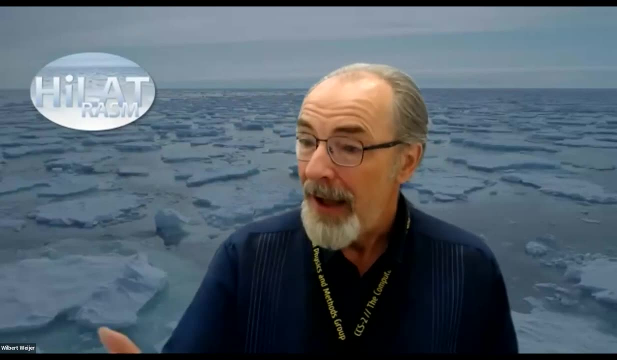 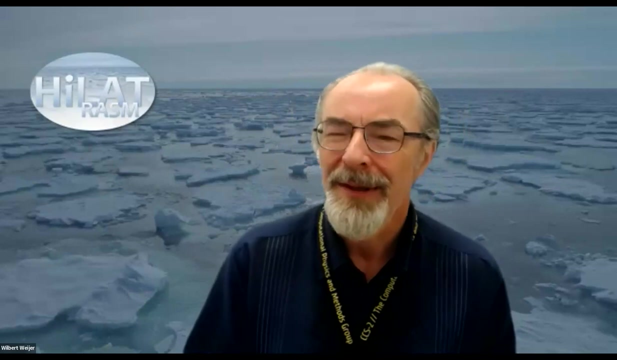 today, unfortunately. um. so she was supposed to represent um, the department of energy interest in the in arctic ocean oceanography. um, jackie, do you want to talk a little bit about kamas, which is an activity that is funded by the department of energy's office of science? 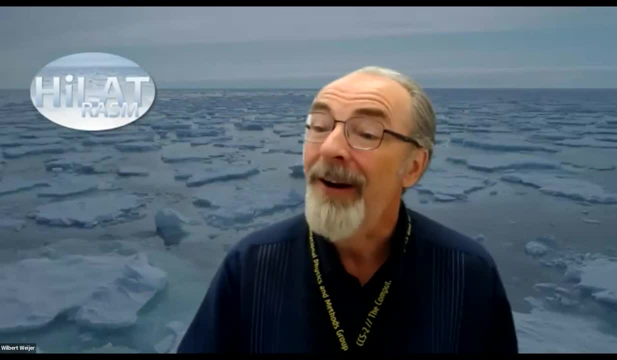 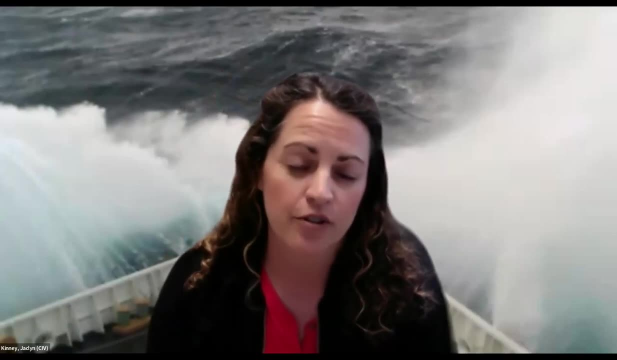 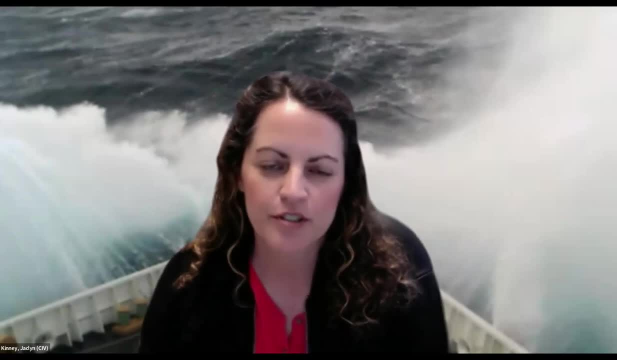 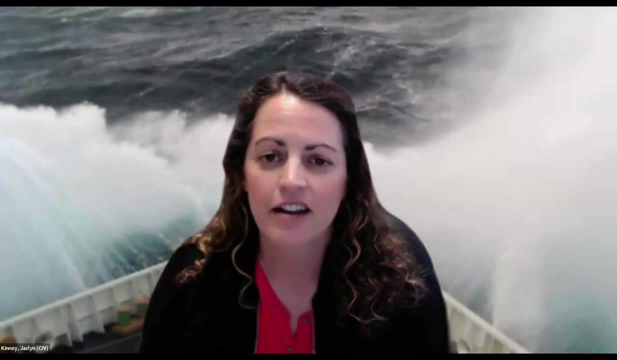 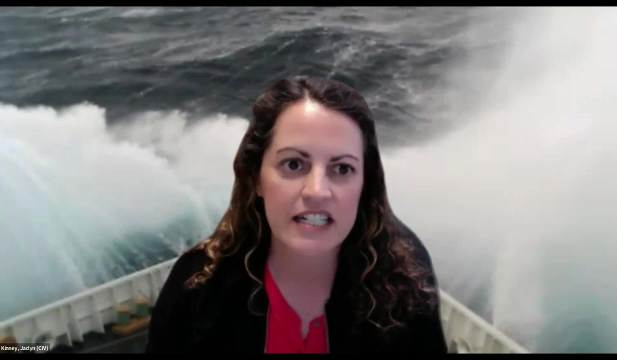 sort of modeled after the previous aoma and famous programs, if you remember those, and it's called kamas, the consortium for advancement of marine arctic science, and the first workshop is going to be in santa fe in february, on february 13th through 16th, and it's